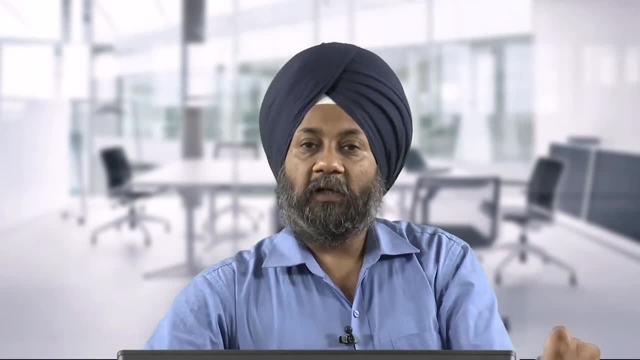 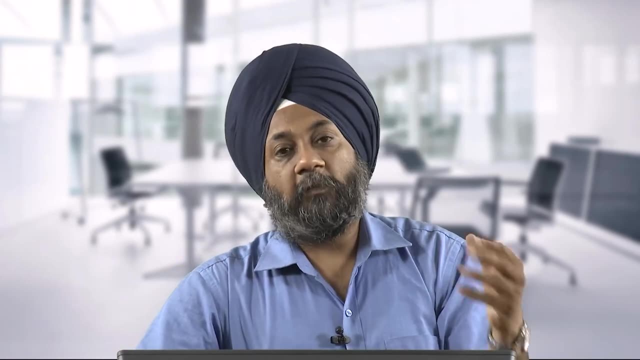 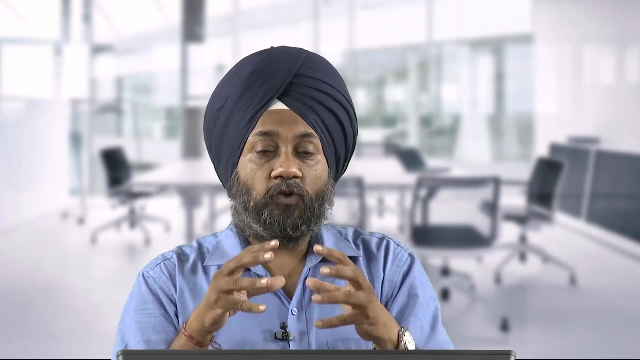 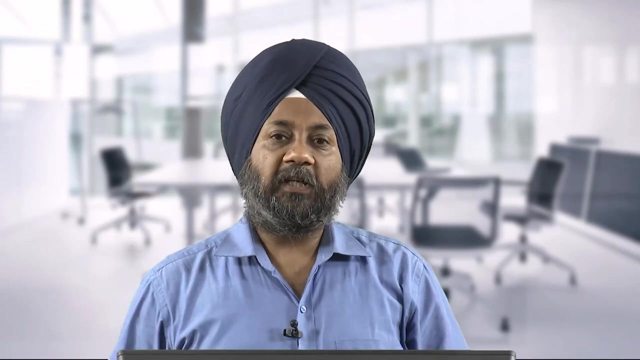 academic domain or the learning domain of a mechanical engineer or of a production engineer or of a design engineer or of a manager. So this course basically addresses the bridge, or tries to create a bridge, between a designer and the concepts of engineering. So basically, 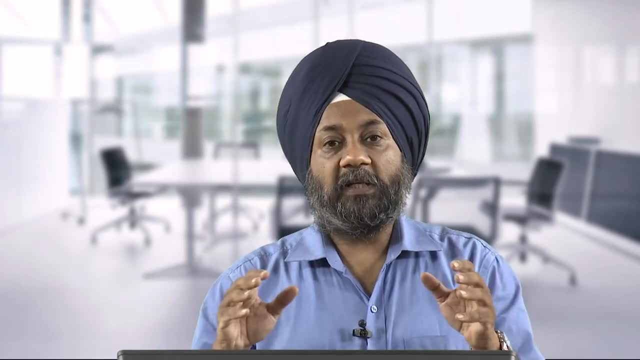 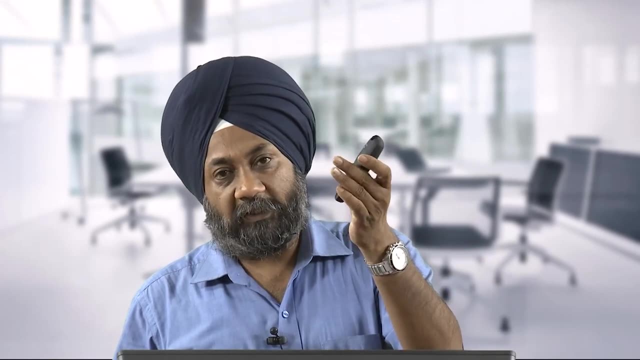 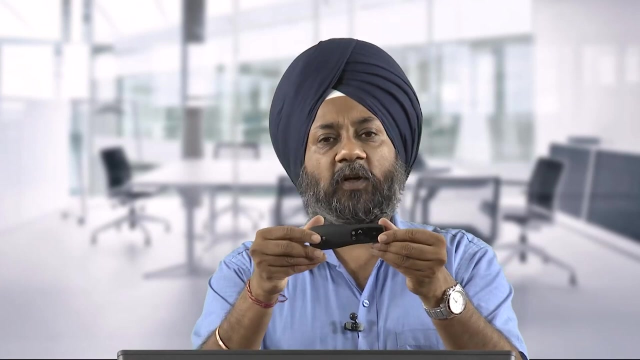 if you see around yourself or if you see around you, you will see so many products are there, For example. normally I take the example. this is one pointer. Come slide changer. it is a product. it has been made using standard manufacturing processes. 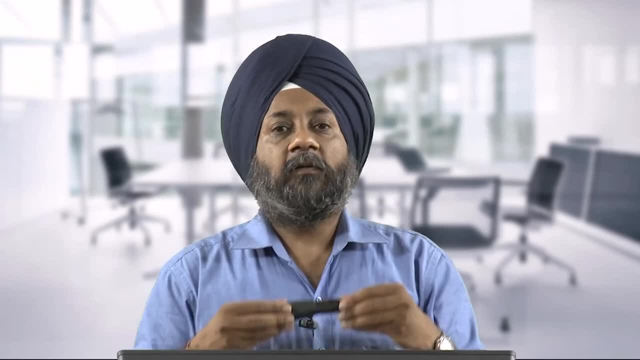 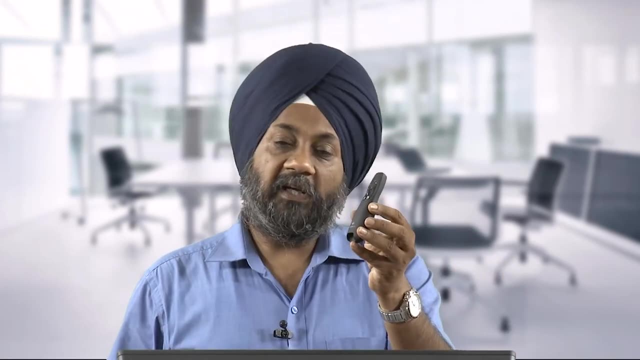 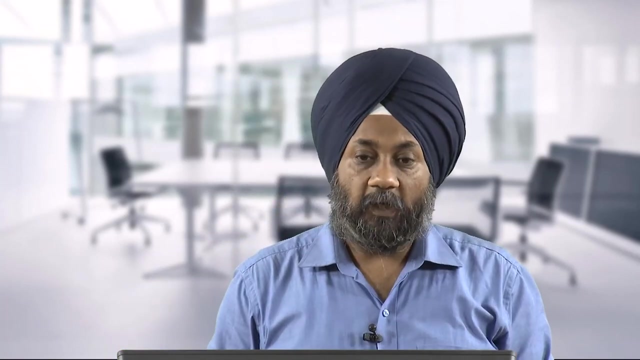 Now those manufacturing processes may be dedicated towards molding of plastics, because it is a plastic product. Similarly, if it has to be made in metal, we need to have understanding of the processes which can used for creating this type of a shape. So, a mechanical engineer, 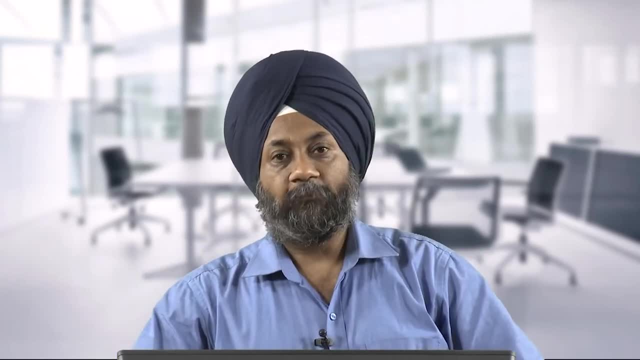 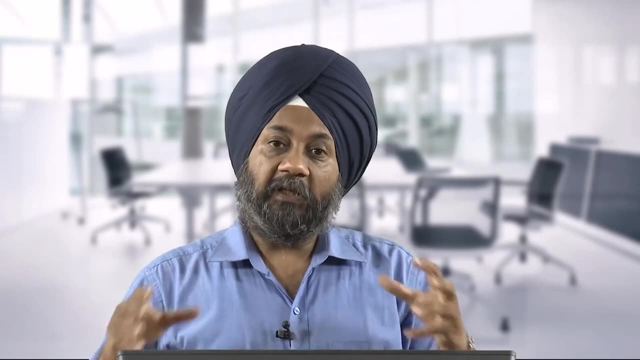 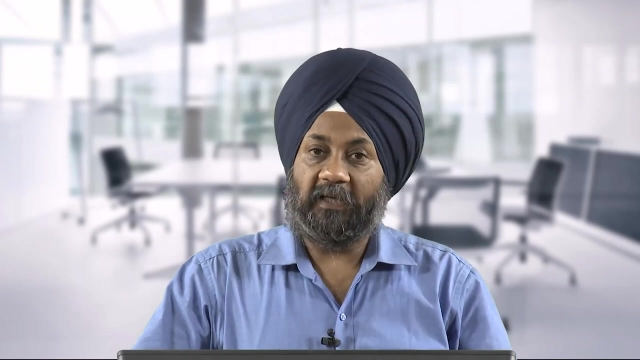 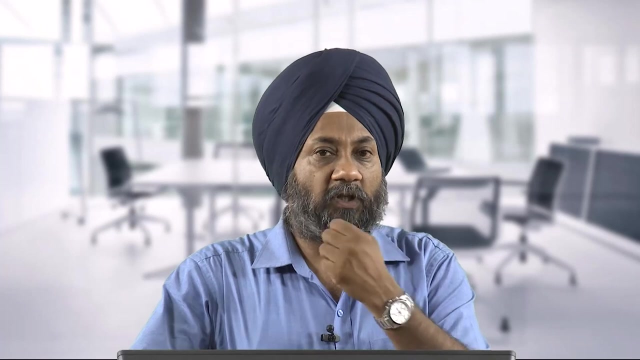 undergoes a curriculum In which he or she is taught regarding the basic concepts of manufacturing processes, Then they utilize this information, or they use this information during their service or during their professional career, But many a time whenever a designer is designing a product, he has no information regarding how this product will be manufactured. Similarly, 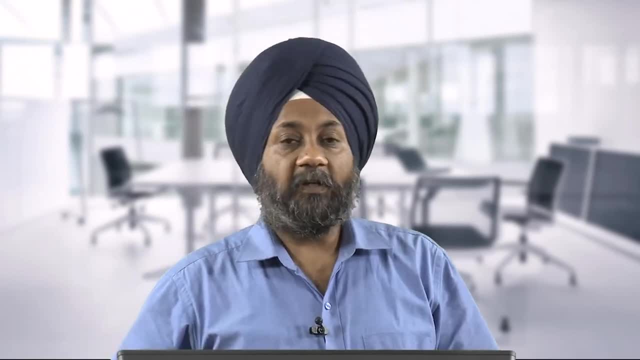 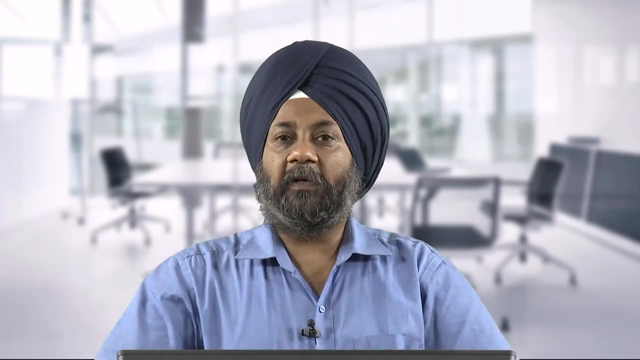 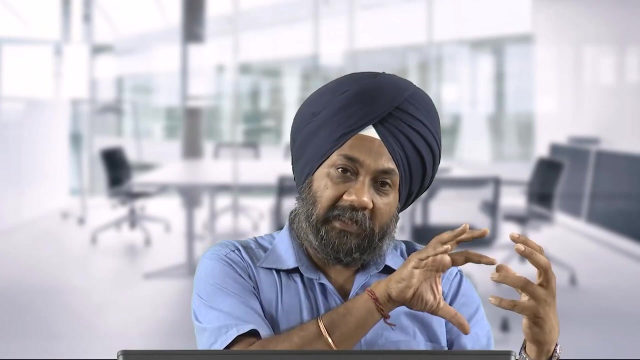 when a mechanical engineer looks at a Design, sometimes he feels that this could have been done in a better manner, or it could have been designed in a better manner so that it is easier to manufacture. So there is a gap between a mechanical engineers thought process related to the product design as well. 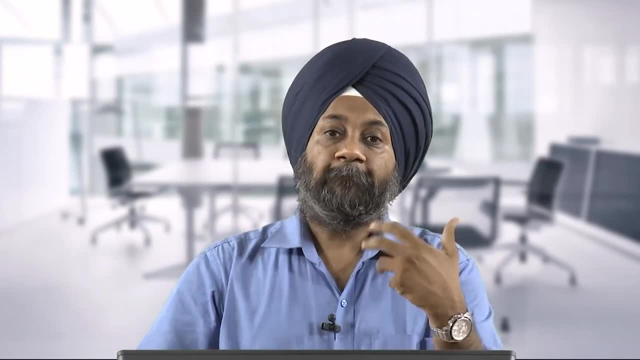 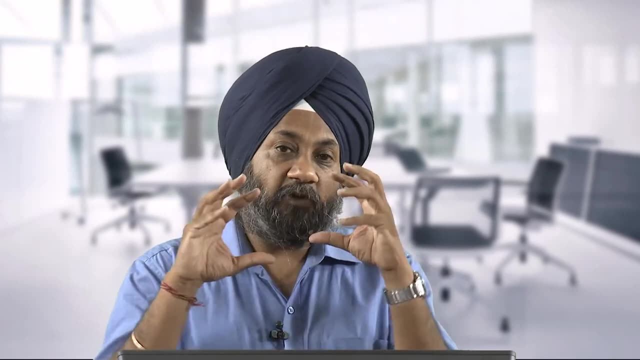 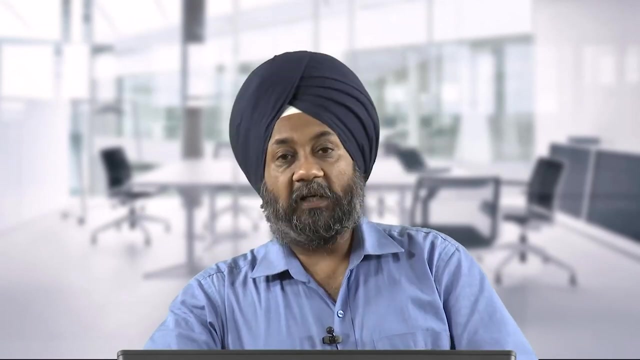 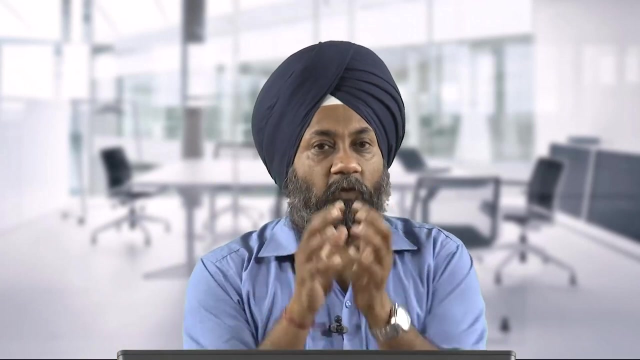 as a product designers thought process related to the manufacturing of the product. So we have tried to design this course in such a way We are able to understand that what are the guidelines that have to be kept in mind when we are designing a product. So, from mechanical engineers point of view, we will boil down. 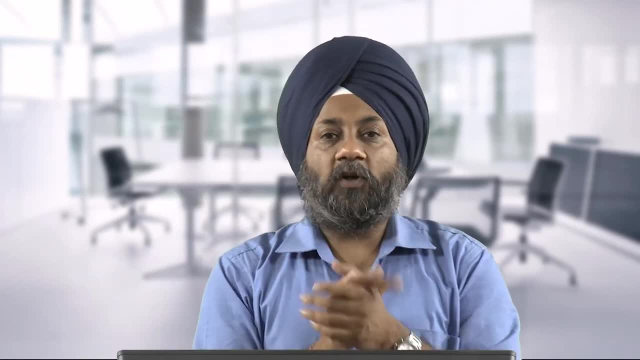 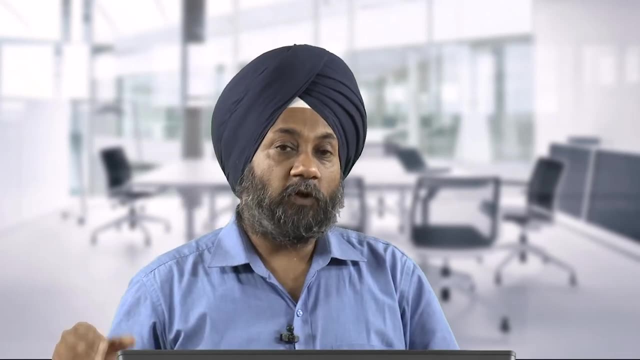 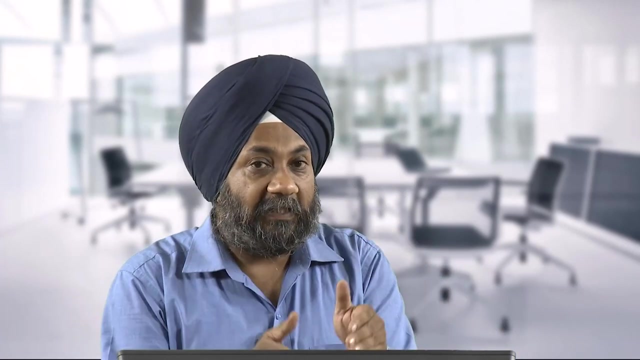 the information into standard guidelines which are already available and may not be taught in the UG or the PG curriculum, And from designers point of view, who has little or no knowledge about the manufacturing, We will try to frame certain guidelines. we will try to discuss certain guidelines which. 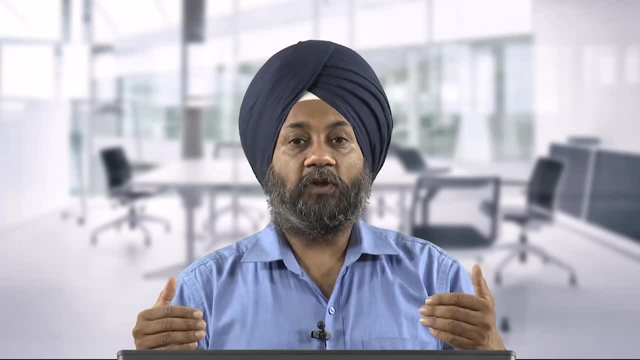 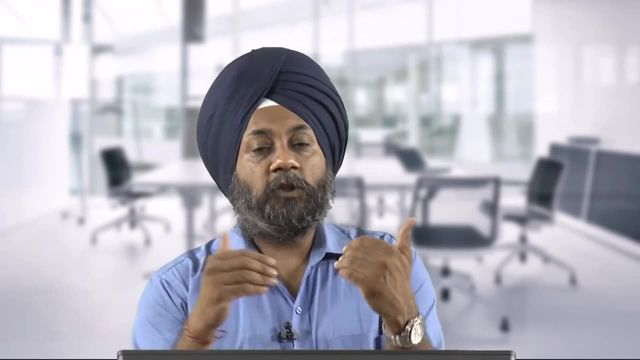 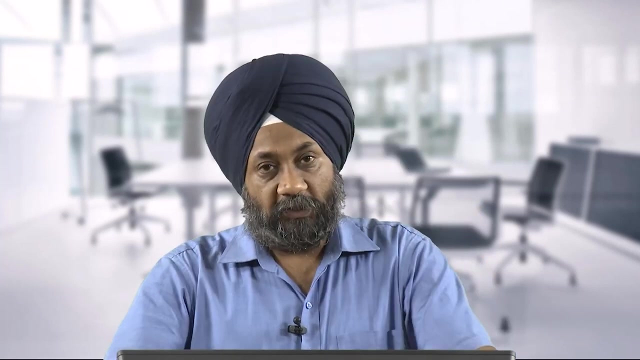 if followed, can help him or her to design the product in a better manner, or can take a informed decision that this product can be manufactured in the best possible manner using this particular process. So that is the bridge, or the gap that we want to fill. 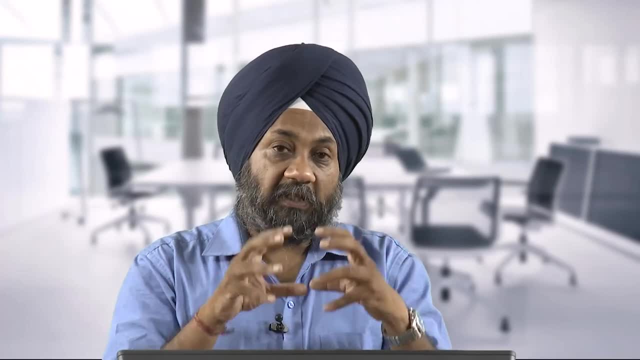 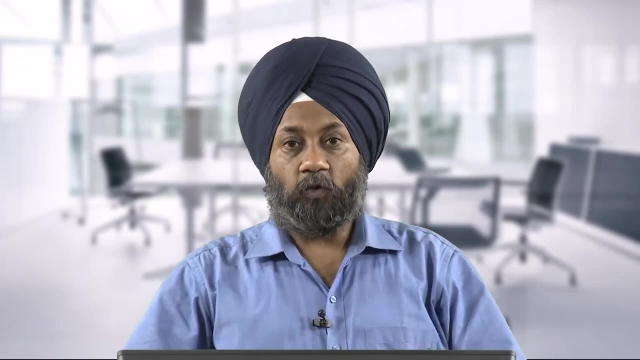 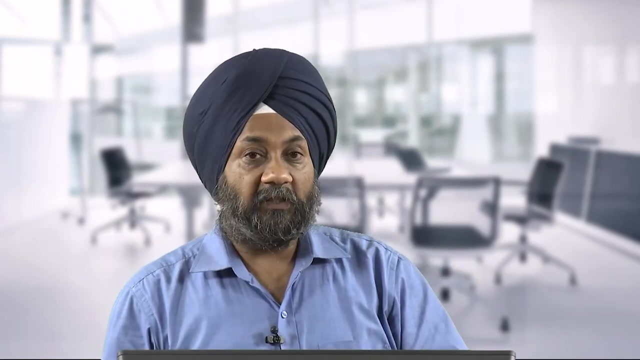 So the thing we want to develop, or we want to discuss, the guidelines for mechanical engineers. mechanical engineer may be knowing that what is a casting process, how to design the gating system for the casting, but sometimes, when the product has to be manufactured, that guidelines. 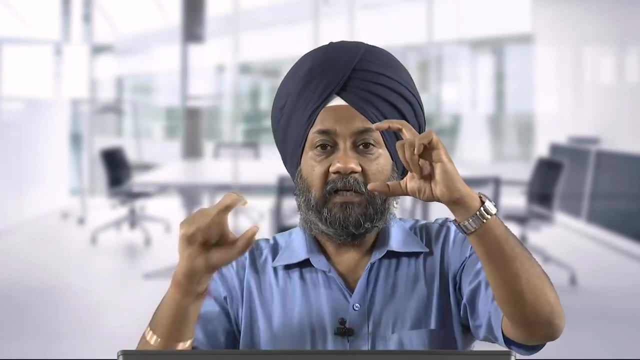 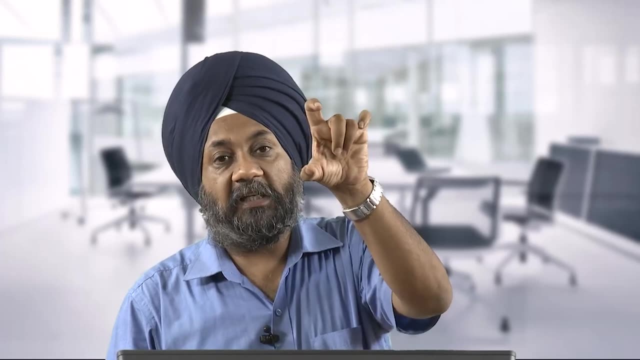 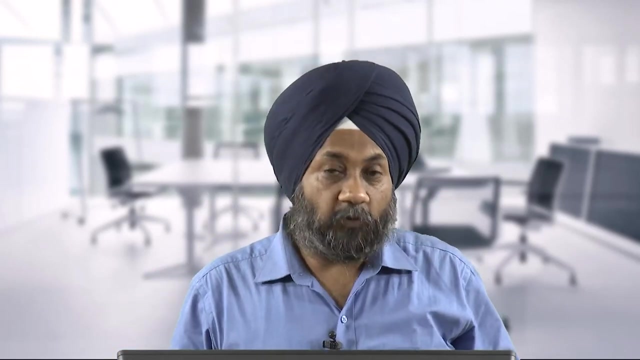 that this product, the watch, must be the change in the cross sectional area allowed. if the product is long, Maybe we have to see that the cross sectional area at one section is higher, other fraction it is too low. in that case, what type of problems may come? 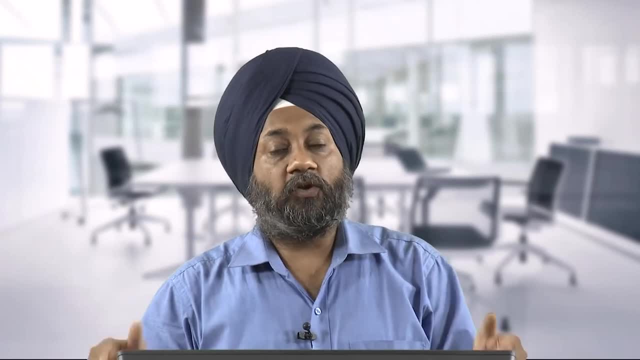 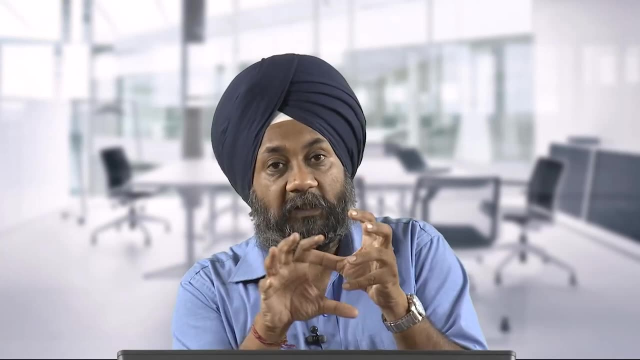 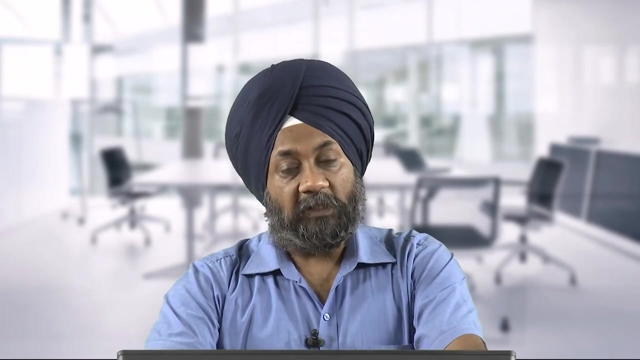 So there may be certain guidelines established based on the research, based on the experience which can help a mechanical engineer to figure out that if the product has to be made by casting, what are the things to be taken care of? Normally in our curriculum we see that we are taught regarding the processes, regarding 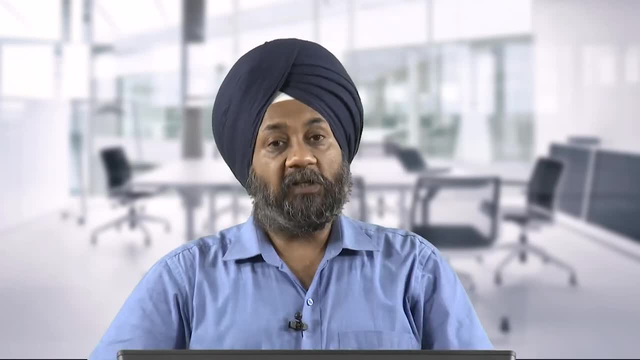 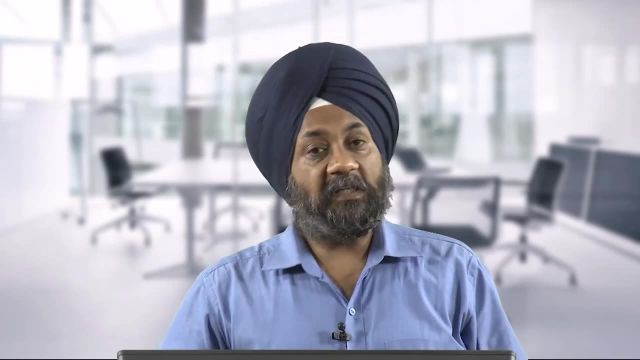 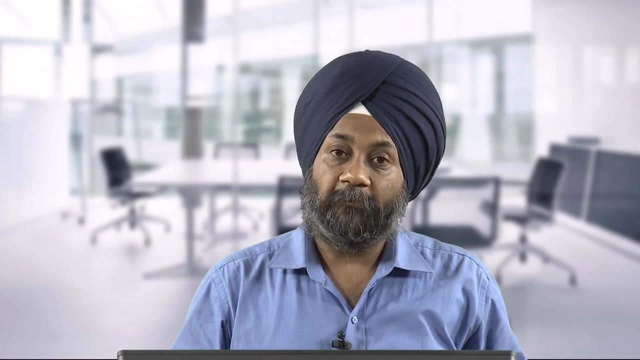 the application regarding the limitations, but we usually lack the design guidelines that are established for the various processes. Very seldom our students know that if casting has to be made, a product has to be made by casting process. what are the various design guidelines to be kept in mind for the design? 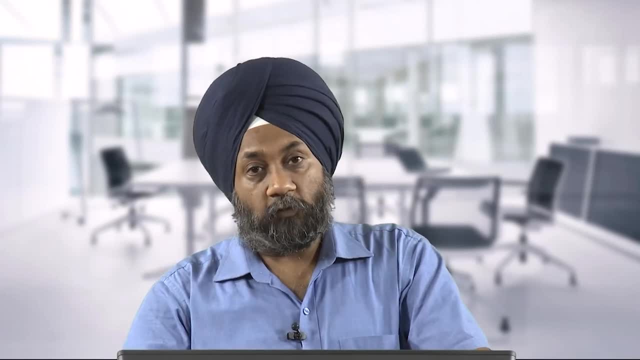 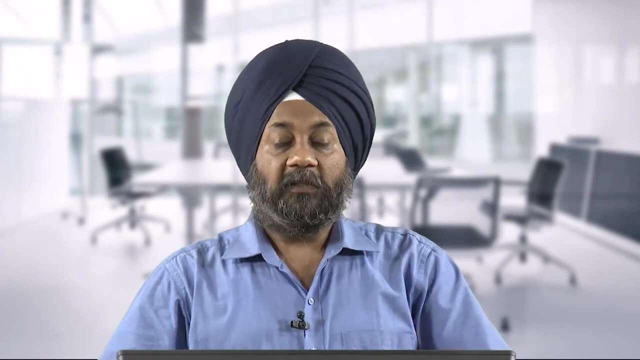 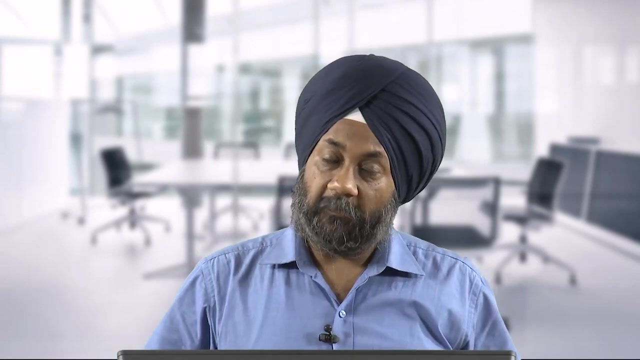 point of view or from the product design point of view. So that is the basic thing that we need to understand. Another thing I would like to mention here is that we are not going to study the manufacturing processes in this course. and if you refer to MOOCs- the massive open online courses which 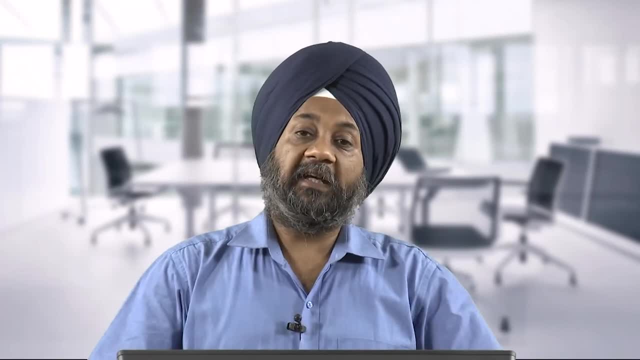 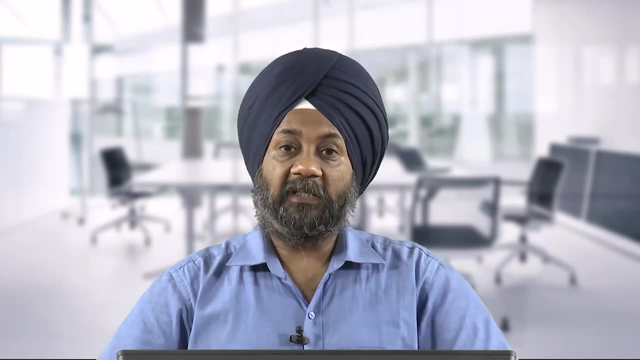 are available. There are number of good courses where lectures have been delivered by the experts of manufacturing, engineering or processes, who have recorded the lectures and have been run successfully. These courses have been run successfully. Our target is to understand the manufacturing processes, So that is the basic thing that we need to understand here. 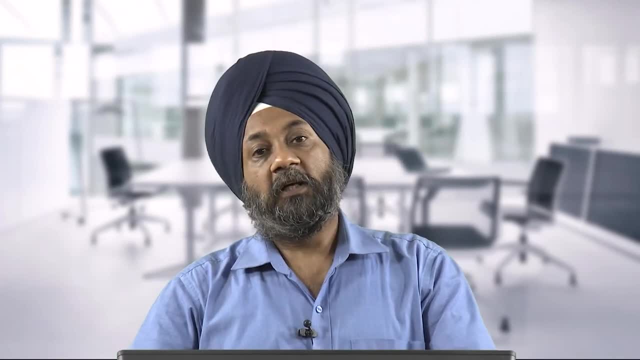 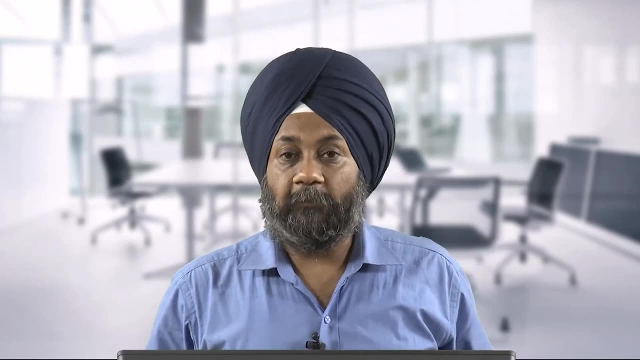 We need to understand the guidelines, which can be helpful for a product designer. So if you want to design a product, what are the various guidelines that have to be kept in mind? So we can say that this course is slightly on the applied side, that we will be just taking. 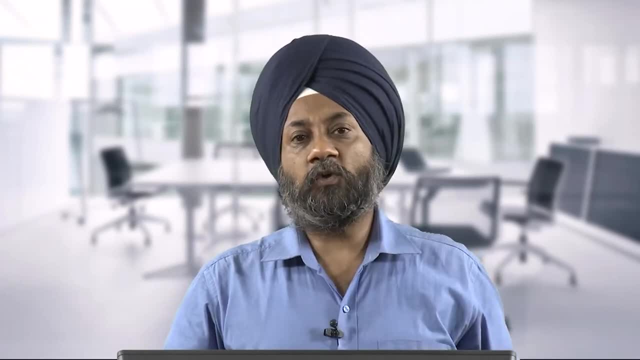 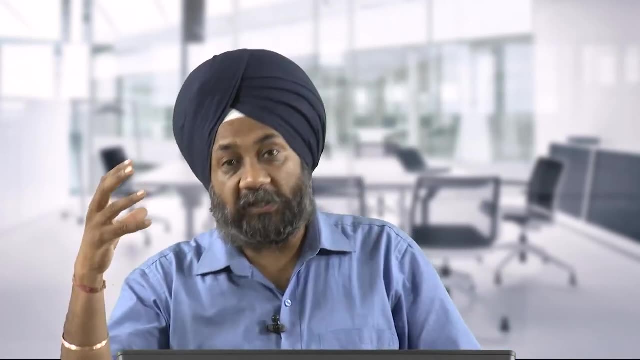 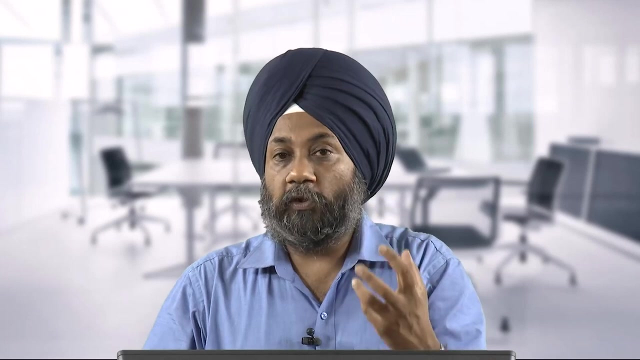 casting as a process. maybe 15 to 20 minutes of discussion on the casting process, But the more focus will be on the guidelines that once you are designing a product- what things related to casting- you must keep in mind So that you are able to produce a good product. 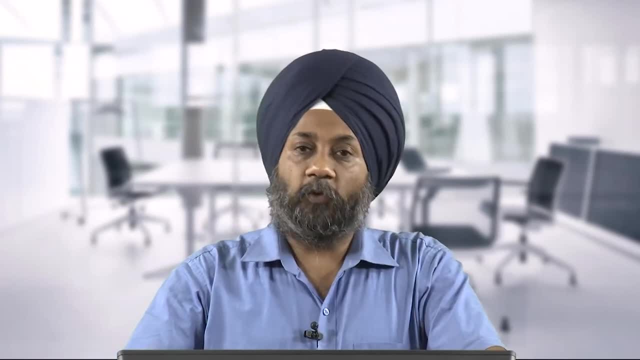 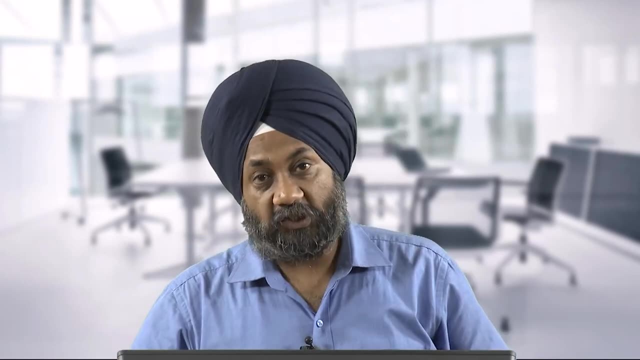 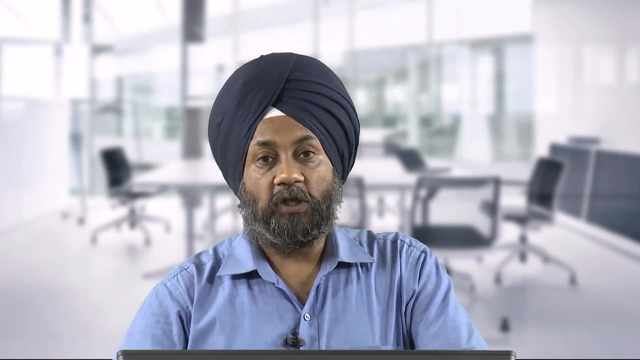 So casting. I have taken an example because it is a well known process in manufacturing engineering. We will discuss regarding the manufacturing guidelines for the plastic products also, like one example I have already taken or we will take different examples: the mouse or the cabinet of a computer system. 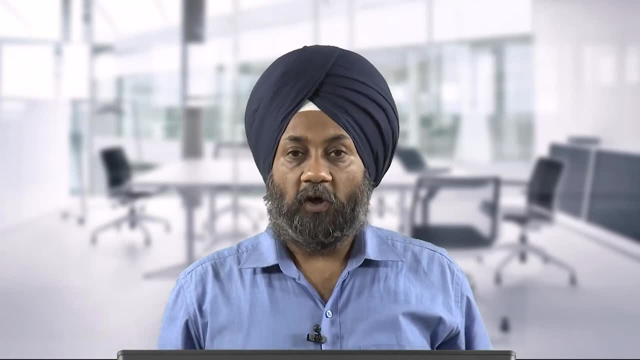 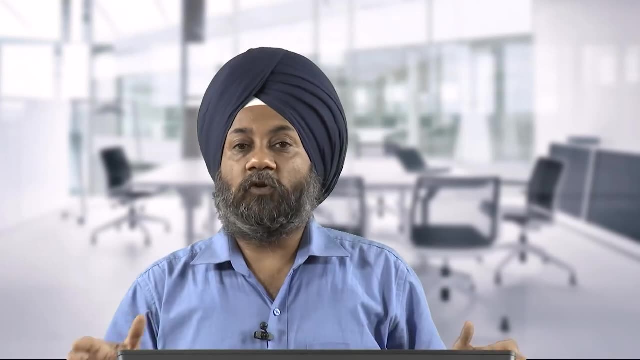 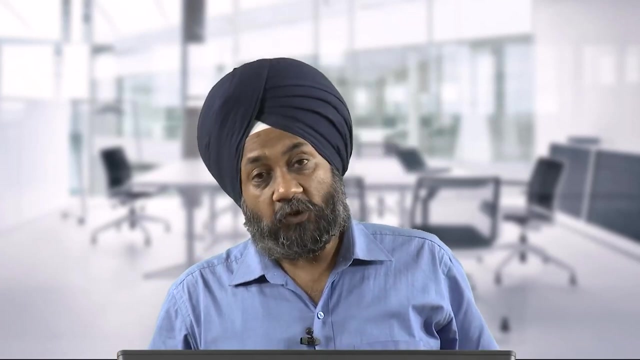 So Different types of products that we use all around us. we may be using a simple key chain or we may be using a pen. we use different types of product. handle of the brush: the bristles that are fixed on the handle of the brush for brushing our teeth. 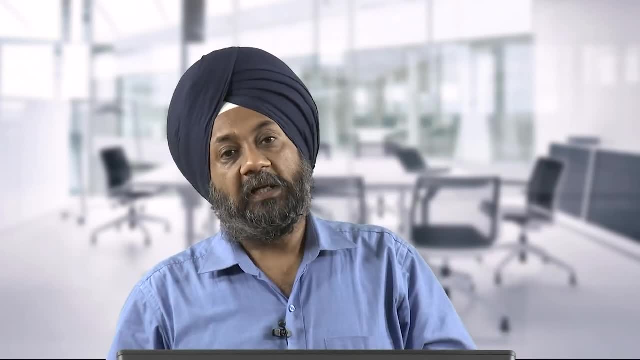 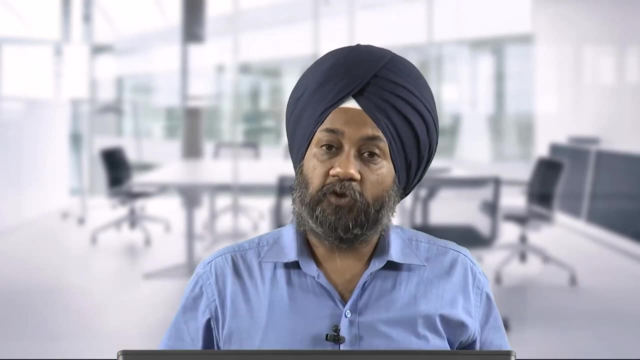 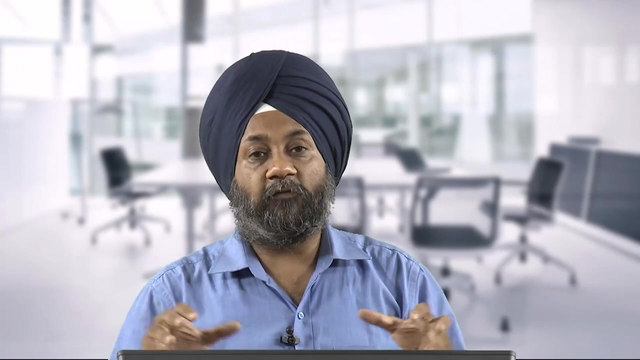 So, right from the from waking up in the morning till we go to bed, we use different types of products which are manufactured using different types of processes. it may not be possible for us So, within these 20 hours of discussion, to cover each and every manufacturing process. 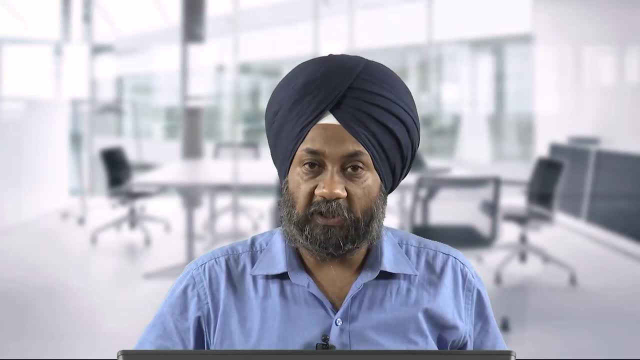 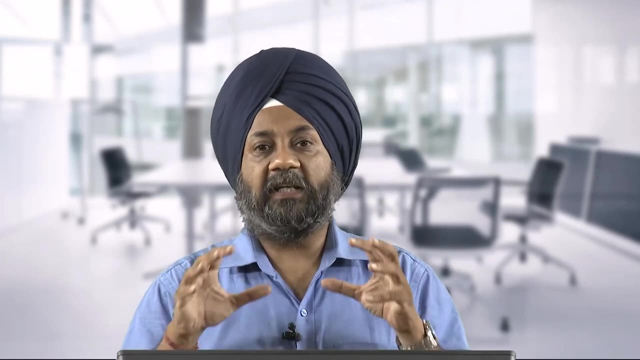 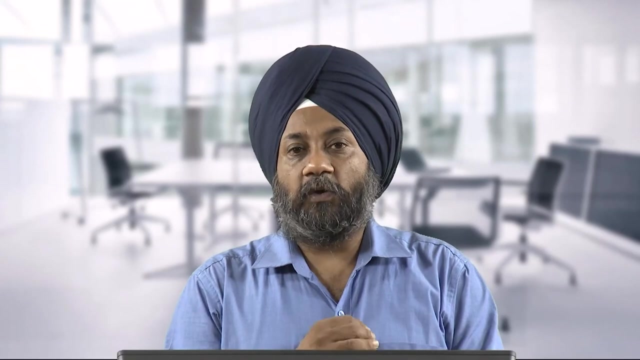 that is used for processing of or fabrication of products, But we will try to limit our discussion to the most important and most widely used processes that are used for manufacturing of products. So we start the discussion today by classifying the manufacturing process or by introducing 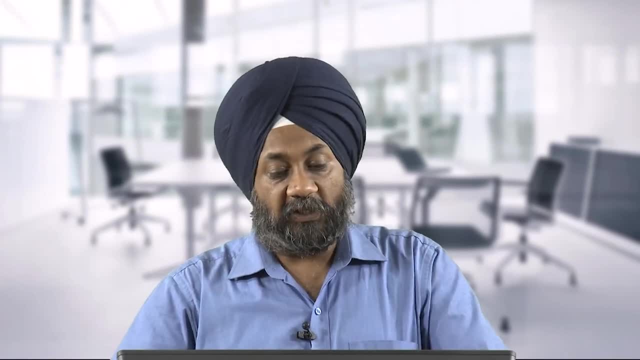 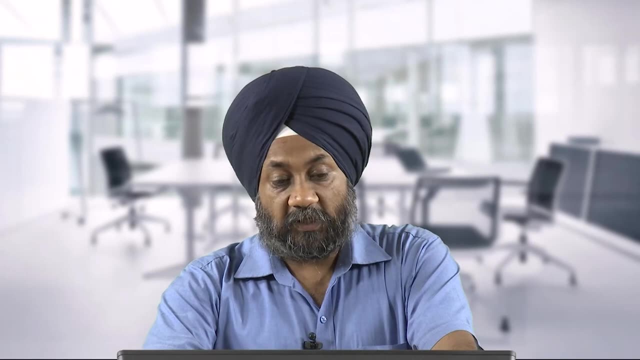 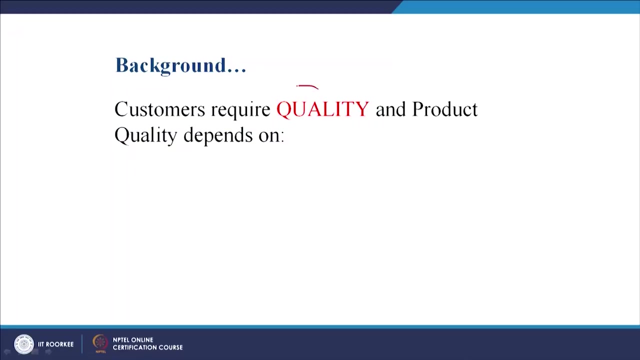 the concept of manufacturing process. What is the title for today's introduction of manufacturing processes? So let us see the importance of the manufacturing processes Now. these days, each and every customer looks for quality, So quality is the key word these days. and how quality is defined, that we can see. 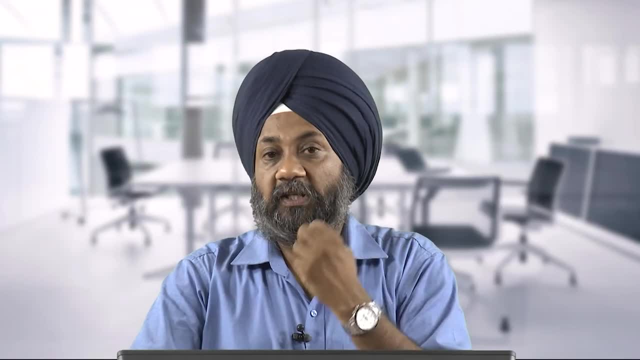 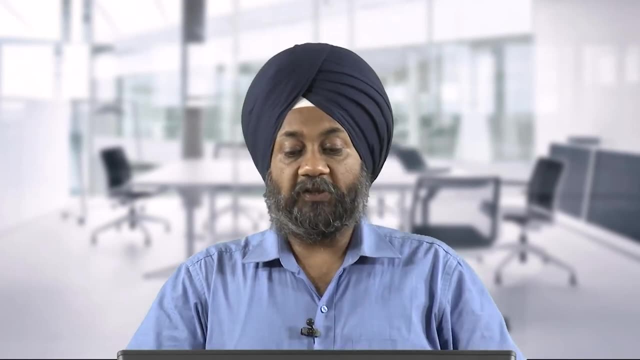 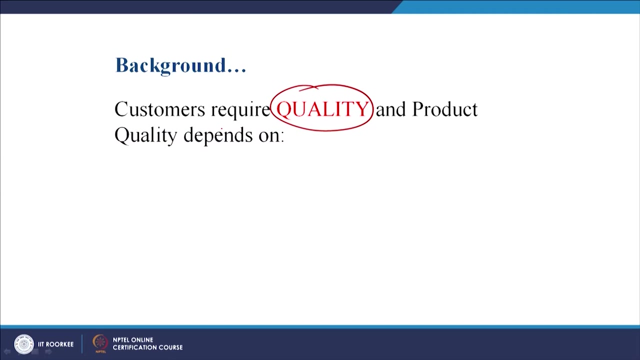 We can see that what are the important characteristics that have to be controlled in order to deliver the quality for our customers. So So the customers require quality and the product quality depends upon- I can give you just 10 seconds to decide that- what can be these parameters? 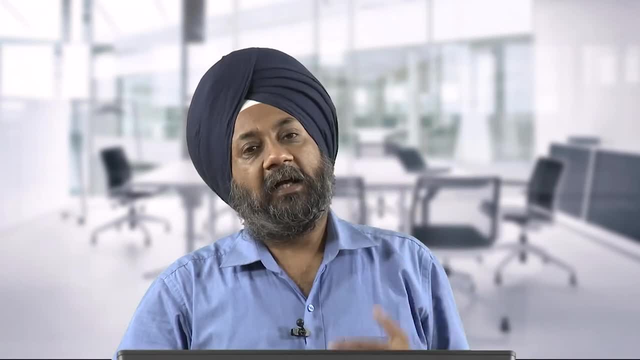 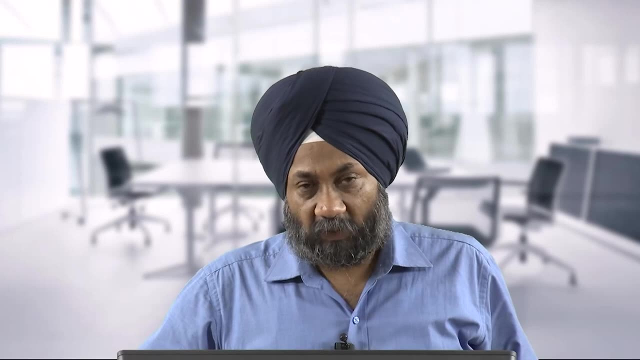 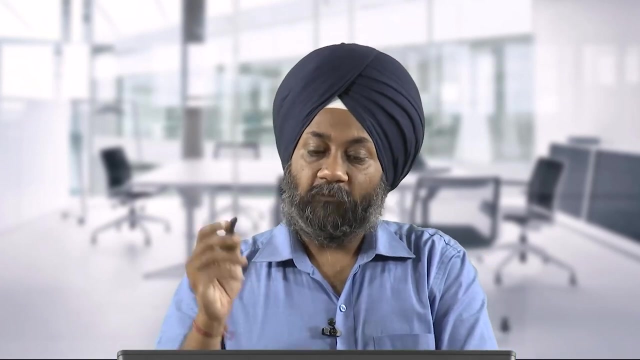 Number of answers will come. all of you will have different answers. some of the answers can be: if the product performs its intended function, it is of good quality. Then, how to ensure that the product performs its intended function? for example, I have used this pen. I have used it to mark quality. 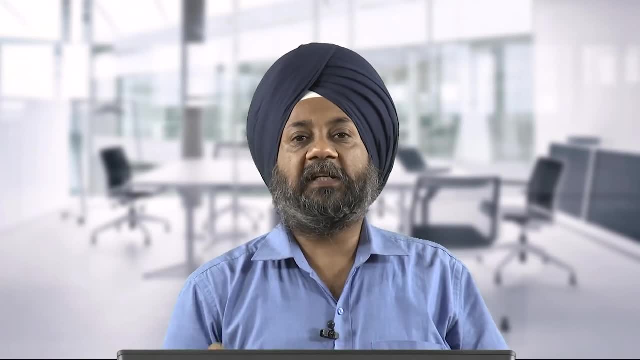 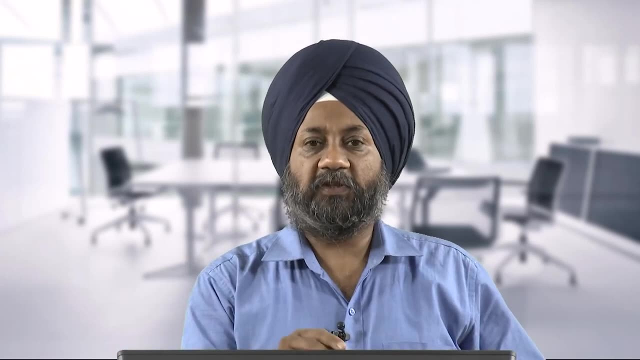 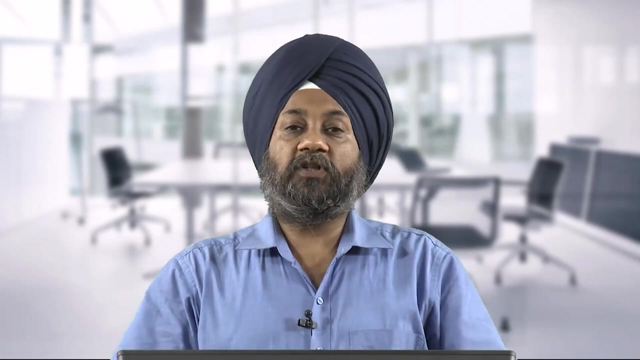 Now suppose I start using it and it is not working properly. I will say over this is having a very poor quality. I was trying to use it and I was not able to draw a circle around quality, So poor quality. so we say quality is a certain when that intended function is achieved by 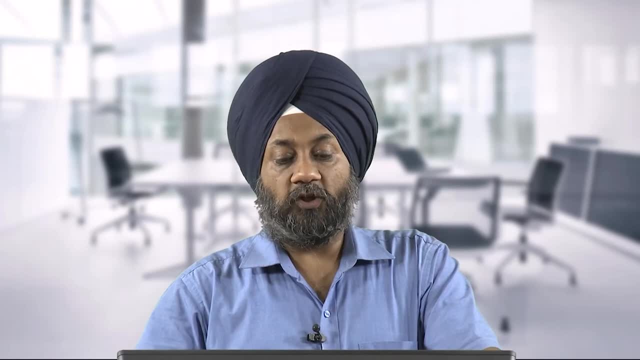 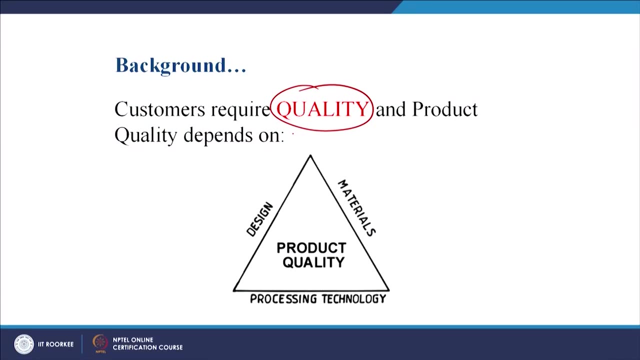 the product, But how to ensure that we can ensure that using 3 important we can say aspects or the characteristics. So the first one that is very, very important is the product design. So product design is very, very important and if you remember, some of you may be familiar- 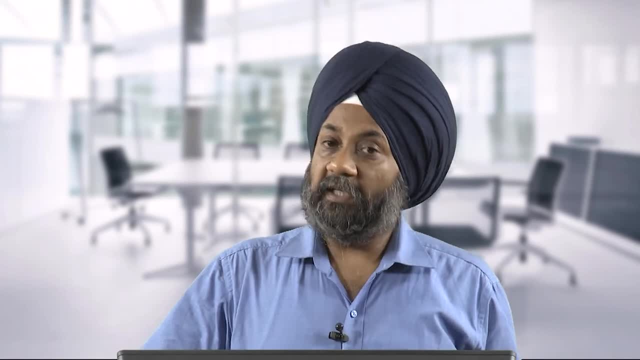 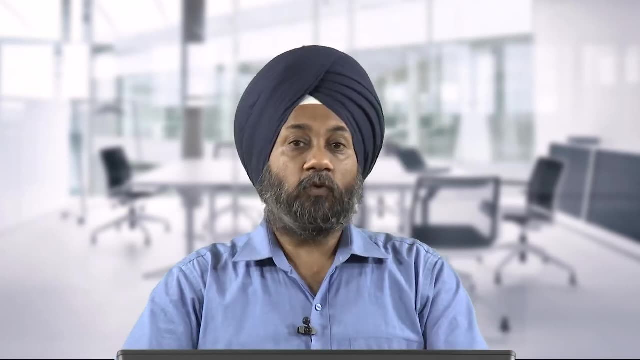 with the lectures that we have covered till today, We already have run successfully 2 times a 10 hour course on product design and development. So we will not go into the importance of product design, but certainly it is an important parameter and important characteristic. 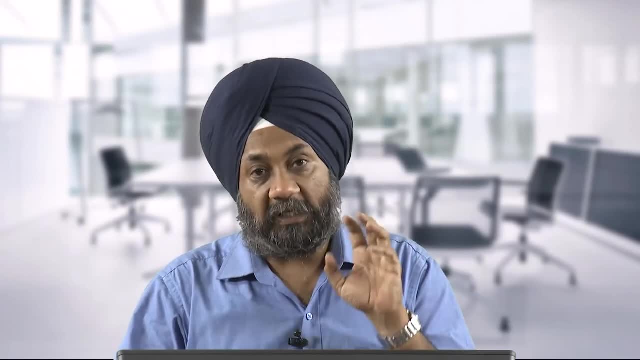 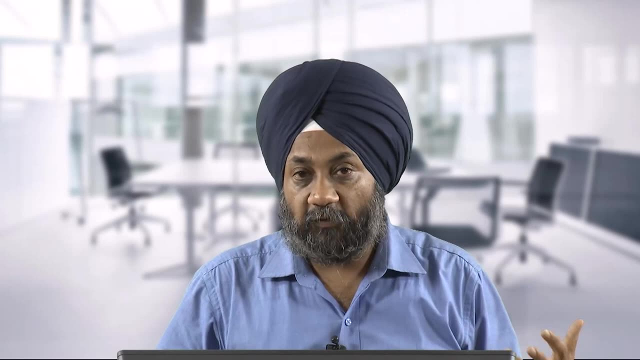 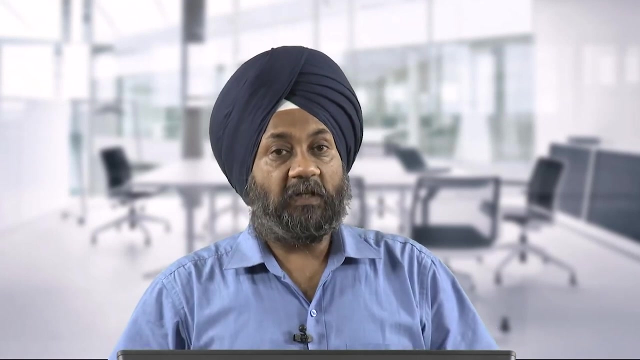 And important aspect And important aspect, aspect, an important criteria which defines the quality. So if the design of the product is good, the quality will definitely be better. So we have to ensure that the product design must be excellent. Now, how we can ensure that the product design is excellent? we have to have this understanding. 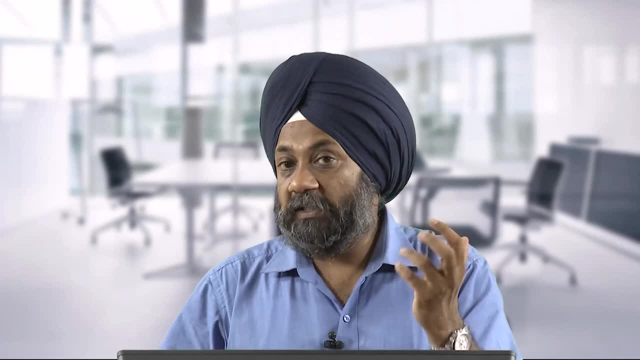 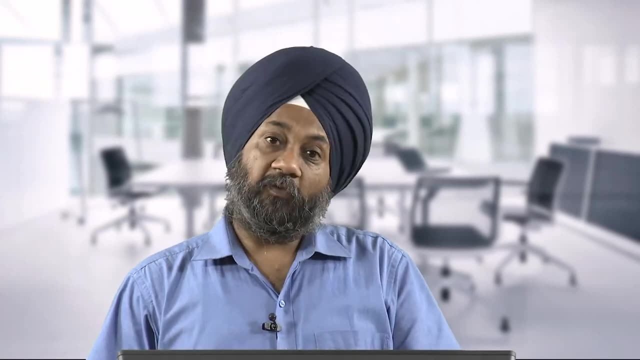 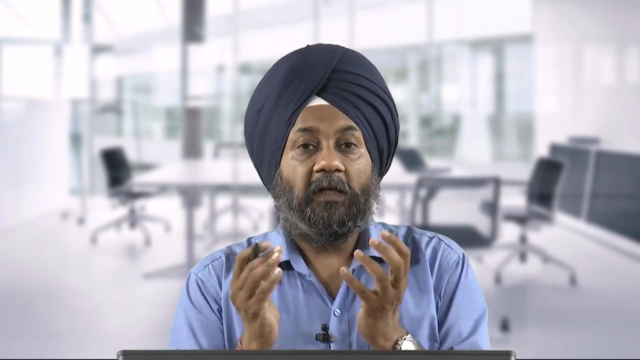 of the guidelines through which we are going to convert our idea into the product. So the first and foremost important thing is the product design. So design has to be successful. and how it will be successful if we have all the information related to the product design process. 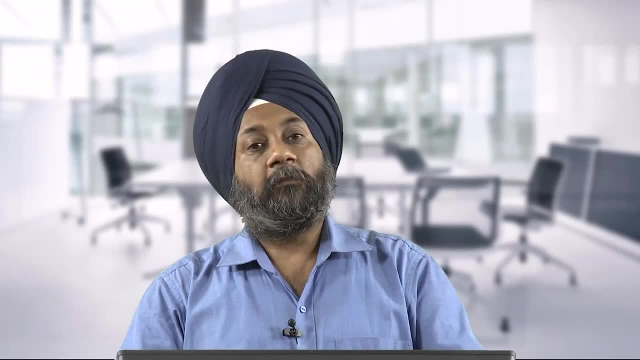 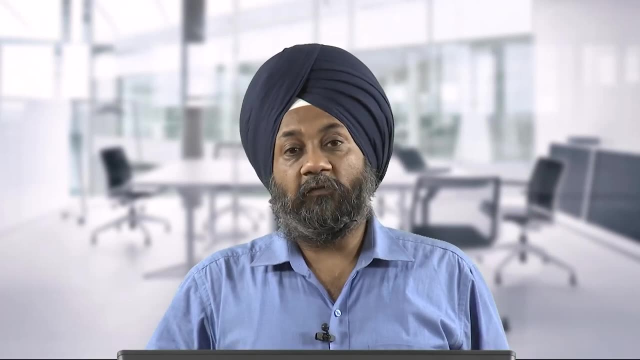 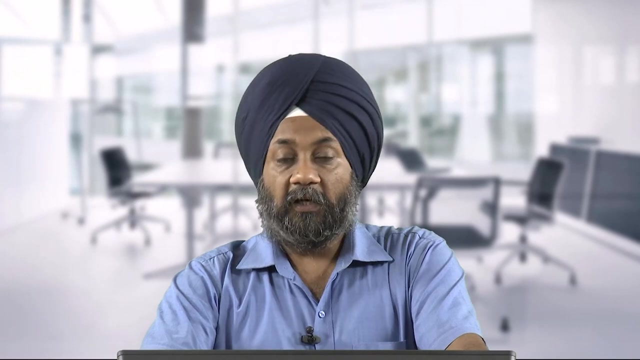 In the end when we do a prototyping of a product beyond that, the product goes for commercialization and actual manufacturing or fabrication. During that time we have to keep in mind that: how the product is going to be manufactured. So during the design stage only our focus must be that: how the product is going to be. 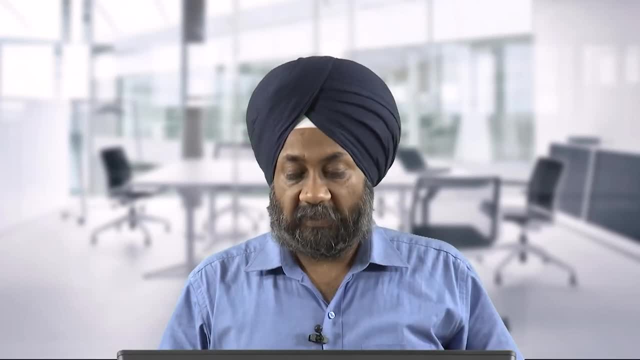 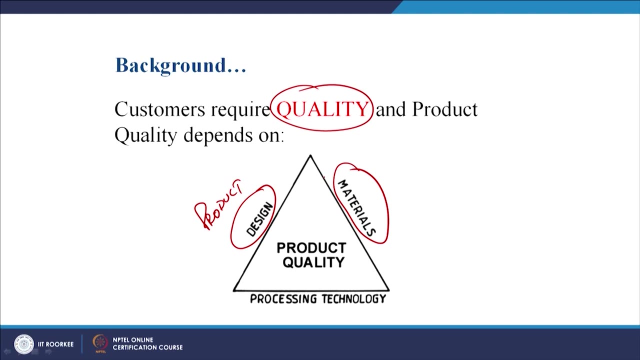 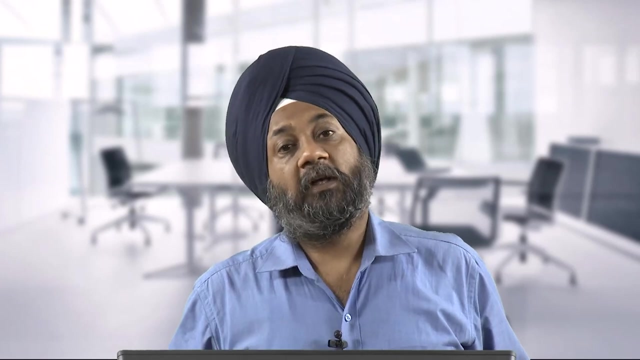 manufactured. So the first important part is the design. The second is the materials that are going to be used, So that, as we have already told, this is a product made out of plastic, then there can be products made out of metals, products made out of wood, and each and every material will. 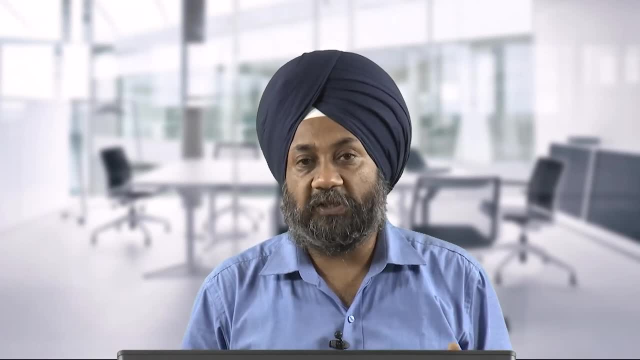 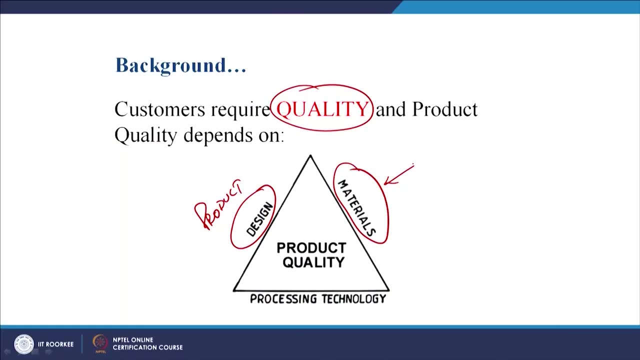 have dedicated specific manufacturing, Specific manufacturing processes. those will be used for processing the materials. So therefore, from materials point of view also, we must have the understanding of the manufacturing guidelines. why? because the manufacturing guidelines may vary for wood. Manufacturing guidelines may vary for metals. 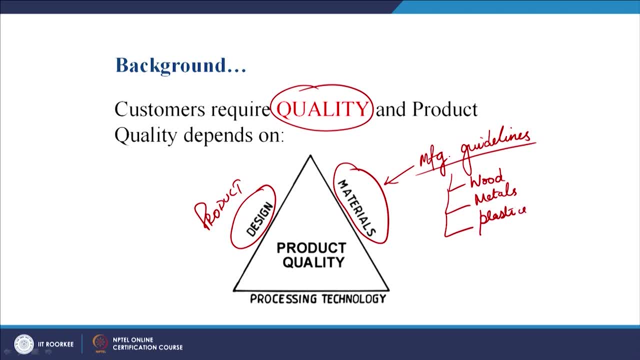 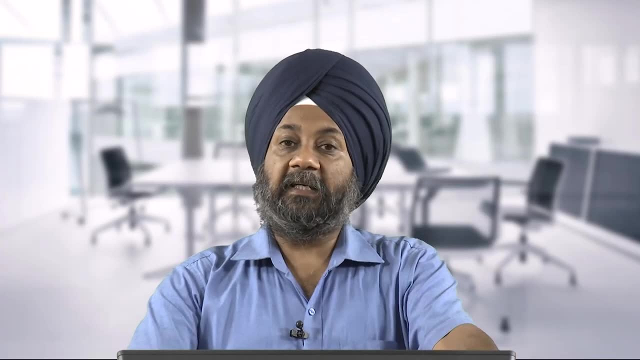 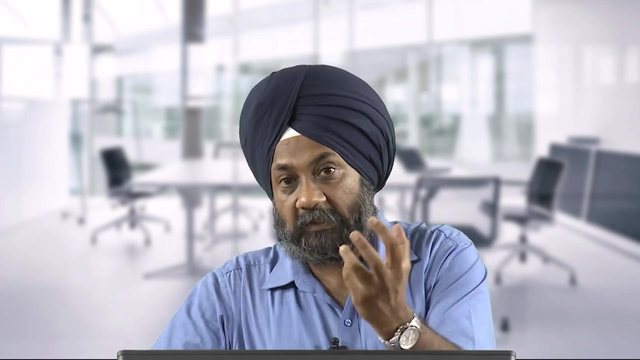 Manufacturing guidelines may vary for plastics. Manufacturing guidelines may vary for composites. Manufacturing guidelines may vary for ceramics. So you can see that if the material is changing, the manufacturing guidelines also change. So we must have idea about the guidelines So that we are able to design the product in such a way that we use a specific material. 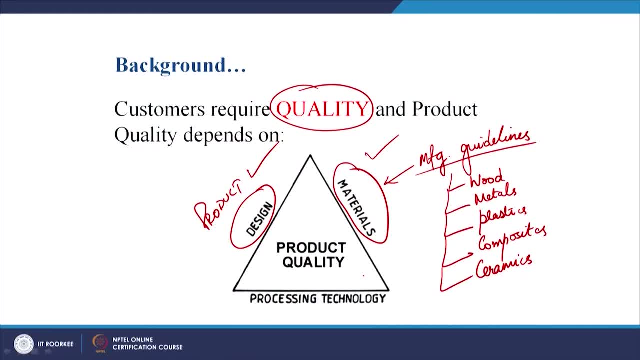 for making the product. And finally, we must have information about the processing technology. And here our offshoot or the summary of this is what is our target in this course. We need to understand the summary of the processing technology. For example, if the product, we have already designed the product. 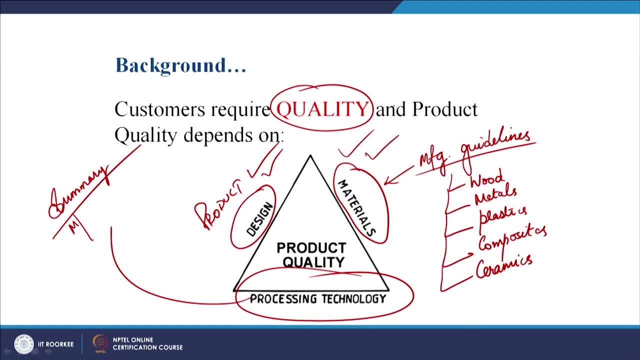 We have selected the material, which is a metallic part or the product has to be made by using a metal as the material. Now we have to do the machining of that part or the product. Now, what are the guidelines for machining? There may be specific guidelines that may be required when we are designing something. 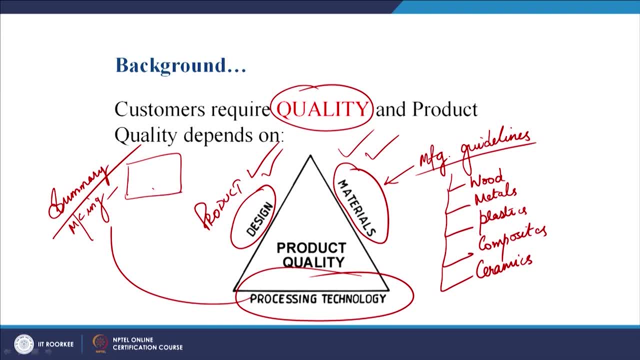 One example we can take. suppose this is the part we have to have a hole here. So when the hole is required at the edge there must be some guideline that how much portion of the hole has to be machined Basically inside the main body of the part. so this can be some guideline. 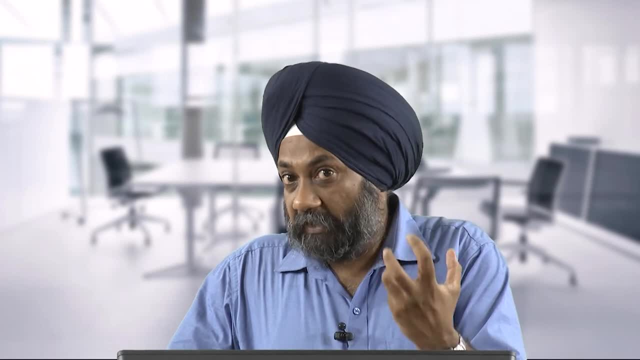 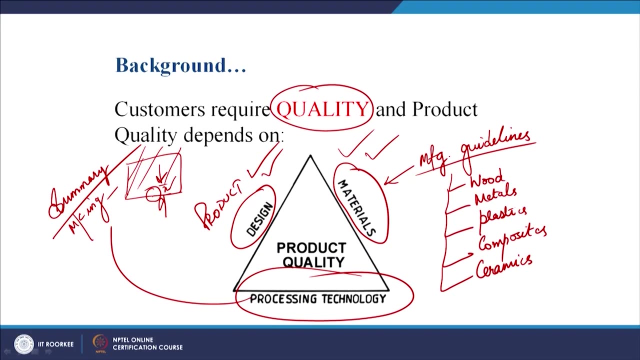 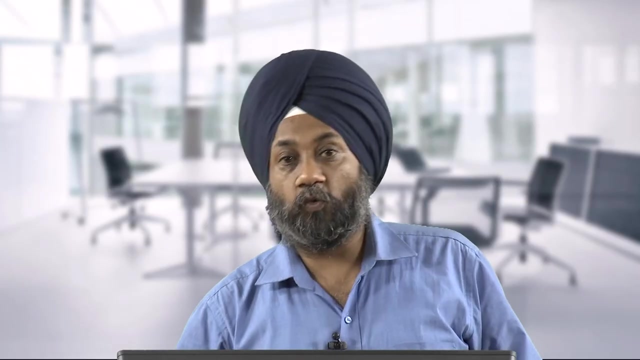 So if that guideline we know, we will take that guideline into the design process. When we are designing our product we will keep this guideline in mind that what portion of the hole must be there in the body of the part, And that guideline will help us to avoid any poor design. 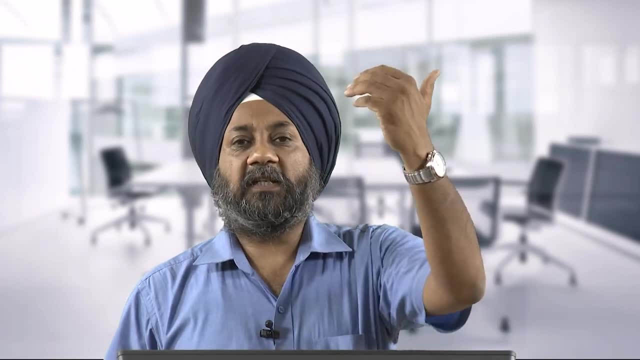 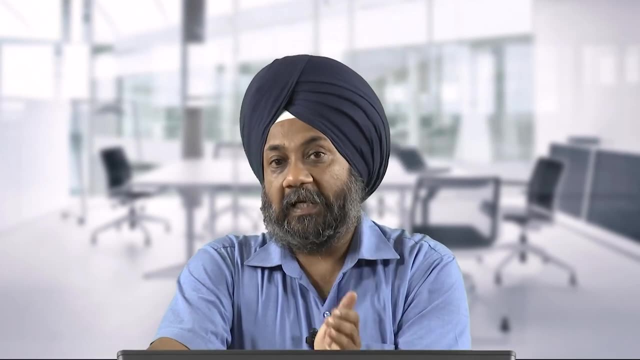 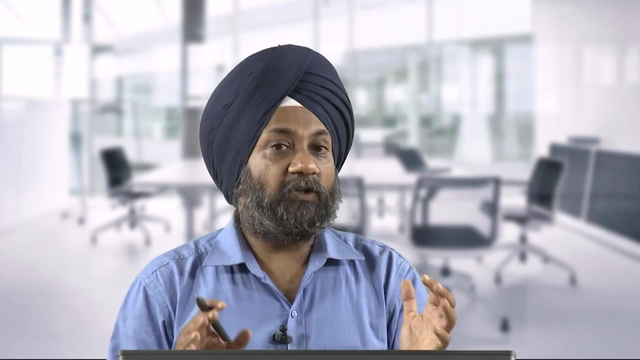 This is one example I have taken. there are number of such examples Which can be taken into account and which will be discussed with the help of examples, diagrams, videos, whatever possible in the lectures we will try to cover So that, once you are complete with the course, you are able to focus on your design by keeping 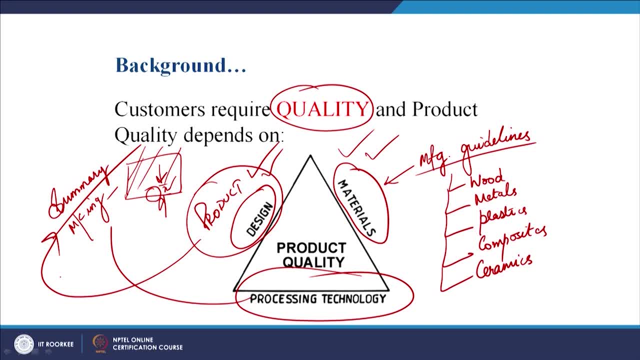 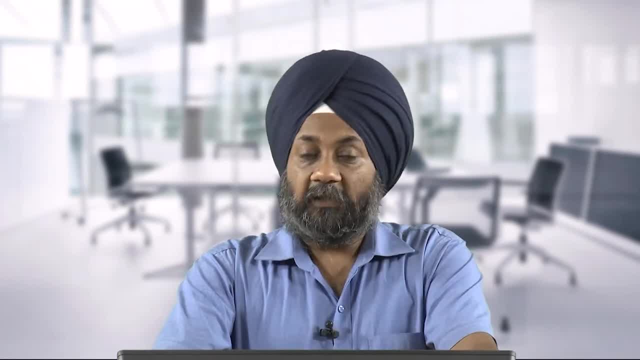 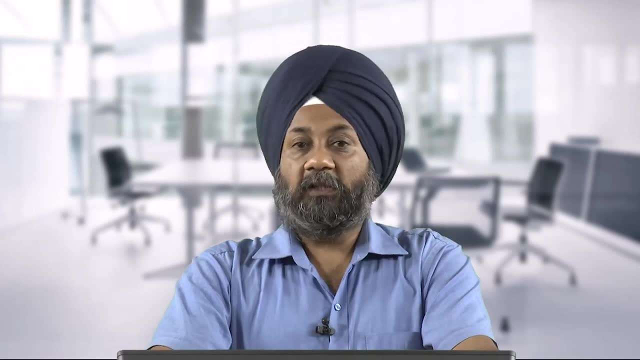 these guidelines in into your thought process or keeping these guidelines as a reference tool while you are designing a product. Once you decide the product has to be made Made in a plastic material and it has to be made by injection molding process, You must follow the product design guidelines which have been established for the injection. 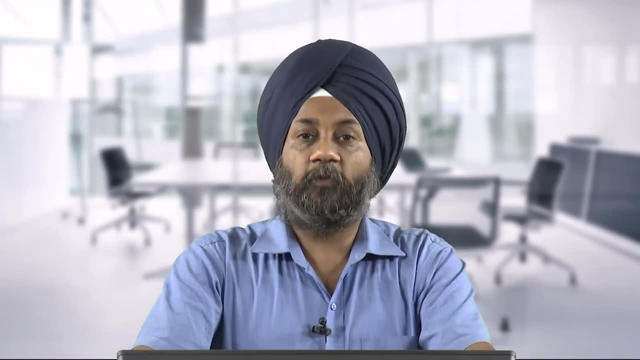 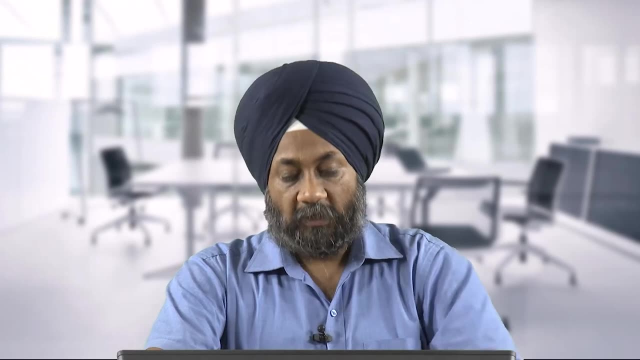 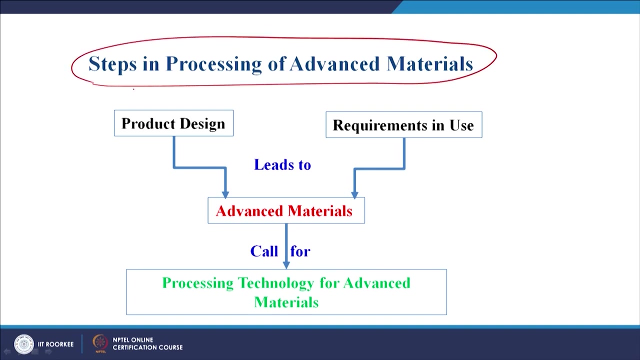 molding process, So that you produce a good quality product which is acceptable to the customer. So that is the summary of what we are going to cover in the next, maybe probably 19 hours of our discussion. Now, what are the steps that have to be followed for advanced material? 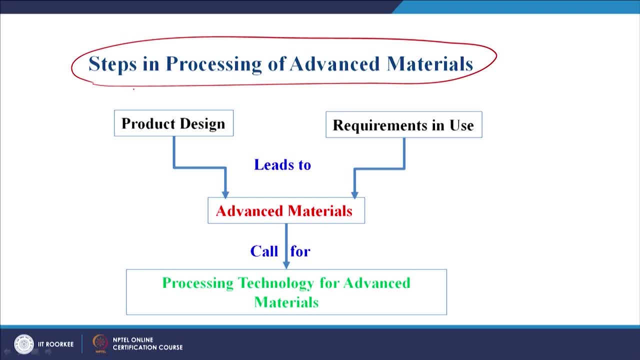 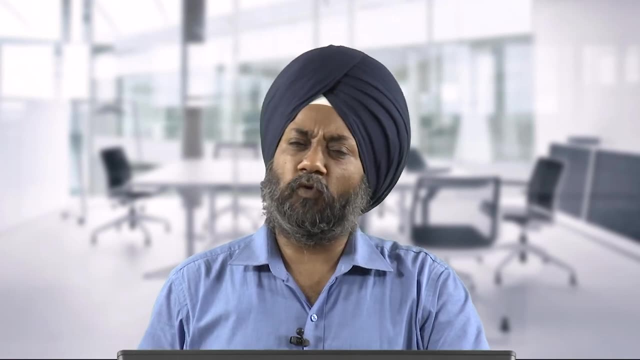 Now We have to decide on developing our product in a new material, in advanced material. So first thing that has to be taken into account is the product design. You can see that product design is very, very, very, very important aspect In today's scenario, when there is lot of focus on innovation. there is lot of focus. 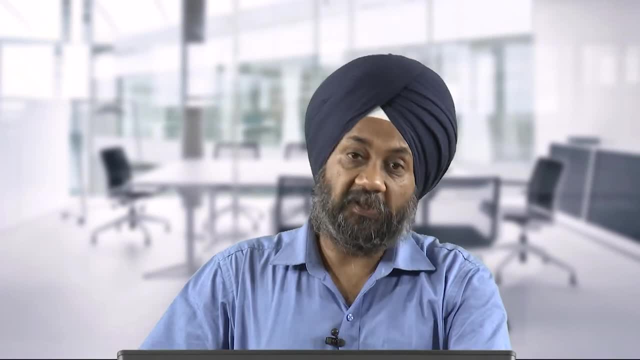 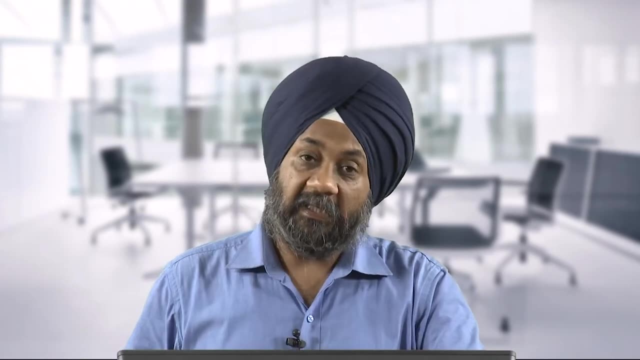 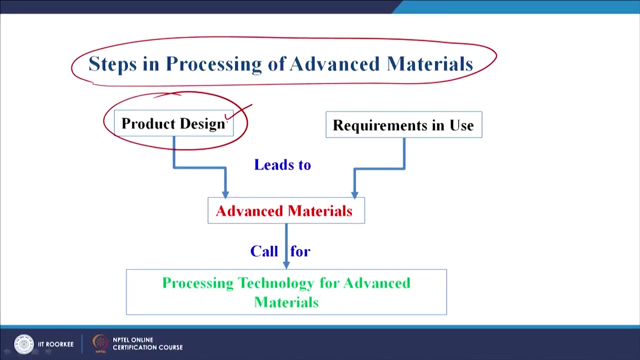 on entrepreneurship. there is lot of focus on starting businesses, So there the product design becomes very, very important. So if you have a good product design, We can Very easily run a successful business. and then we have to see that when we are talking of advanced materials or new materials, we have to adjust our product design accordingly. 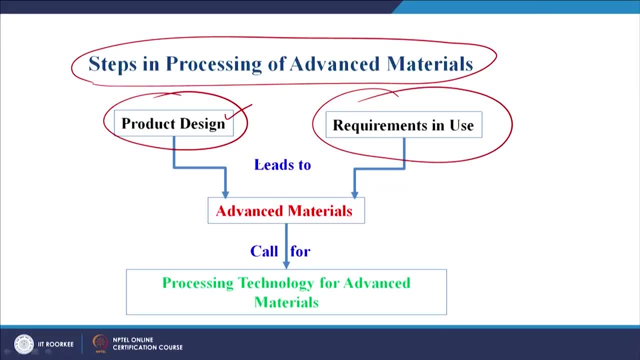 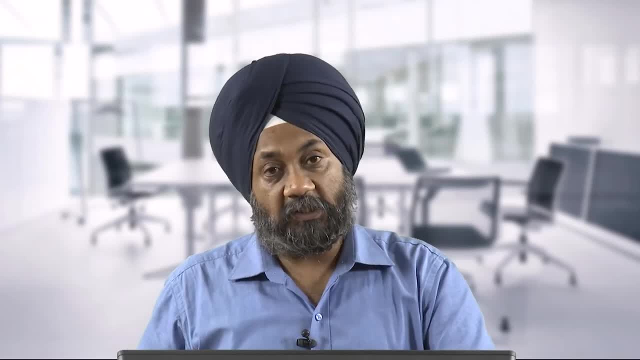 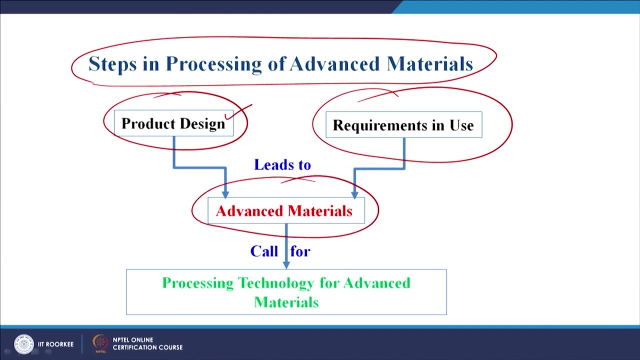 Similarly, we have to understand what are the requirements in use, That when we are going to use the product, how or what type of environment, what type of conditions it is going to encounter, And that leads to the development of advanced materials. So the once we know that advanced materials have been developed, we must have the information. 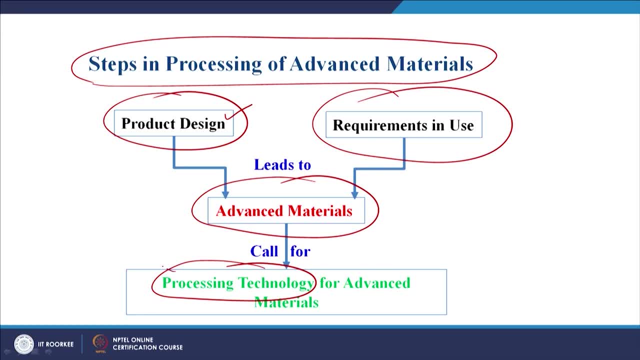 about the processing technology- and here also our course is going to address that once. for advanced materials or new type of materials. what are the guidelines So we have? these are the materials. maybe one category of these materials can be composite materials. What are the processing guidelines for these materials? because whatever are the traditional 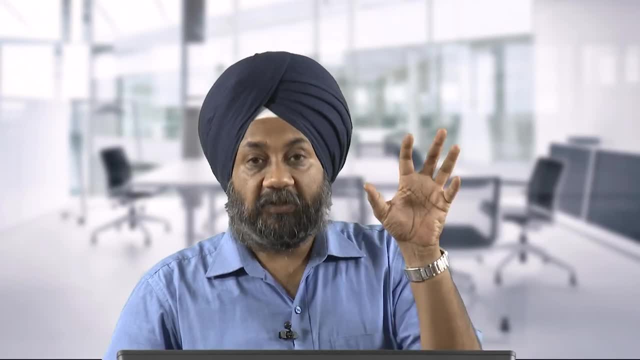 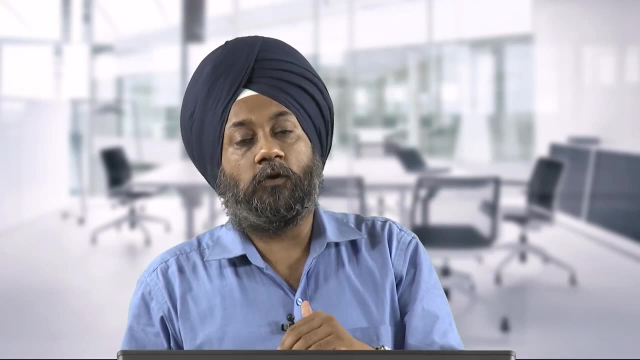 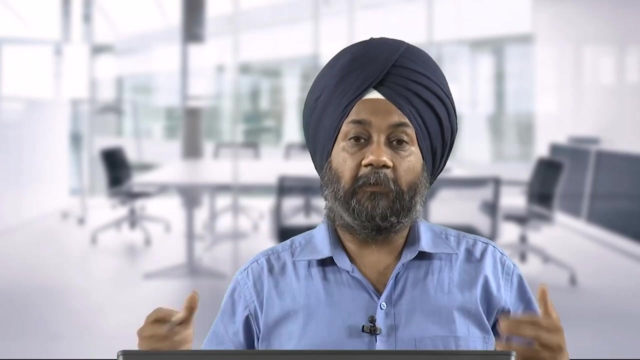 materials that are being used. more or less. there are standard guidelines which we are going to cover. We are not going to exclude those guidelines. we are going to cover those guidelines also for standard processes. But with new and new developments taking place, new and new requirements coming up for product, 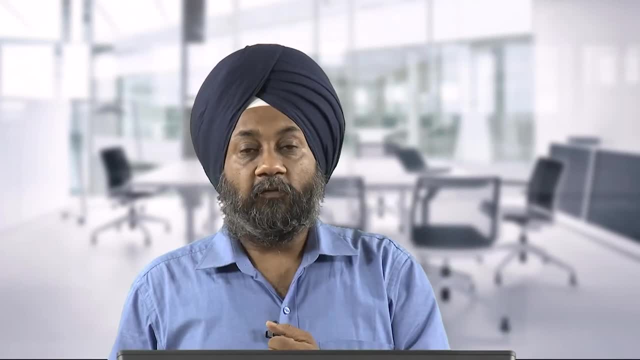 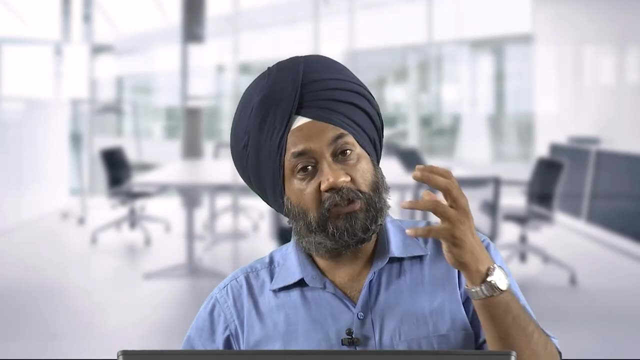 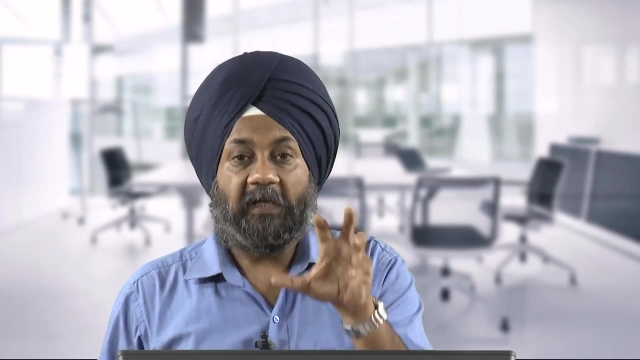 designs or for different types of products. We need to develop new materials, and for new materials we need to have new processing techniques, tools, and for these techniques there have to be standard guidelines which have to be established So that our product is made in a successful manner or made word, I can quote- it is processed. 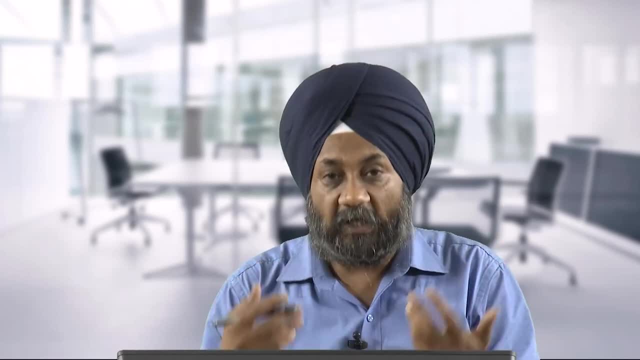 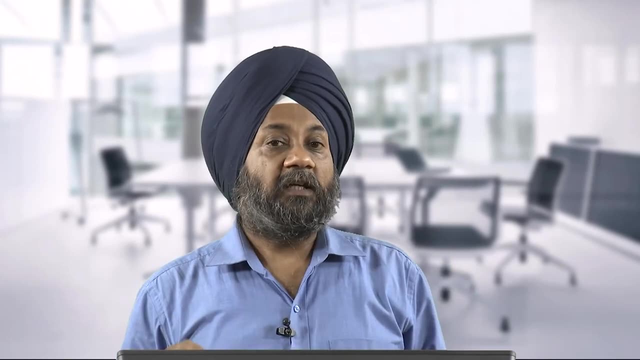 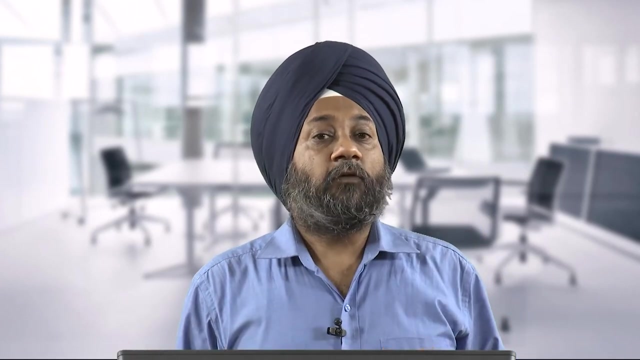 it is fabricated, it is produced, it is manufactured in the most economical manner to the best of quality. So that is our target: That once new materials are also coming into picture, we must be able to establish the manufacturing guidelines from the product design perspective and that we are going to see in our subsequent 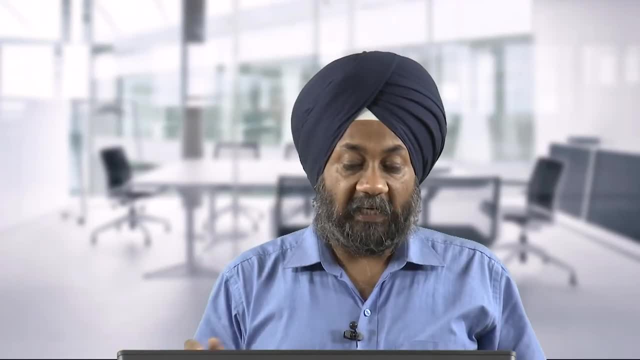 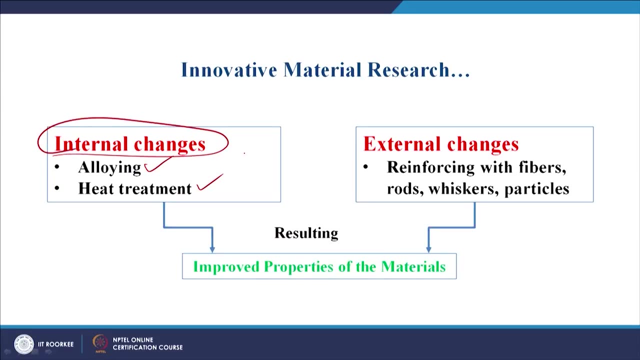 sessions. Now, new materials, how they can be developed. let us see we can do some internal changes in the materials, which can be alloying or heat treatment, or there can be some external changes Which can be this total weighting, Which can be this total weighting. 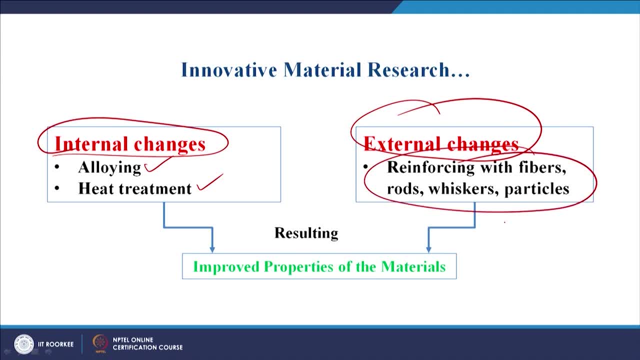 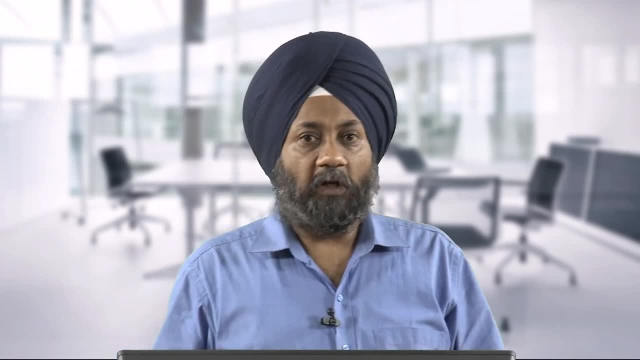 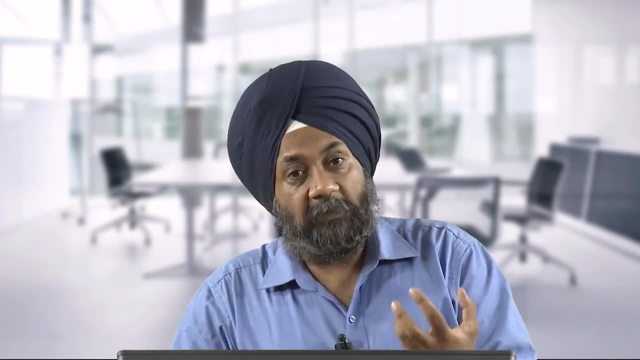 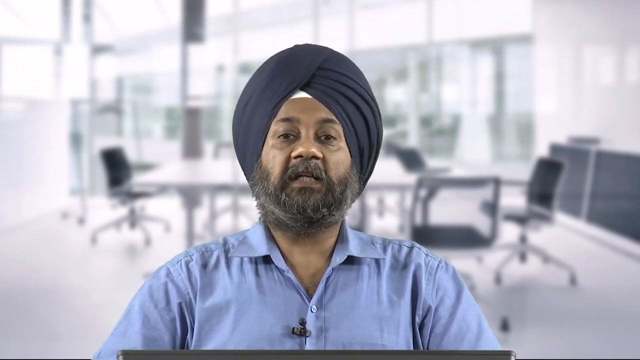 word composite and what are the different types of composite or how it is related to the course. The course basically tryst to establish the manufacturing guidelines which can be helpful for the product designers when they are designing new and new products, So these products can use different types of materials. now, materials can be metals. 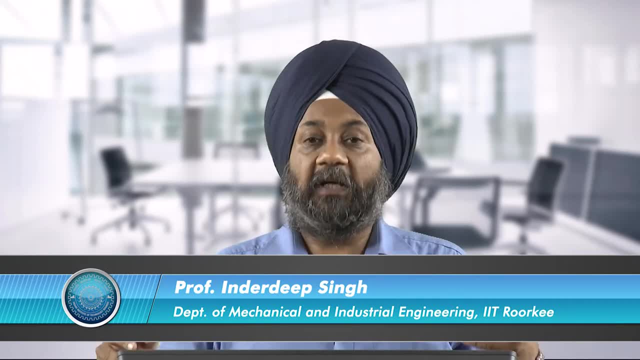 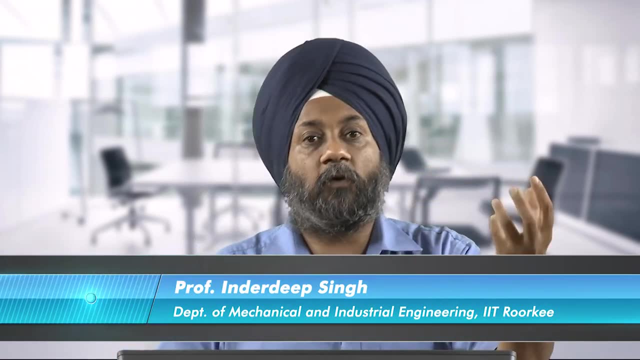 they can be ceramics, they can be wood, it can be a plastic, it can be a composite, it can be a shape memory alloy, it can be a nano material. So for a specific type of product, specific type of materials will be used, and for these 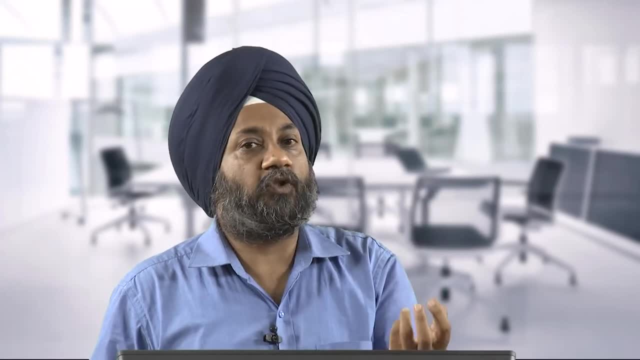 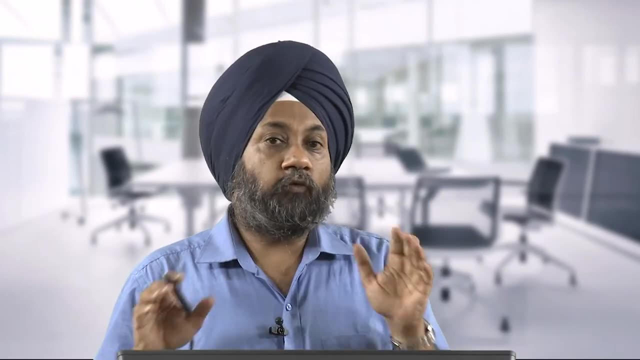 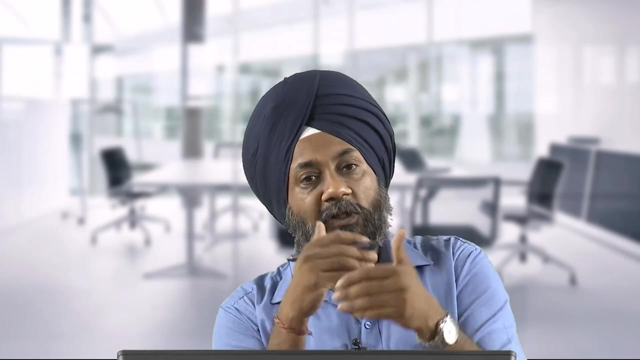 materials, there will be certain manufacturing processes. those will be used for converting them into the final product as per the product design. So our focus is to understand those manufacturing guidelines. but this slide is just giving an indication that how the new materials can be developed. 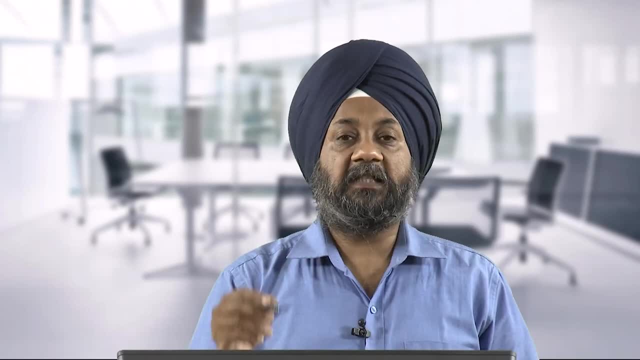 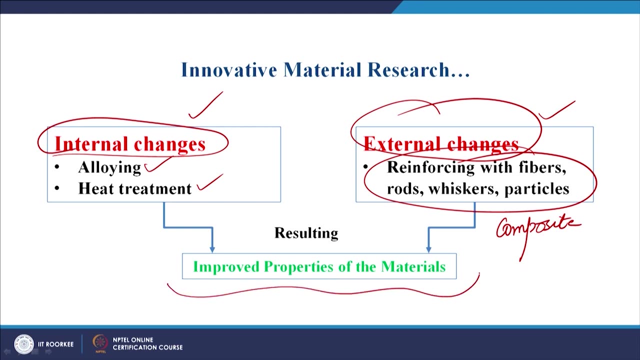 So new materials can be developed by doing the internal changes or the external changes. and once we try to develop a new material, it will lead to improved properties of the materials, How it is related to our course, because when the properties of the material will change, the manufacturing 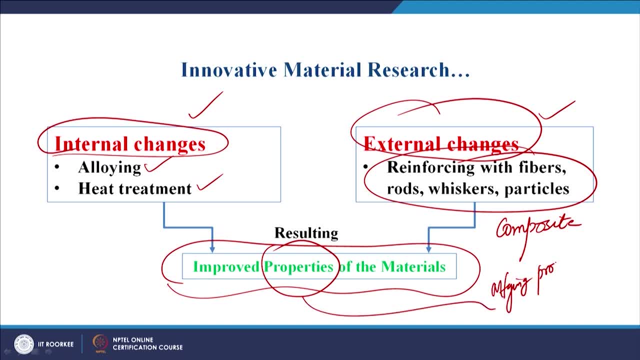 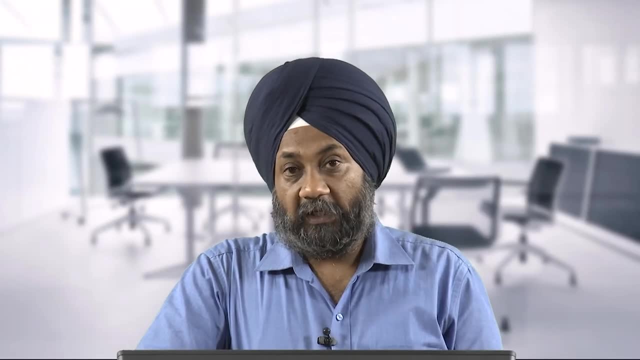 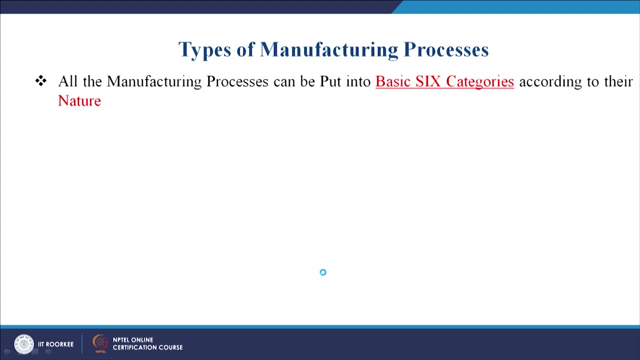 Processes also need to be controlled or also need to be designed in such a way that we are able to produce these new materials as per our product design. Now let us see the main topic for today, that what are the types of manufacturing processes? Now, all the manufacturing processes can be put into 6 basic categories. 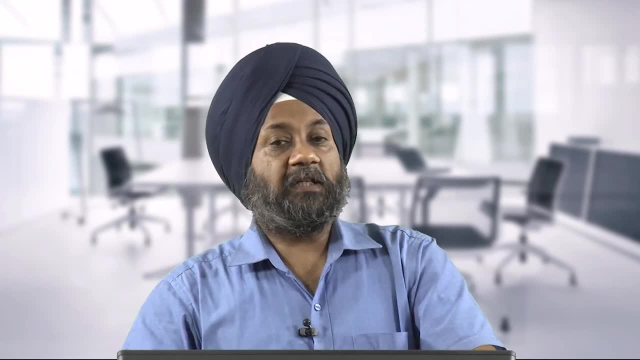 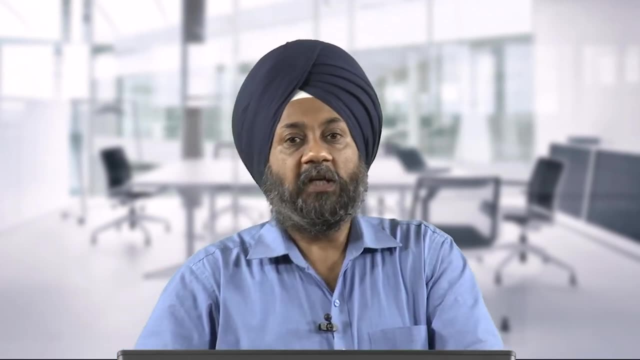 So we are not going to get into the intricacies of each, Each and every process, that how this process is done, But we will see that. what are the guidelines for this process? So we will be focusing on the guidelines majorly instead of focusing on the process. 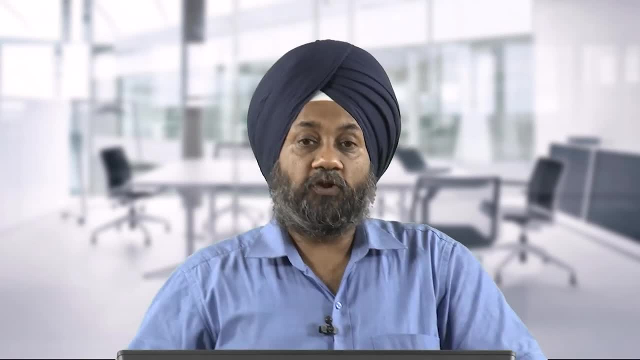 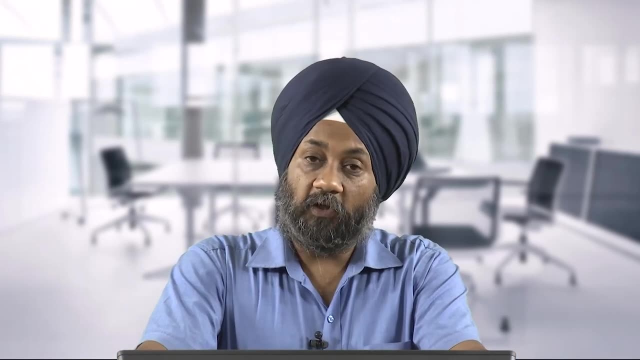 Process. if you are really interested to get to know about the process, that how the process is done, Then you must follow other courses which are already prevalent, which are already being run successfully, maybe for the last 1 or 2 semesters. So this is the main topic for today. 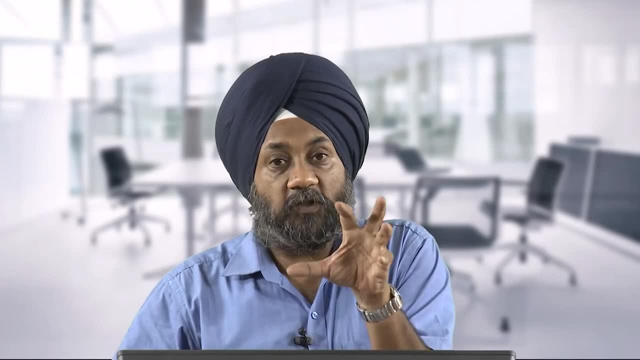 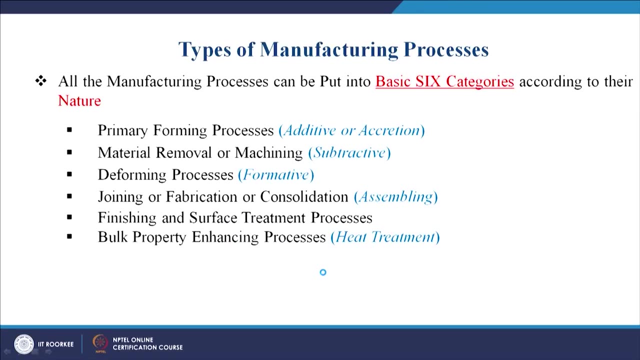 Thank you very much. Our focus is on the guidelines which are established for these processes. Now, what are the processes? These are the processes on your screen, The primary forming processes. one of the example here can be the casting process. Then we can have a metal removal already. the example is given: machining, which is the general. 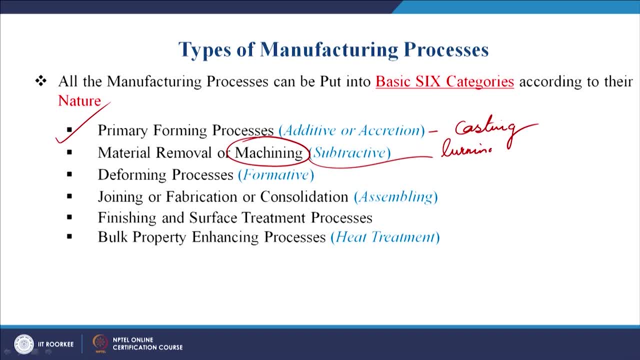 term. Then we can, within machining, we can talk of turning, We can talk of drilling. So we will have primary forming processes, We have material removal processes, We have deformative processes. We can take an example of extrusion here. We can take an example of rolling here. 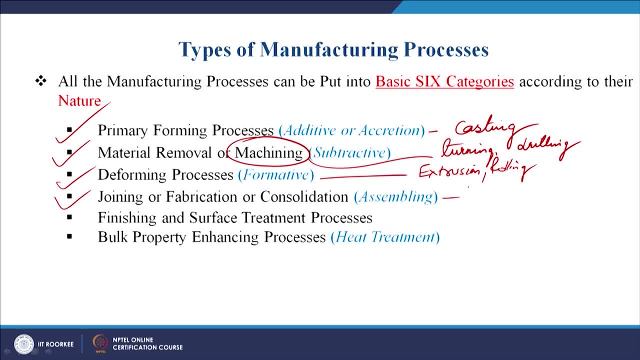 Then there are joining or fabrication or consolidation processes. We can take an example of welding, or we can take an example of soldering here. Then there are Finishing processes. Then there are finishing and surface treatment processes. we can take an example: finishing. 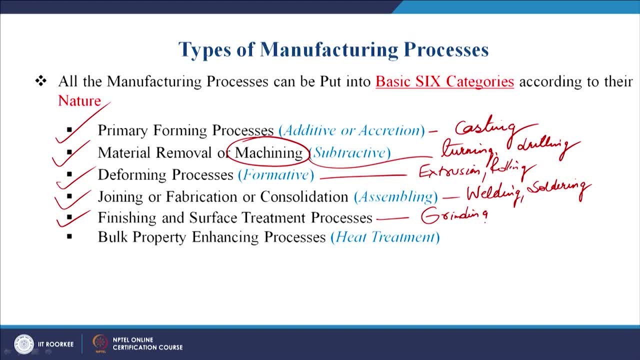 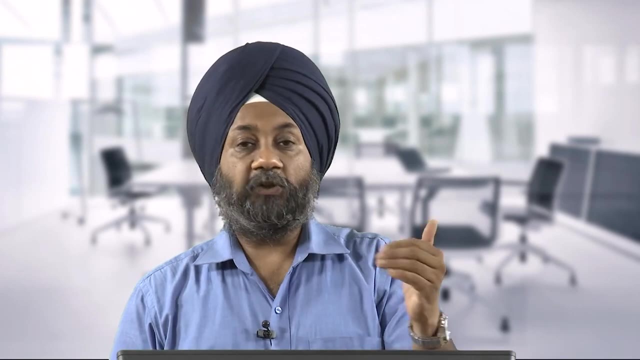 can be. one of the most common process is grinding. there can be other super finishing processes also, then bulk property enhancing processes such as the heat treatment. there can be processes like annealing, or we can have a tempering process also. So we can see that the general manufacturing processes can be classified into these basic 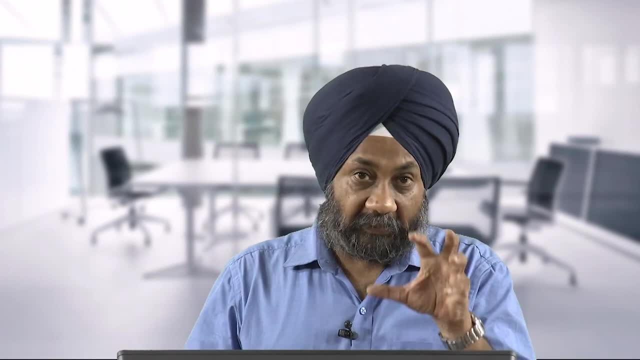 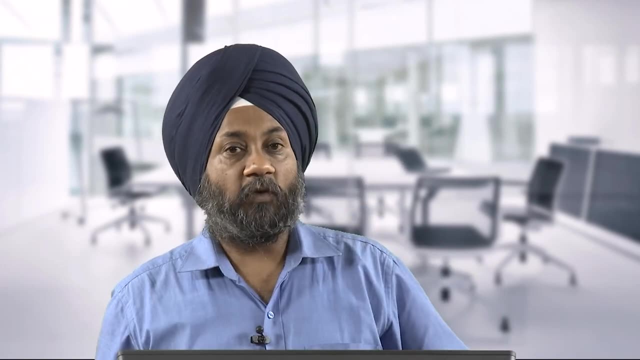 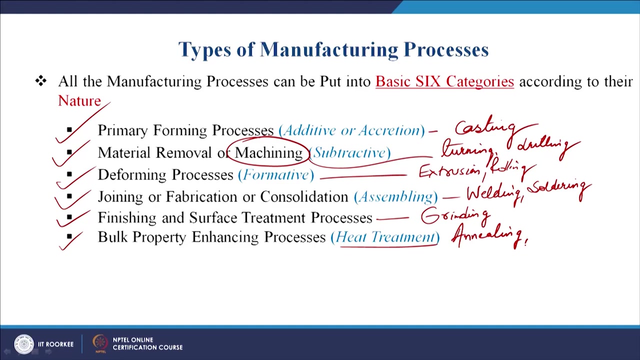 categories and we will try to understand the guidelines which have been established for some of these processes, because all we cannot cover in a short span of 20 hours. So our focus will be on the most commonly used manufacturing processes and how they can be, we can say, harnessed for making our products. 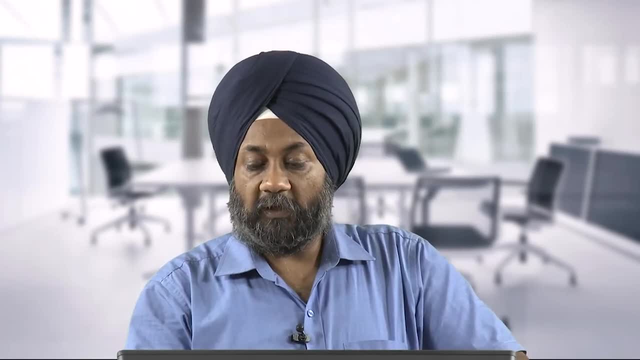 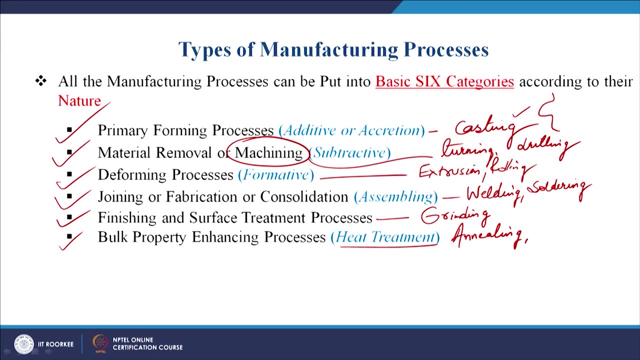 So that will be the main focus, That will be our target here. So in primary forming we have seen casting. so what are the guidelines for casting? So, for example, we can take a product which is something like this, which has to be made by casting. what are the guidelines for making this product as per our process of casting? 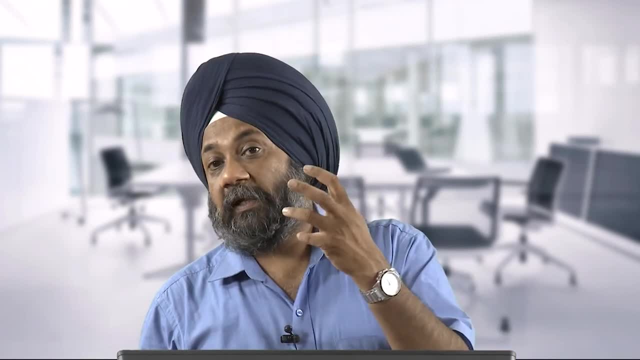 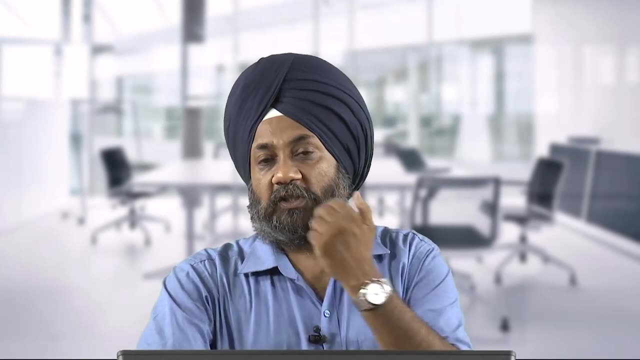 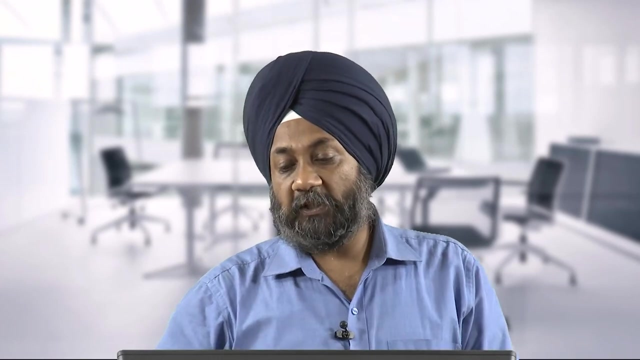 So we will see what are the guidelines or what important checks or what important requirements must be kept in mind Once this type of product is to be manufactured. that is a target that we are going to achieve after undergoing this course. Similarly for drilling, I have already taken an example in the previous slide that how. 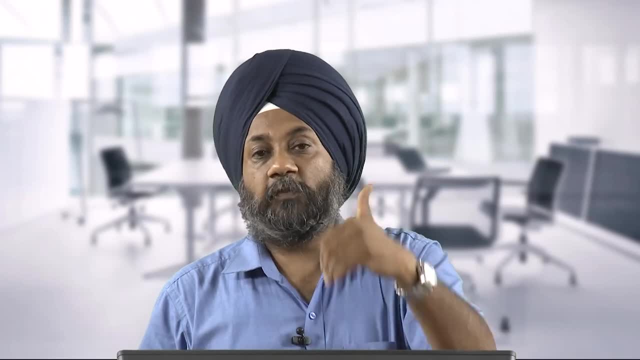 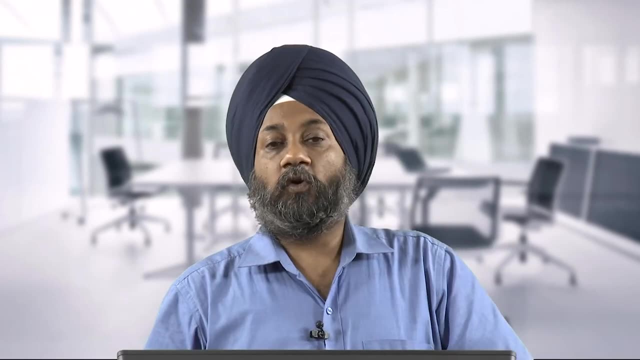 much portion or how much area of the hole must be within the plate if the hole has to be made at the edge. just one example of making holes. So, for hole making, what must be the difference between the 2 holes? now suppose drilling- 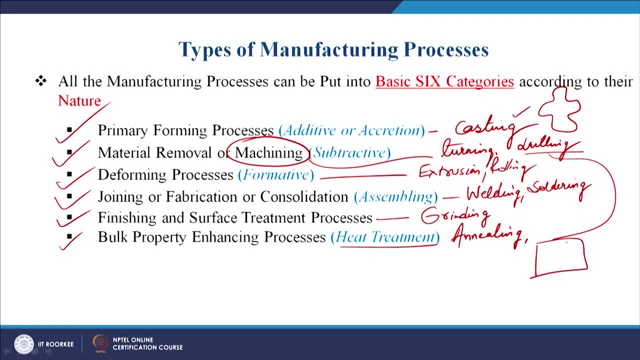 we can take. Let us take an example. suppose this is a plate. we want to make 4 holes, so what must be the centre distance from the edge, this distance x. or if we want to make a hole here, again what must be this distance x in order to make a good quality hole which does not serve to? 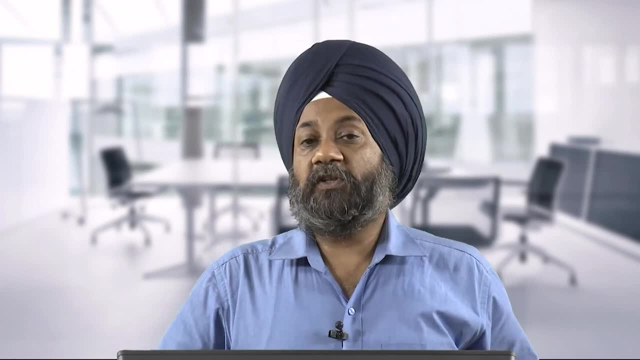 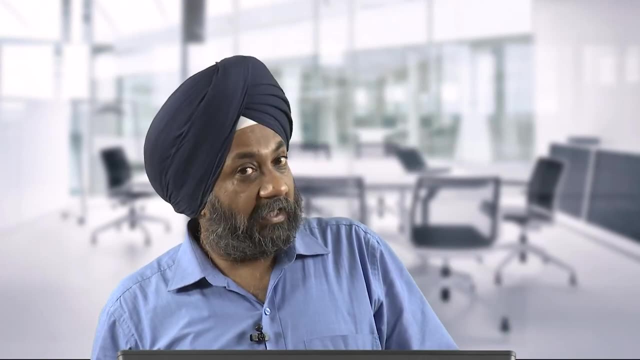 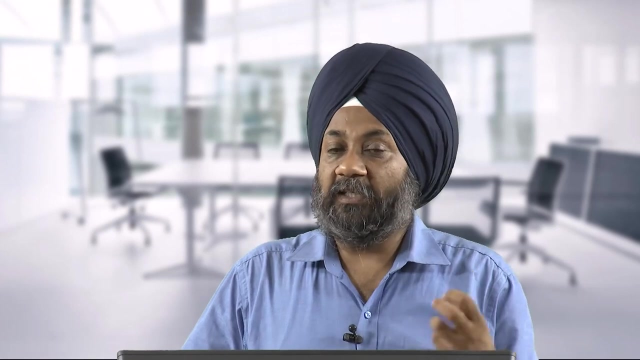 impair the performance of the product or which does not hamper the performance of the product. So all these guidelines is our target, And these guidelines will become a handy tool for each and every product designer, for each and every mechanical engineer who is involved in the product design process. 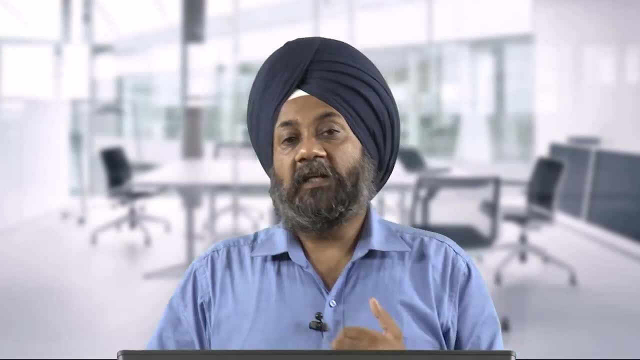 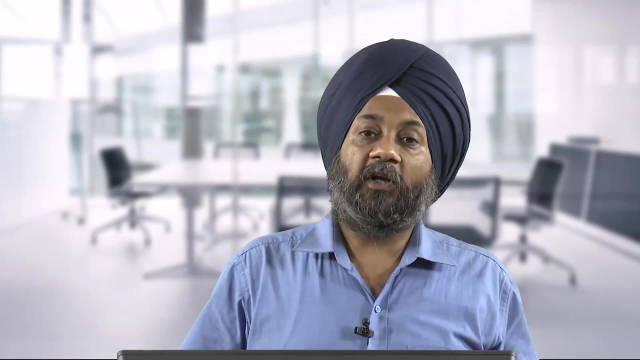 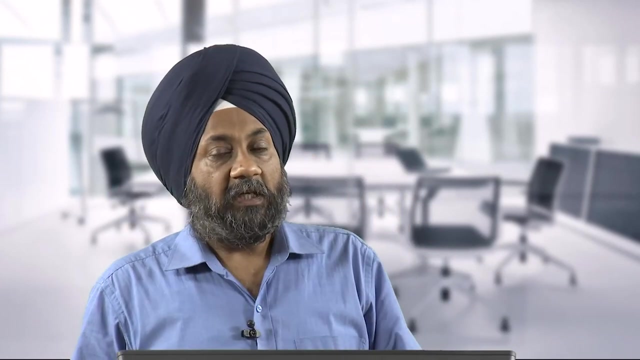 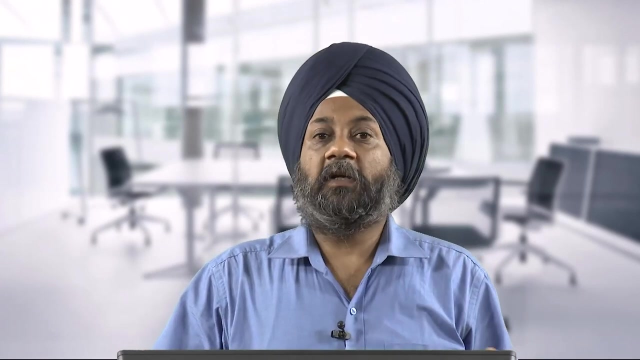 If these guidelines are followed religiously, the product will be developed to the best of quality and the iterative designs may not be required, Because many a time it happens that we have designed a product but once it goes into the actual manufacturing It is sent back to the designer with some notes, or with some suggestions, or with some. 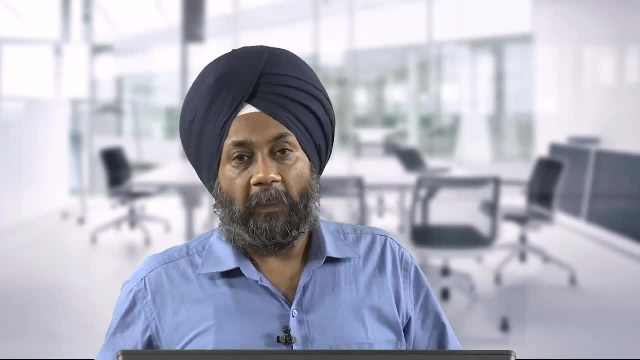 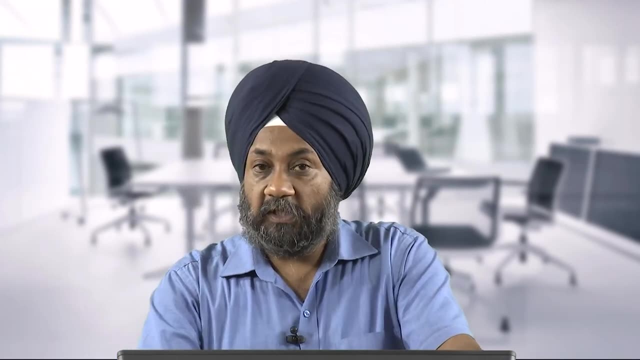 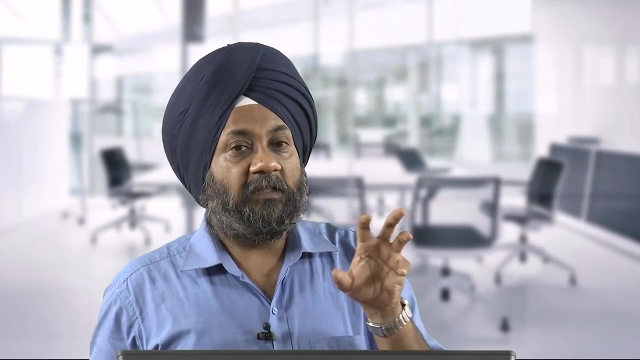 issues that cannot be addressed in manufacturing. So that is the basic concept for design for manufacturing or design for assembly. So our focus is more on the technical content because from design for manufacturing also 2 aspects are there. One is the hard core engineering aspect. 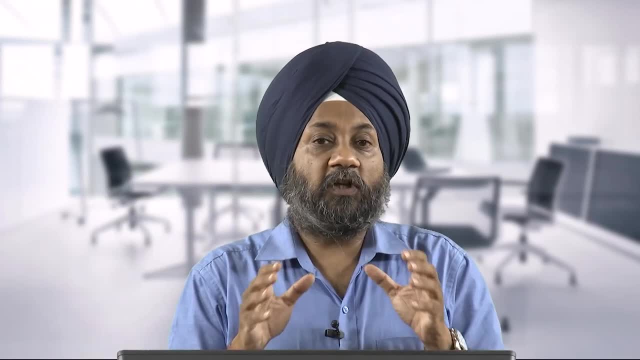 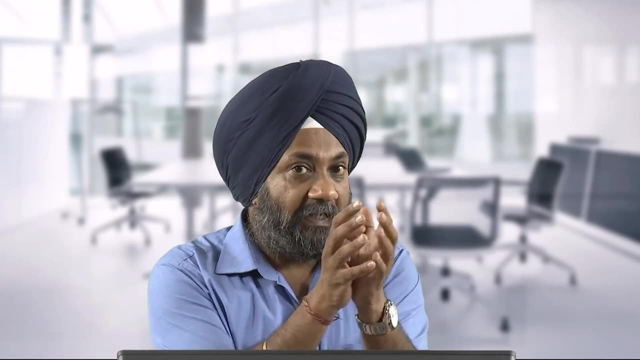 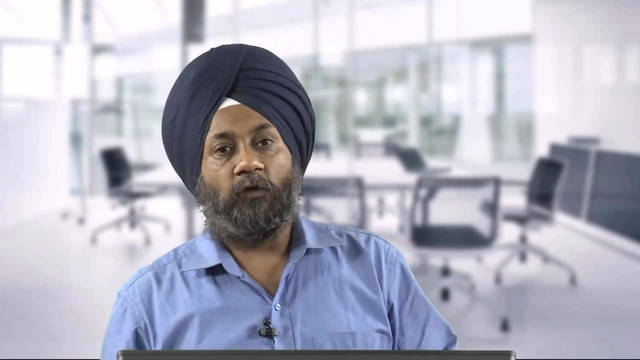 Another one is the industrial engineering aspect. Our focus primarily is on the engineering aspect for design, for manufacturing. So we will focus more on the guidelines related to the manufacturing processes which are helpful for the designers in the design of the product, So that iterative thing I was talking about that- once the design is final with the product. 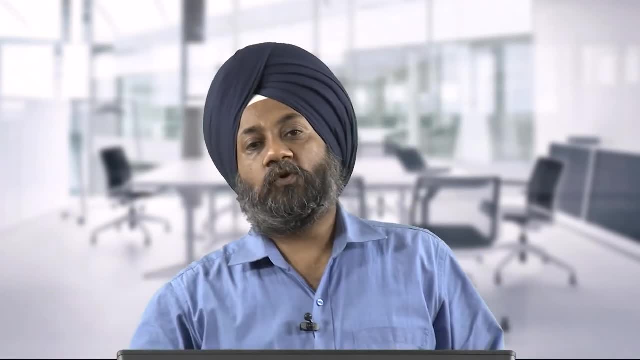 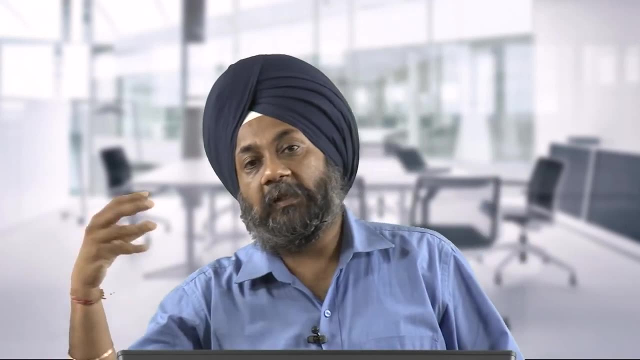 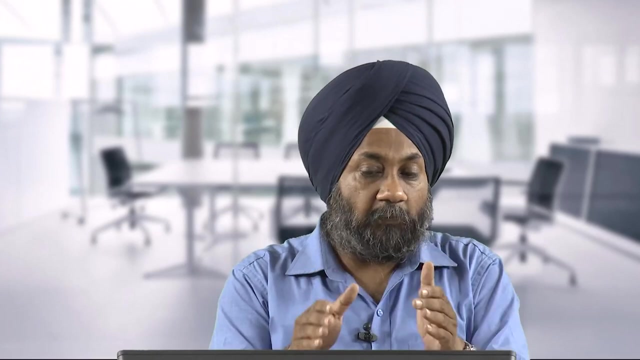 designer, It goes to manufacturing And then it has to come back sometimes Because of lack of consistency in the thought process of the designers and the people who are actually responsible for manufacturing the product. So that can easily be avoided if the designers keep all these manufacturing guidelines in. 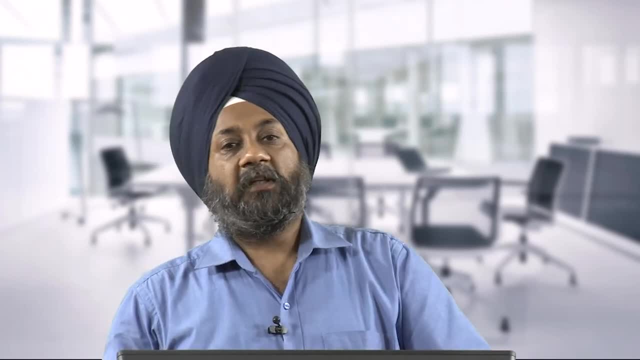 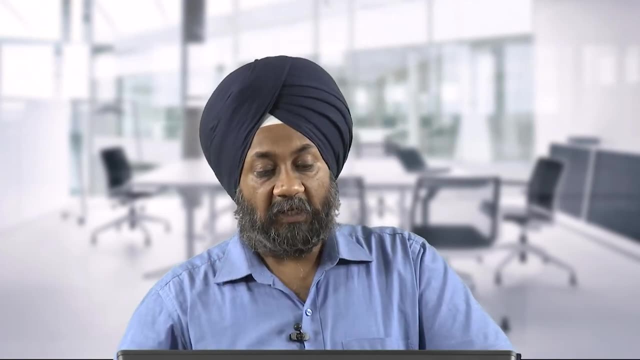 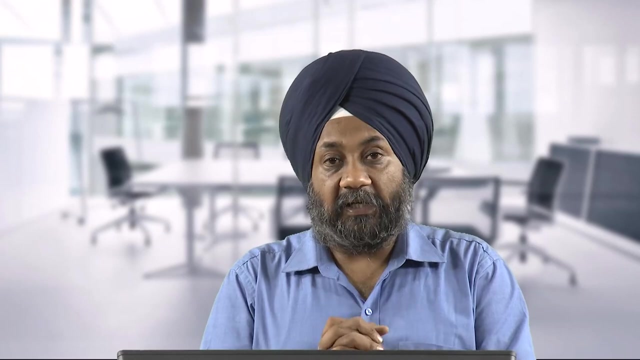 their mind related to the various processes that are going to be used for fabricating the product. So 2 or 3 examples I have taken, so we may not be going into the entry cases again and again I am emphasizing, we are not going to study casting in detail. 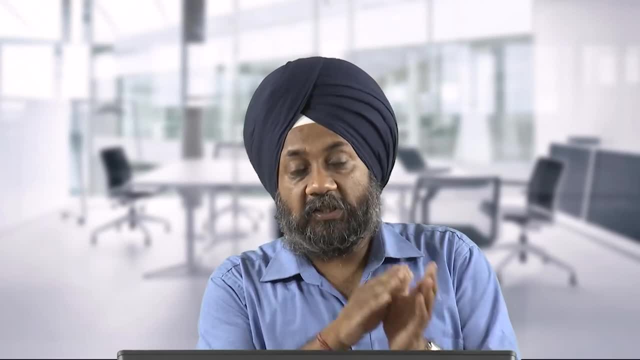 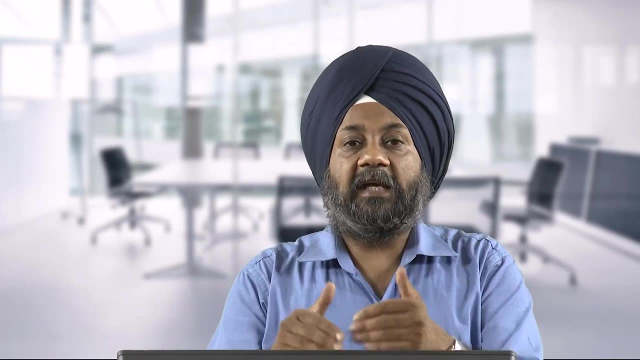 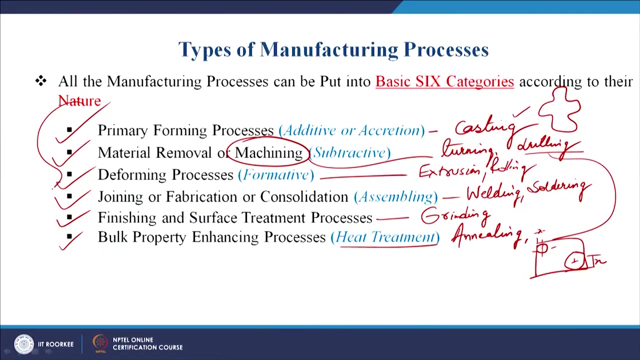 But we are going to study casting details or casting guidelines as applied to product design. Similarly, machining guidelines as applied to product design process. So that is the target. So these are the broad, we can say, classification of the manufacturing processes. Let us see another slide which will make them further clear. 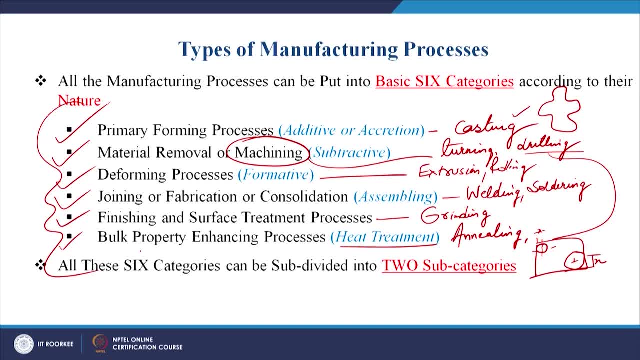 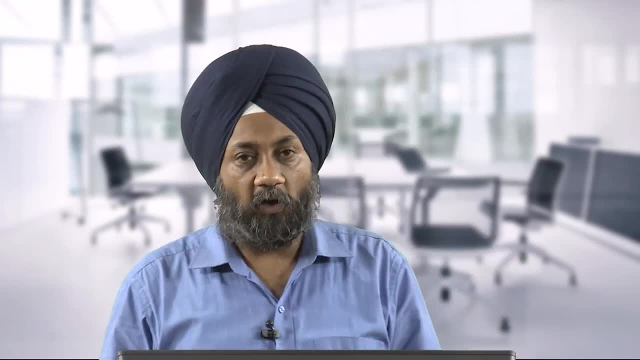 So these are the 6., 6 categories. then there can be 2 subcategories. also We can have these processes which can be conventional or sometimes unconventional or advanced. Now, what do we? what can, how can we differentiate? Now, conventional processes are processes which are used for so many years and which have 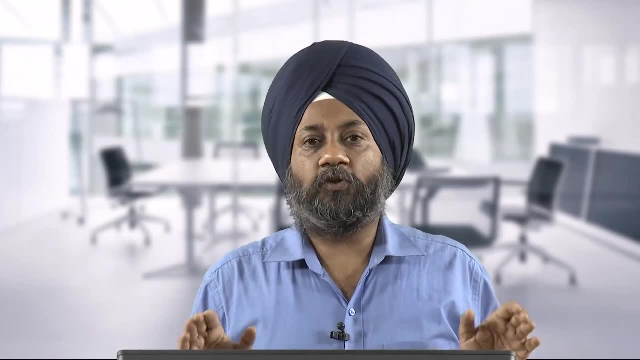 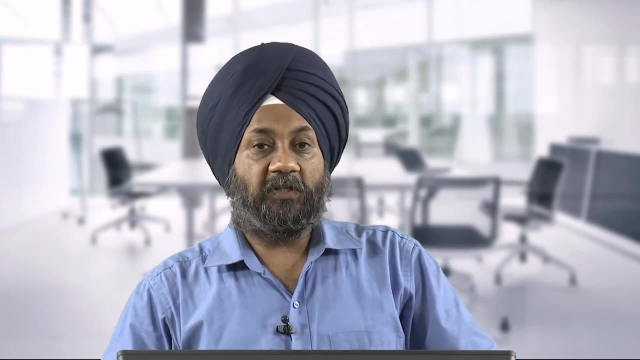 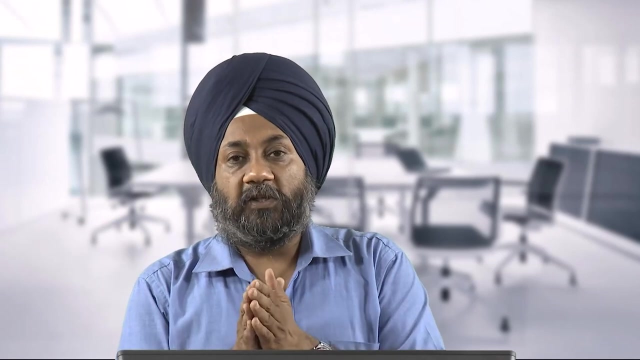 established themselves as the commercial processes for manufacturing of products or manufacturing of materials, But unconventional processes. But unconventional processes Sometimes, which are may be in the research stage or which are beyond the conventional processes, For example in conventional machining. the tool will come in contact with the work piece. 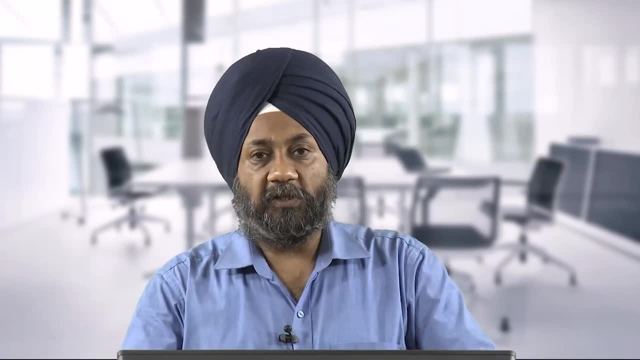 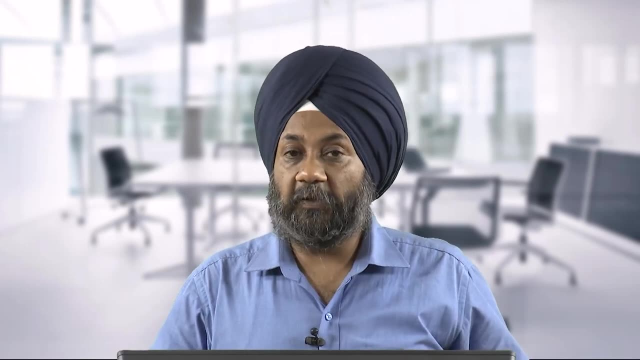 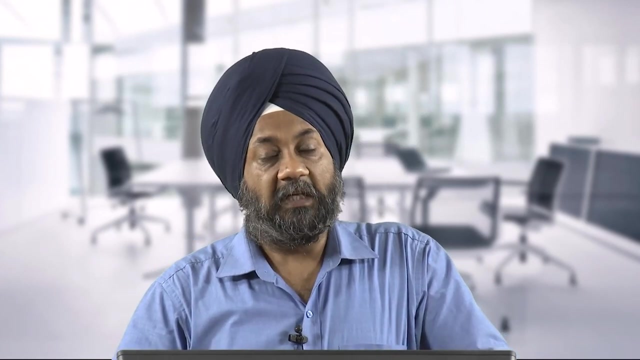 and will remove the material in most of the processes, Whereas in unconventional method of removing the material, the tool may not come in contact with the work piece, So the material may be removed by other actions. sometimes the abrasive action can lead to removal of material. 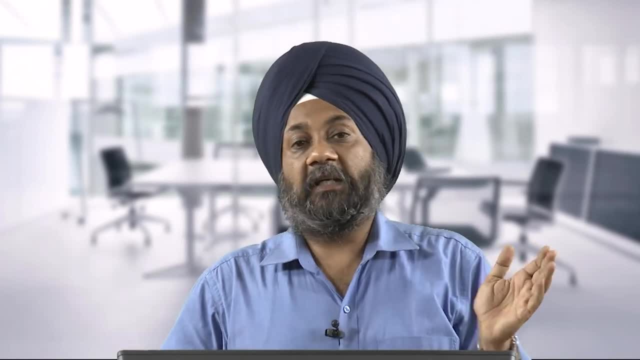 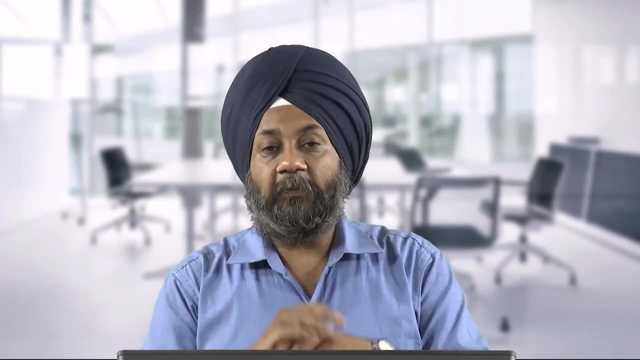 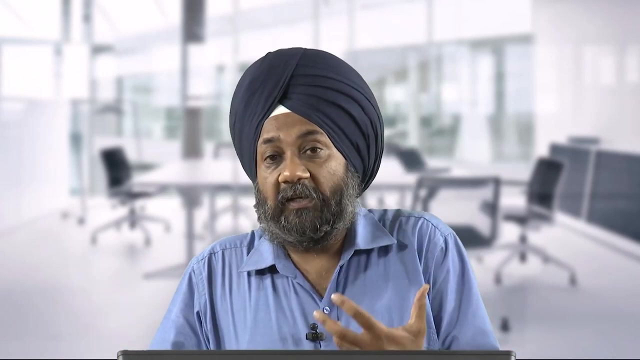 Sometimes Vaporization of the material, melting and vaporization may lead to removal of the material. Sometimes it may be removed by only by the application of heat. So but the tool is not coming in contact with the work piece, So that is something which is unconventional. 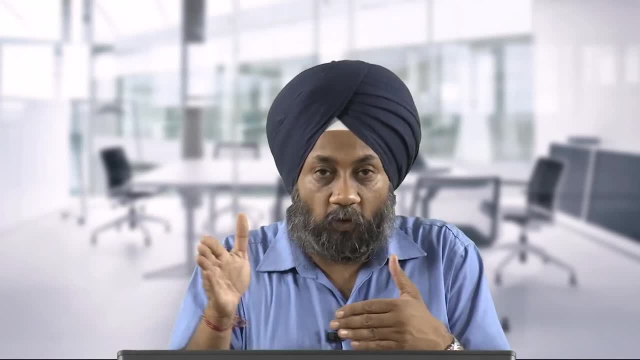 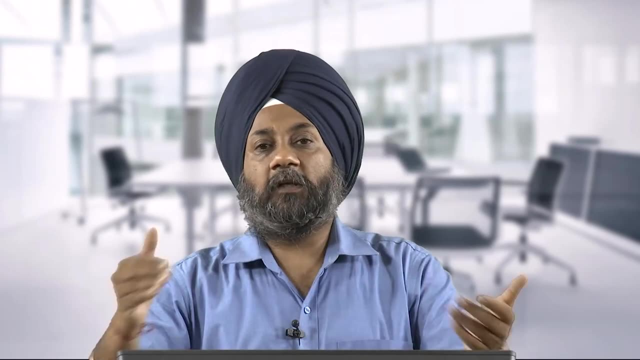 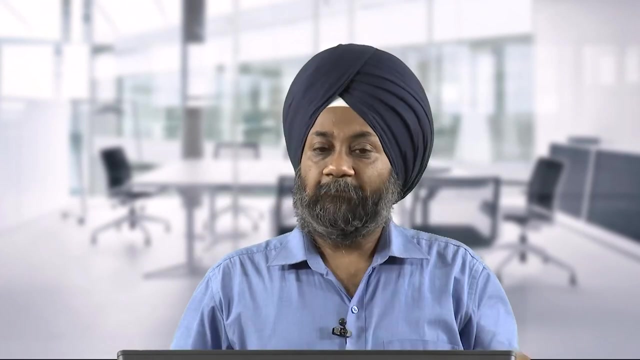 Conventionally, whenever we remove the material, we feel that the tool will come, it will rub against the work piece and remove the material, Whereas in unconventional approach, the tool and work piece are out of control, or maybe not out of control, I must say, are not in contact with each other. 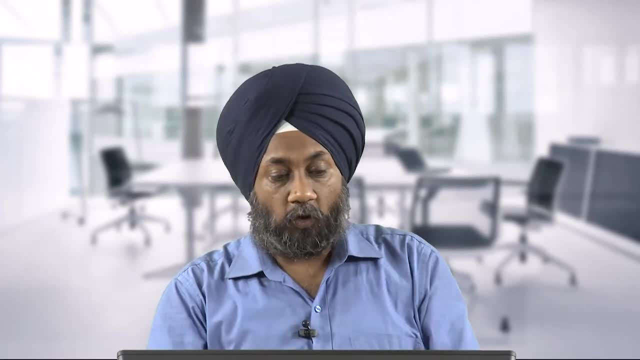 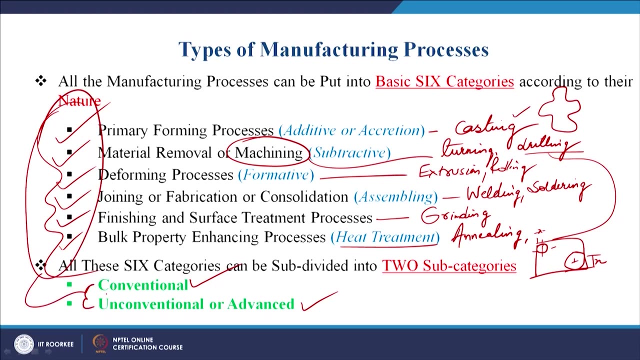 So that is the basic difference between conventional. So all these 6 processes that we have listed here can further be classified as conventional and unconventional. For example, usually it becomes clear in conventional processes or conventional machining we can take a process for hole making as drilling. 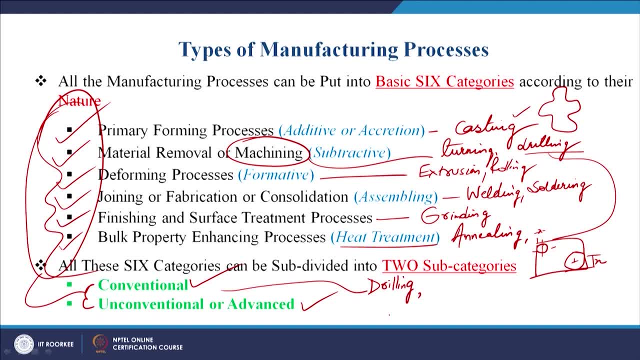 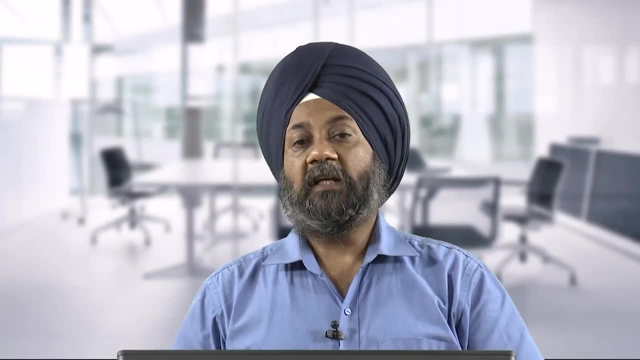 But if we talk about unconventional, we can have a process called EDM, which is electric discharge machining. So we can make a hole using EDM also and we can make a hole using conventional drilling process also. But what is the difference in conventional drilling? the tool will be in contact with. 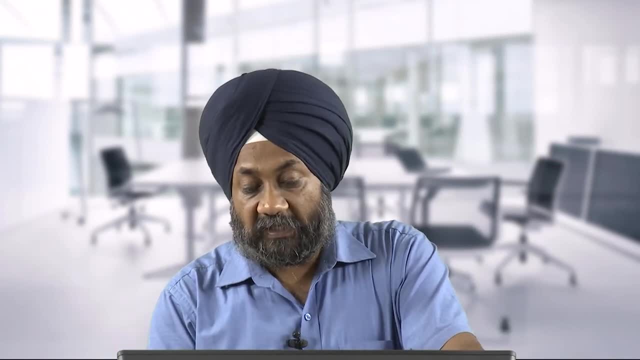 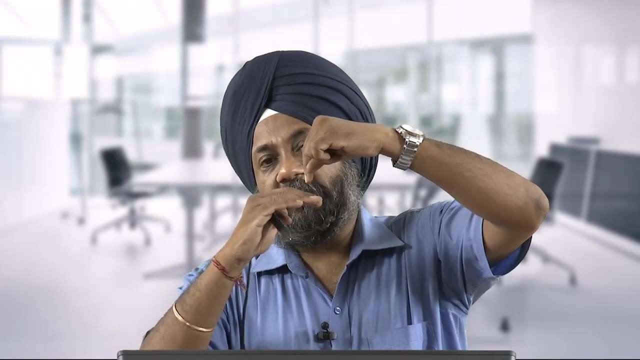 the work piece and physically the material will be removed, Whereas in EDM process the tool will not be in contact with the work piece and only the spark That is the work piece. So that is the difference: The spark is generated between the tool and the work piece will remove the material from. 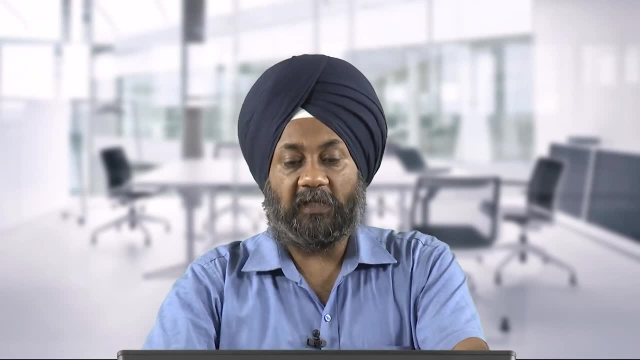 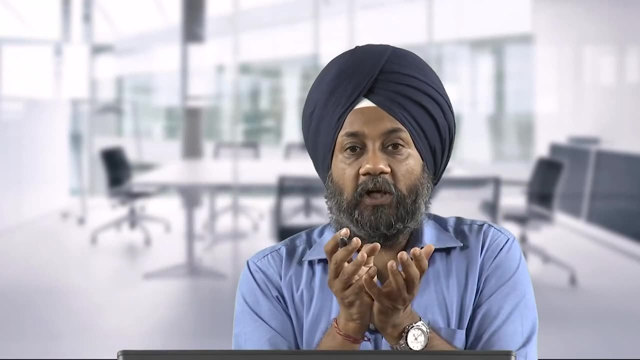 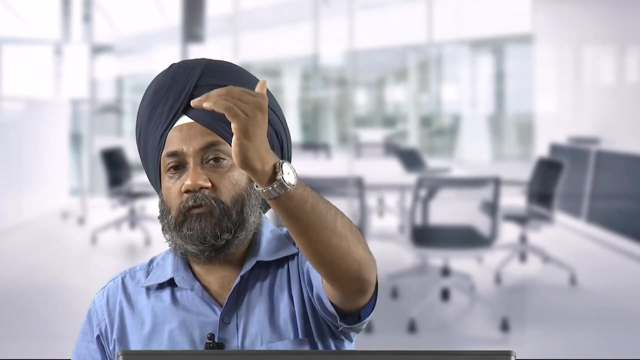 the work piece and a hole will be created. So that is the basic difference between conventional and unconventional And if you see the list you can easily categorize into a tabular form name of the category that is primary forming. Then you can write what are the conventional primary forming processes. 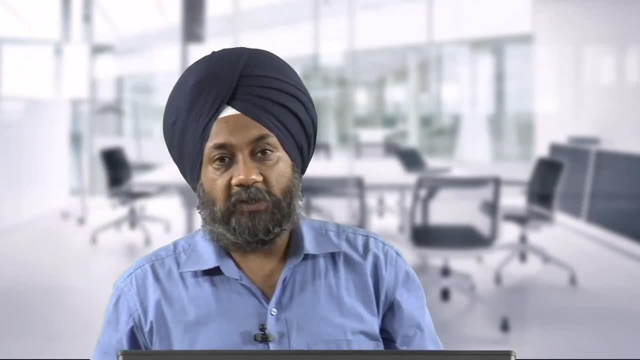 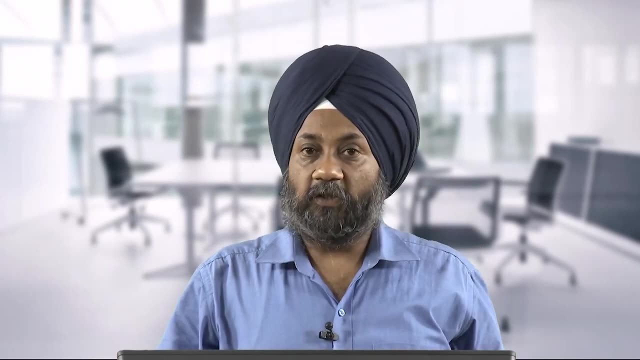 Next column can be: what are the unconventional processes? So you can have conventional primary forming, You can have unconventional primary forming processes. So that way you can classify, and I think this is a good assignment for all of you in the very beginning of the course. 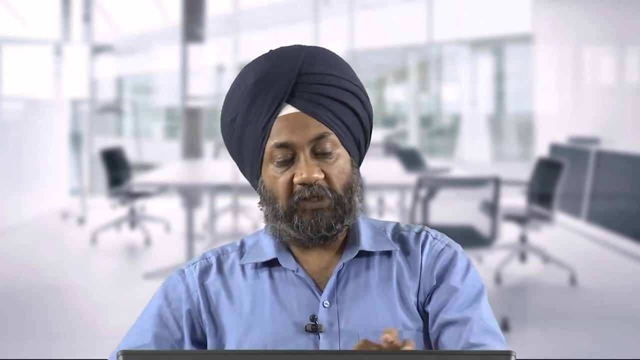 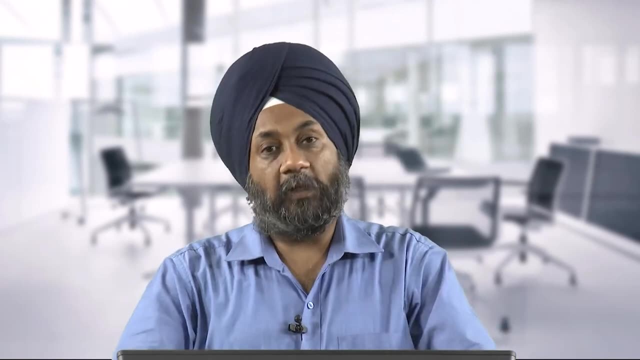 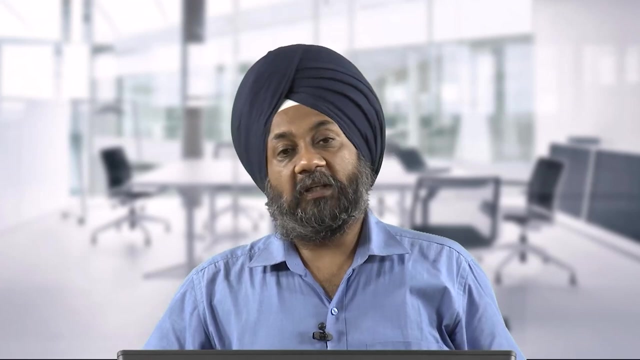 That when you are classifying the manufacturing processes, 6 categories already told, Then the subcategories. you can take an example in different books. You will find it in the tabular form that what are the conventional primary forming processes? What are the conventional material removal processes? 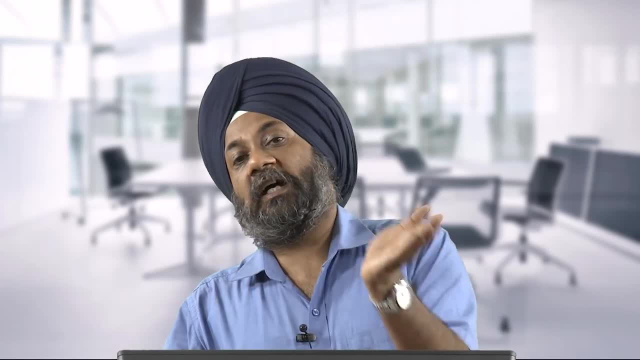 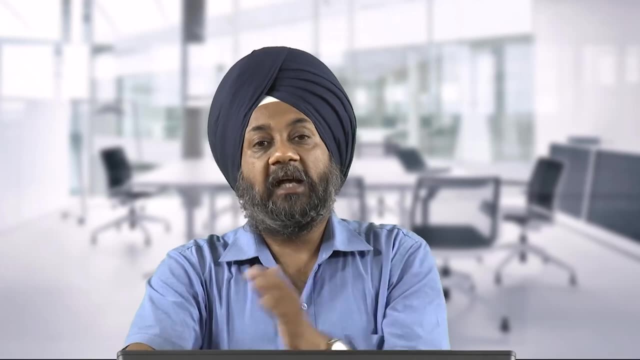 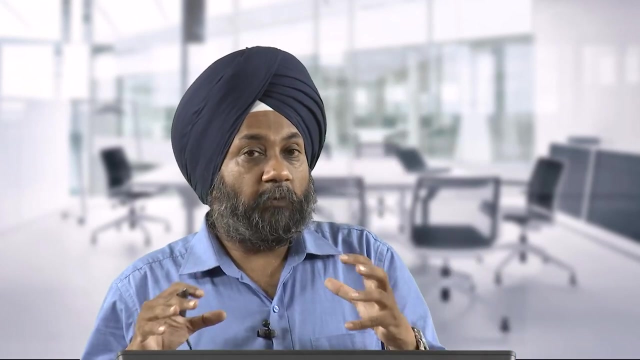 What are the conventional deformative processes, As well as What are the unconventional primary forming, unconventional machining or unconventional material removal processes, as well as unconventional deformative processes. So I can take examples of each one of these, But due to the paucity of time and the focus area of our course, I am not going to get into. 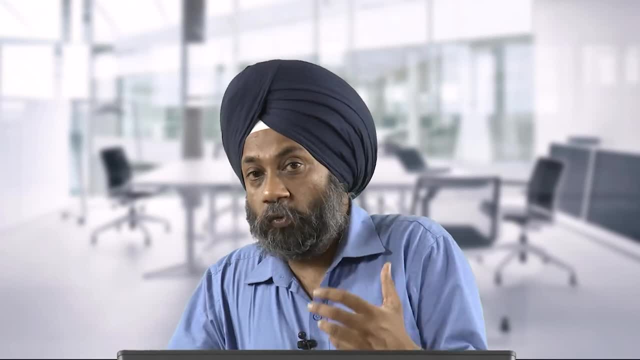 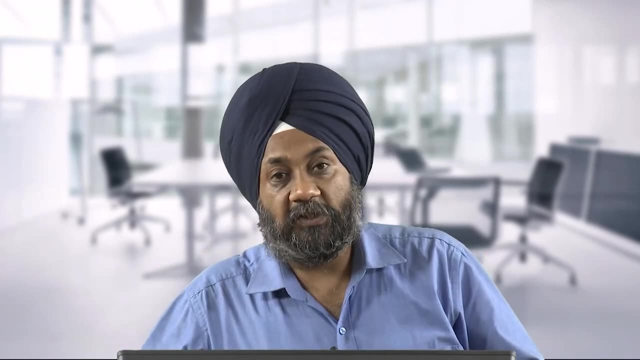 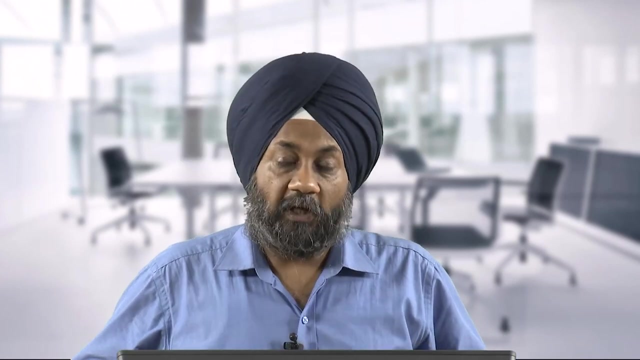 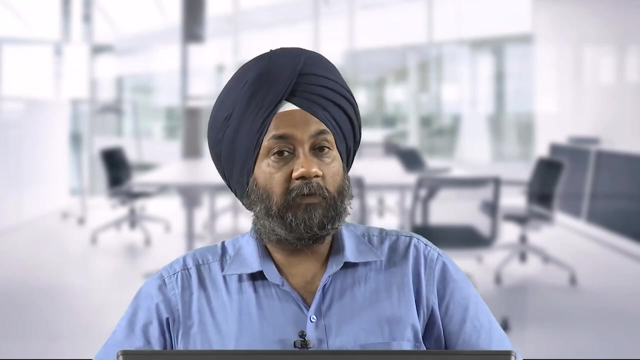 all those details. Otherwise, maybe just to explain to all of you, just one more example. if we talk about the deformative processes, Okay, The conventional can be rolling process, it can be extrusion, it can be wire drawing, tube drawing. All these processes will fall under the conventional deformative processes or conventional deforming. 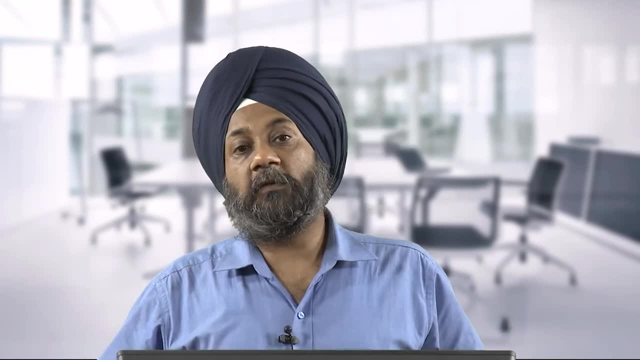 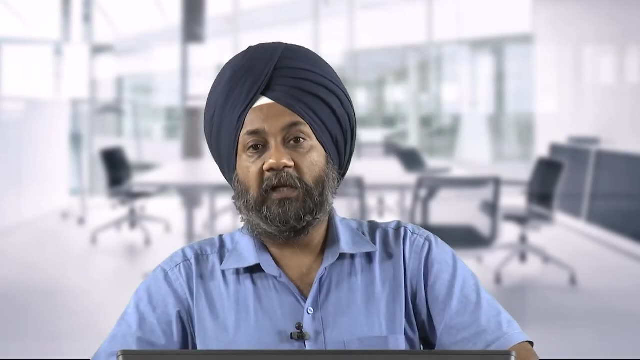 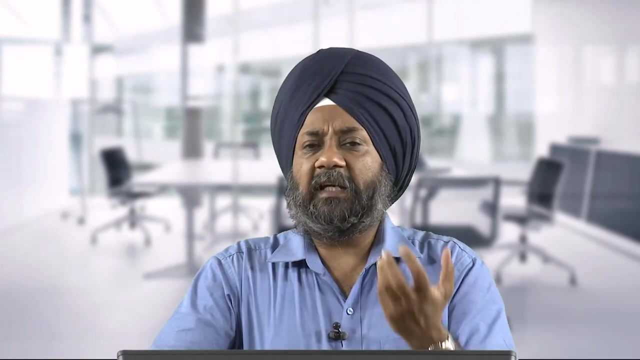 processes. But if you go to the unconventional deforming processes, you can take the example of explosive forming, You can take the examples of hydro forming. So you have different ways of deforming the metal. Okay, In the previous case we have taken conventional techniques like rolling, extrusion, wire drawing. 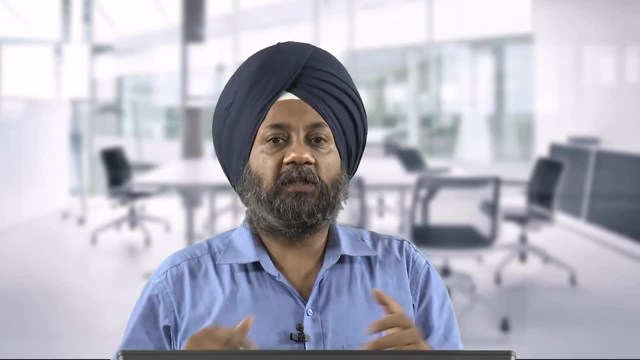 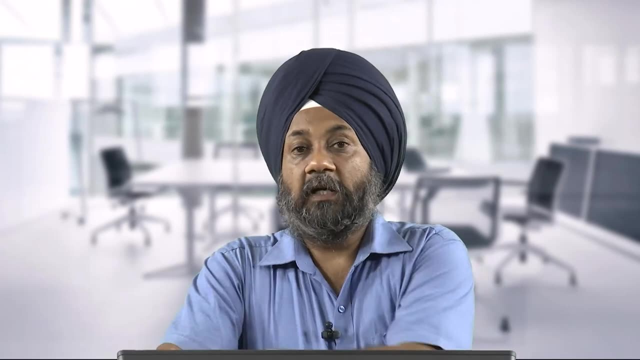 tube drawing standard processes which are used for changing the shape of the metal, Whereas from the unconventional side we are talking about 2 different examples. just now I have taken Explosive forming. you use the detonation and you explode. the waves will deform the. 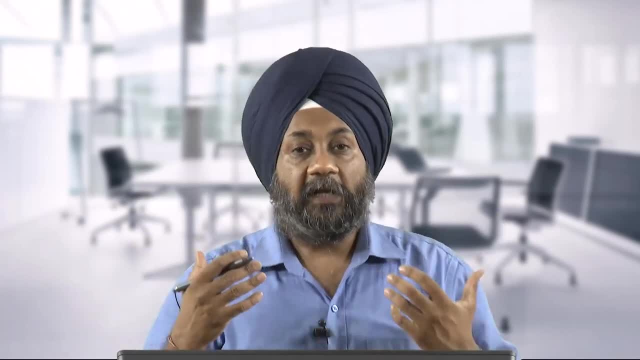 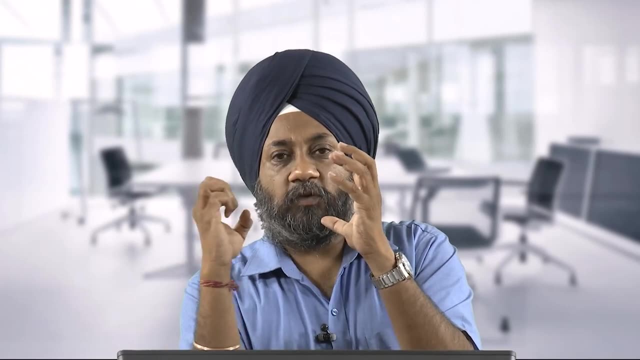 sheet in the form of the die in which it we are hitting it against. So there may be a die, there may be a sheet, and there may be a detonation And explosive as soon as the waves will hit the sheet. the sheet will take the form of: 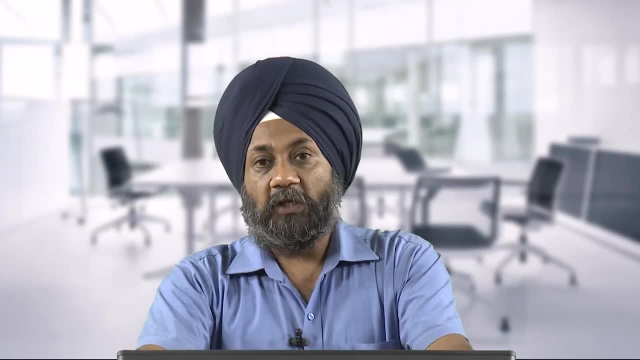 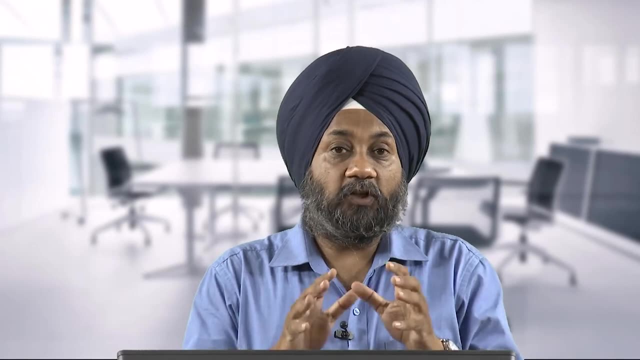 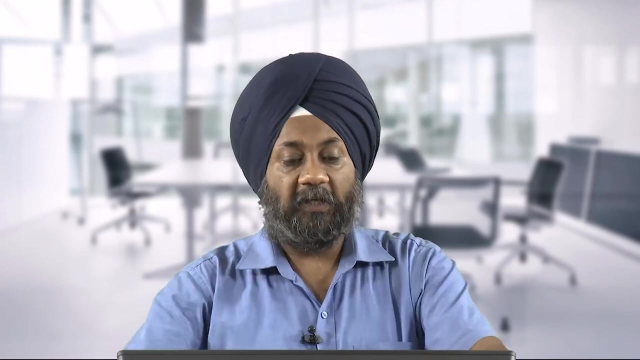 the die after the explosion. So we can have unconventional deformative processes also. So this example I have taken just to give you an idea that all these processes that are listed here- 6 processes are listed here: Primary forming, material removal processes, deformative processes, joining processes. 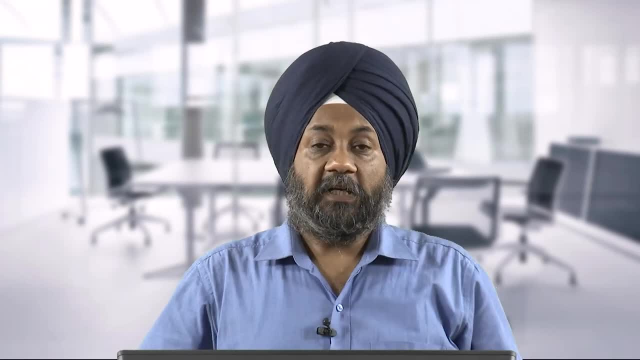 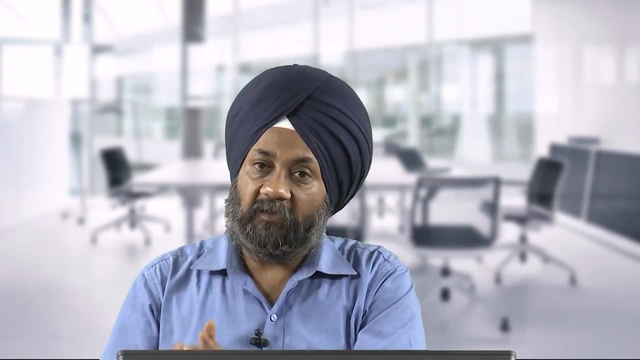 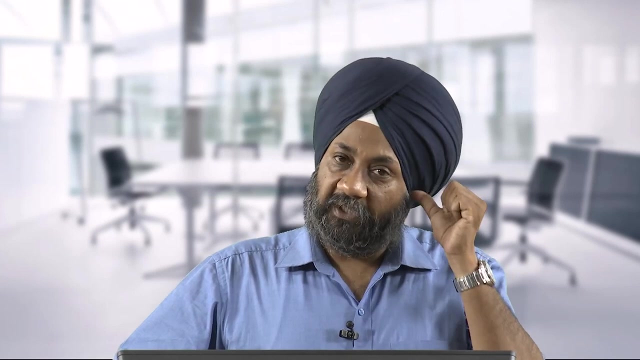 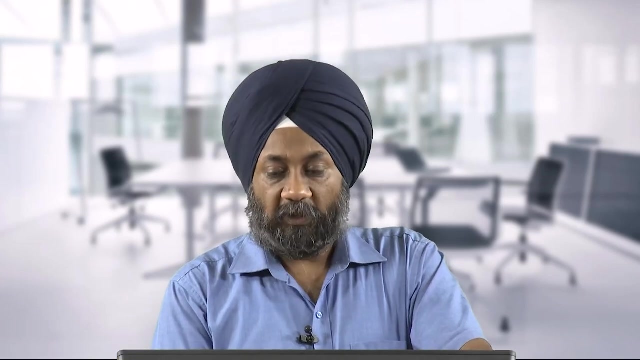 finishing processes, Bulk property enhancing processes. each one of this process can be both having conventional processes as examples as well as unconventional processes as the examples. Two examples already I have taken. first one was related to the material removal processes. the second one is related to the deformative processes- 2 examples already taken. 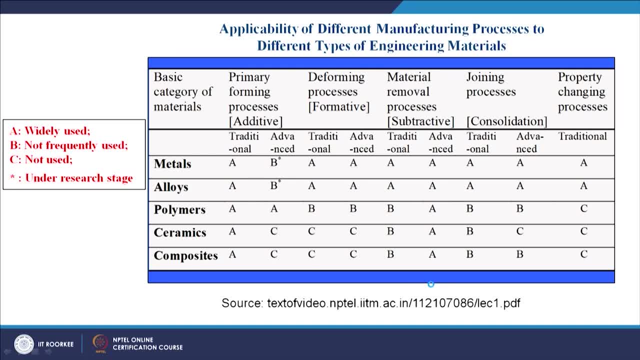 Now this is the source- is given applicability of different manufacturing processes to different types of engineering materials. So this is the list of processes on your screen You can see here. these are the processes which we have already covered: Primary forming processes, deforming processes, material removal processes, joining and property. 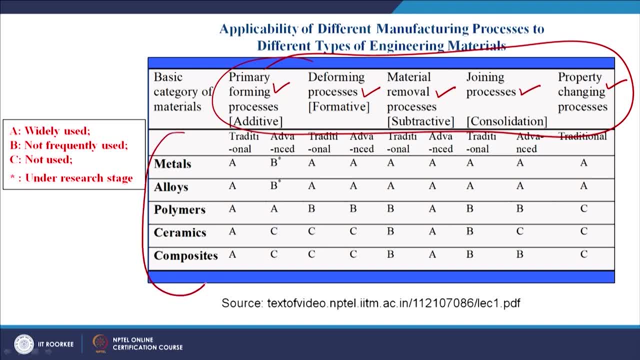 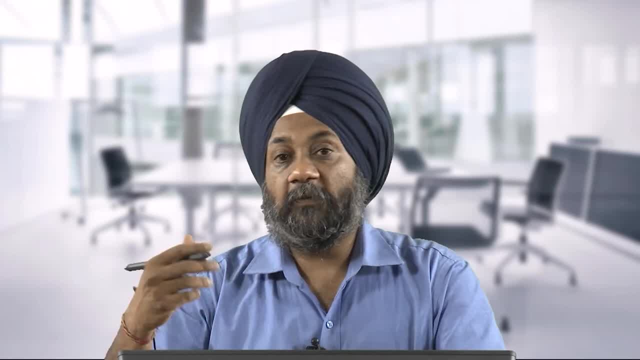 changing processes. These are the engineering materials which we are going to cover in our second week of discussion. that what are the various engineering materials and what type of products can be made. What are the manufacturing limitations for these type of materials, or what are the manufacturing? 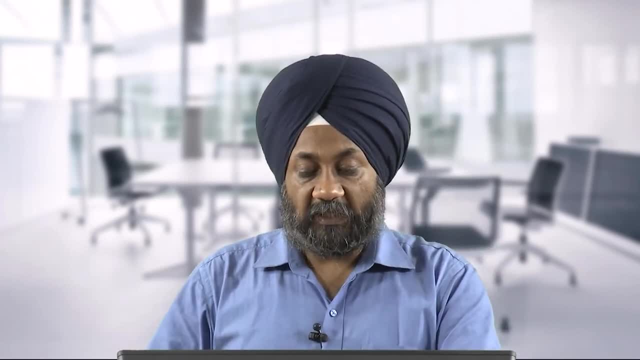 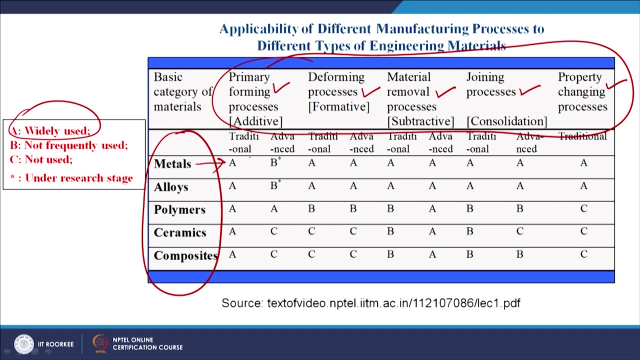 limitations for these type of materials. So we can see that A is widely used. So for metals, if you see in this column most of the processes are well established. So we have A in most of the processes. so metals can be easily fabricated or easily. 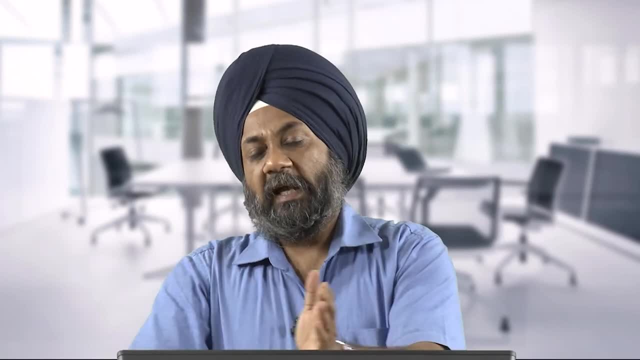 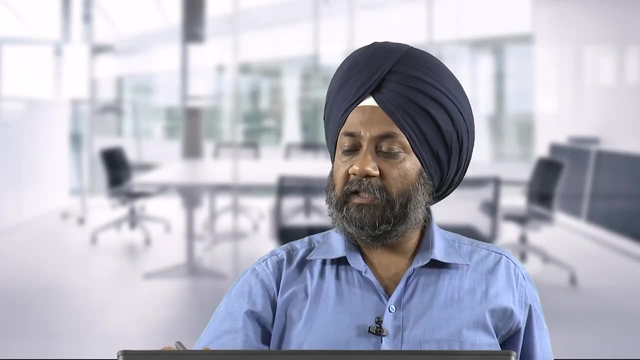 processed or easily produced or manufactured. Okay, So we have A in most of the processes, so metals can be easily fabricated or easily manufactured using any of these processes, depending upon the specific requirement we will choose. If the 2 parts have to be joined together, definitely we will go for a joining process. 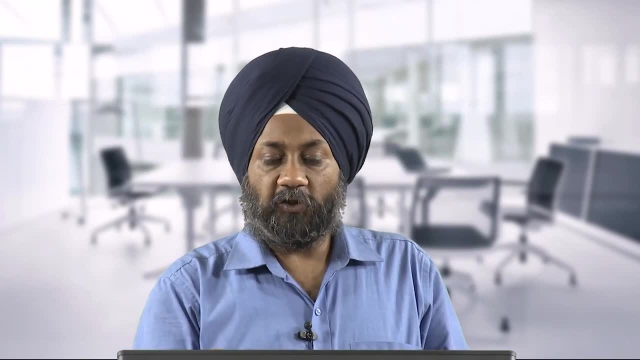 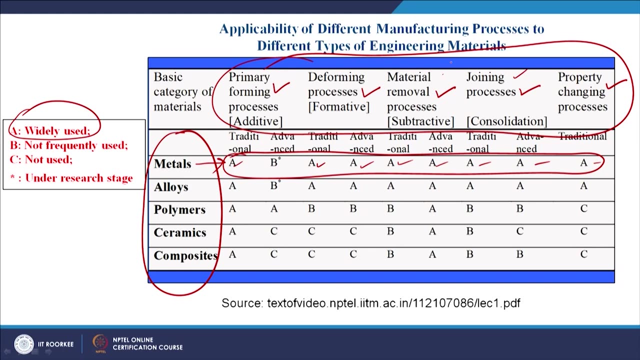 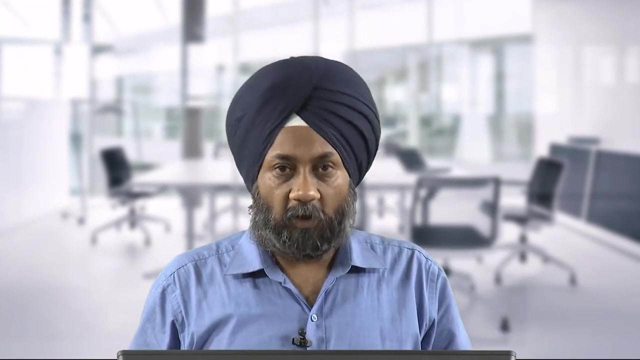 or if holes have to be made, we will go for a machining process or the material removal process. So specific requirements will lead to use of specific processes, but metals. it is established that most of the processes are well known or well researched, As well as well commercialized, whereas if we take any other examples- let us take the. 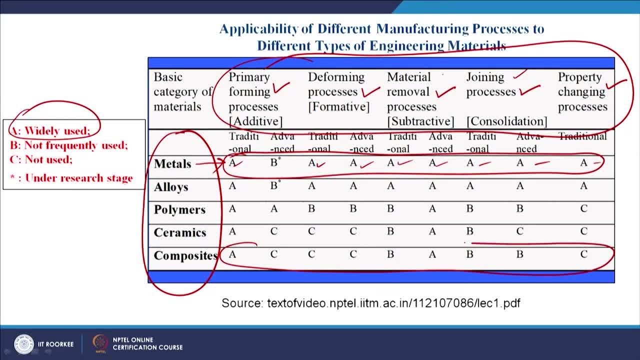 example of composites. So here you can see there are number of C. so C means not used. So you have a C here, C, C, another C here, and B is not frequently used. So we have a B here, we have a B here and we have a B here, which means that for composites 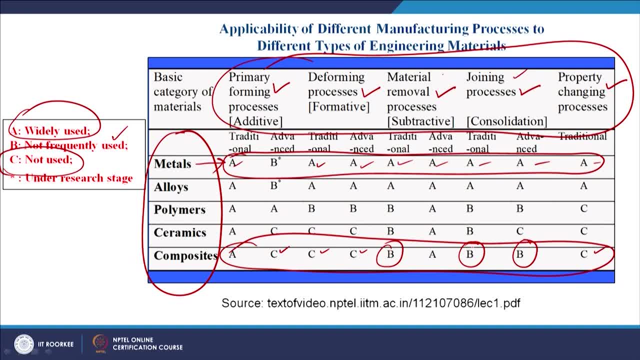 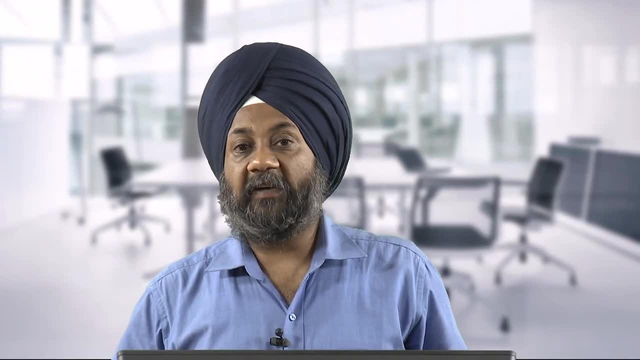 lot of research efforts are required. You need to develop new, better processes so that these Bs are also converted into As, that is, they are also widely used, and these Cs can also be converted into A, that is, these processes are widely used for manufacturing of composite materials also. 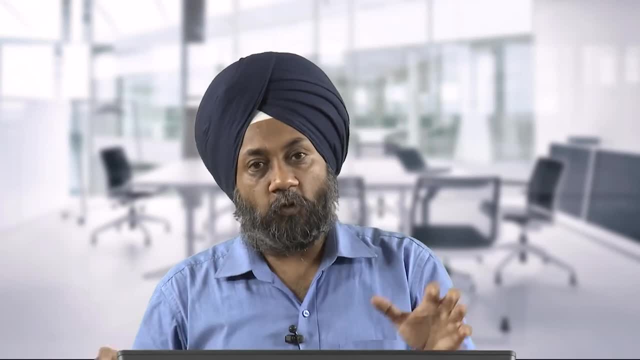 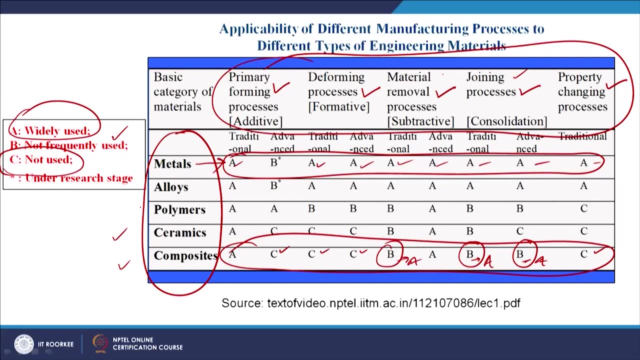 So this is quite clear from here, that for metals, most of the processes are very well established, and for other types of materials like composites And ceramics, as well as for polymers, we need to fine tune or we need to develop an understanding about the manufacturing processes. 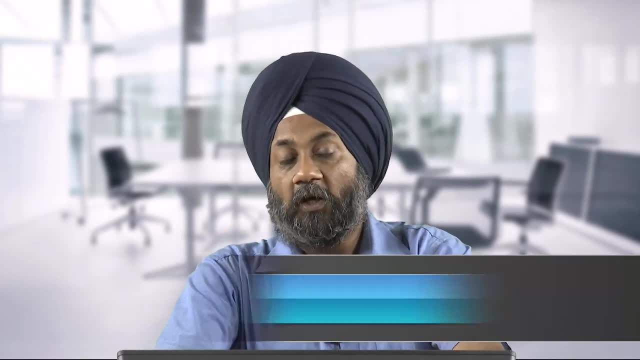 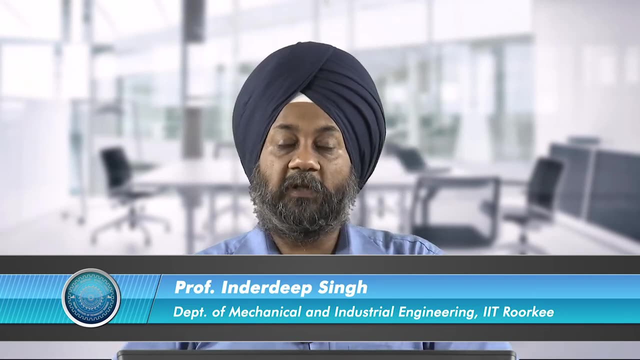 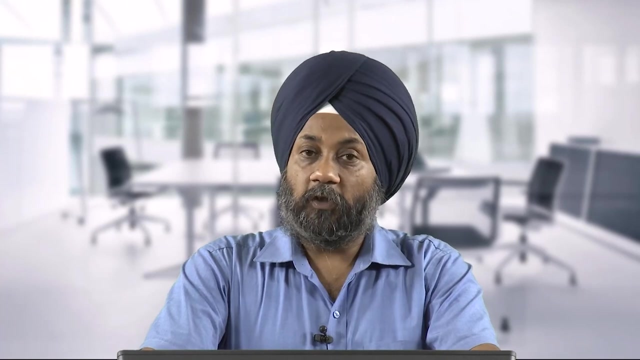 So that these materials can also find application all around us. So for plastics, if you see, these days lot of products are being made using the polymers or the plastic. It means the manufacturing processes are now well developed for manufacturing of polymers or plastics. 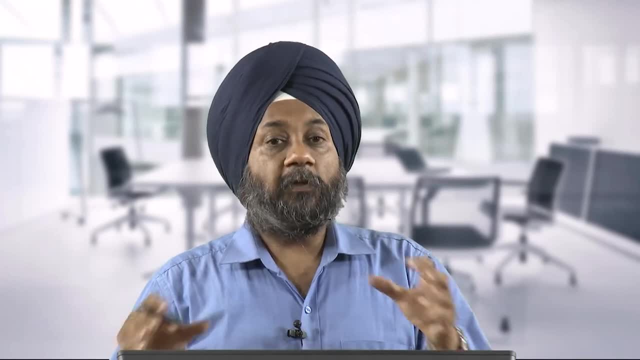 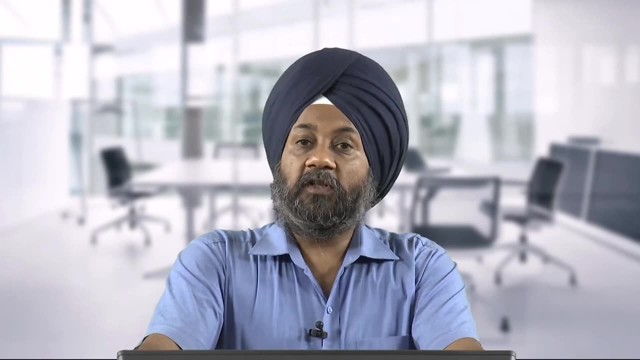 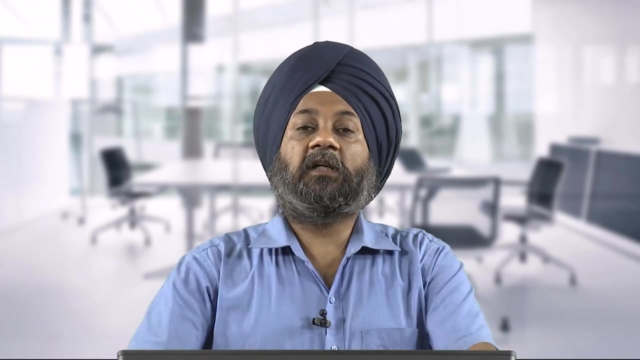 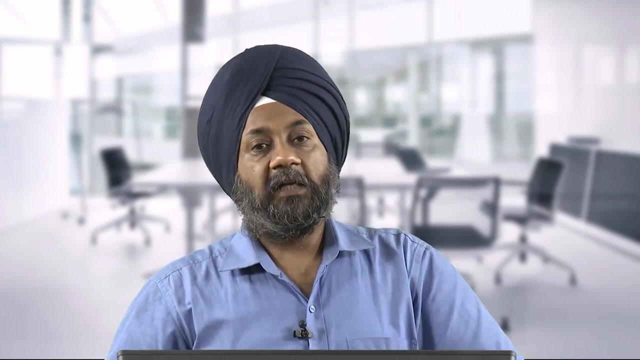 Processing of polymers of plastics and therefore the importance of this course is further, maybe substantiated. why? because when plastics are being used in such a big way, we must know that what are the manufacturing guidelines or the processing guidelines that we must follow when we are designing a product that has to be made in a plastic material. 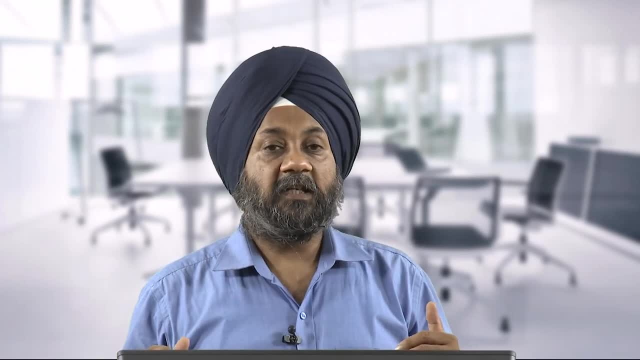 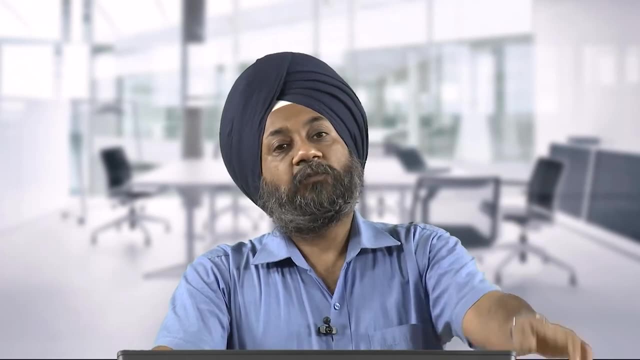 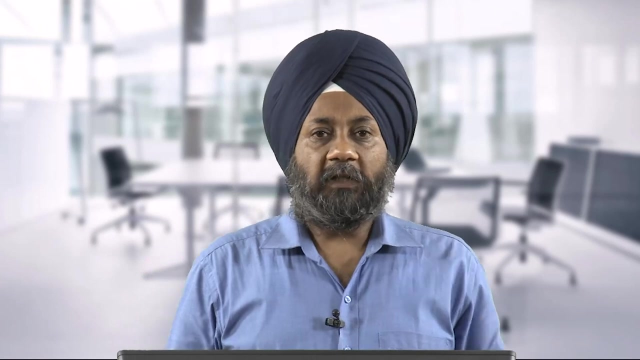 So that, therefore, we need to hone our skills. Okay, So we need to hone our skills to make our skills relevant from the product design point of view by focusing on the manufacturing guidelines. Sometimes we may propose a very good design, but we do not know that how this product is. 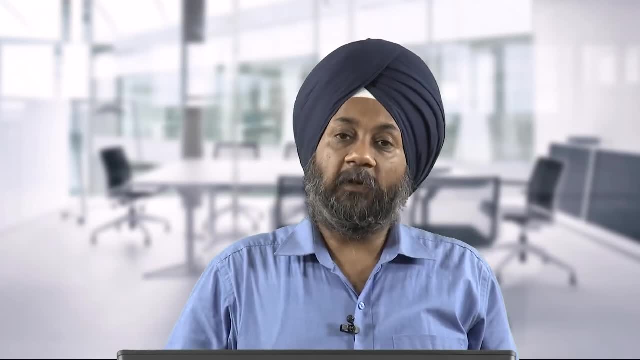 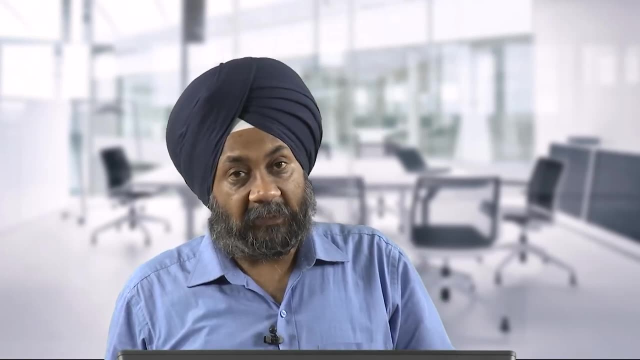 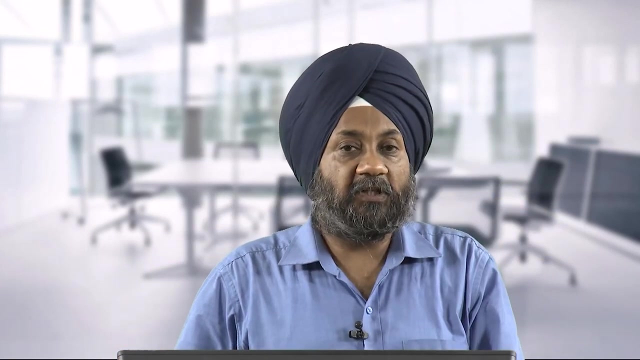 going to be manufactured. In that case, what is going to happen? the product design or it may look very good, but it cannot be manufactured. So if we have idea that X process or Y process or Z process, Okay, Z process, which is used for processing of plastics, can process this type of shape, can. 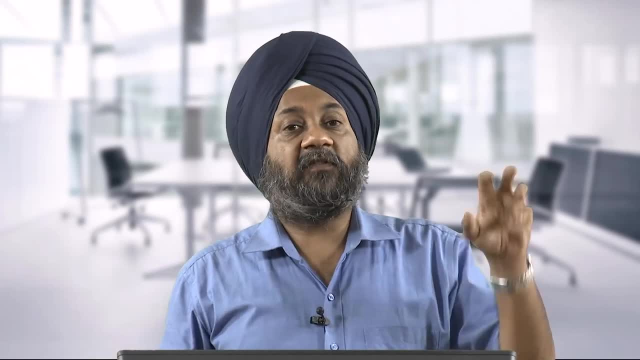 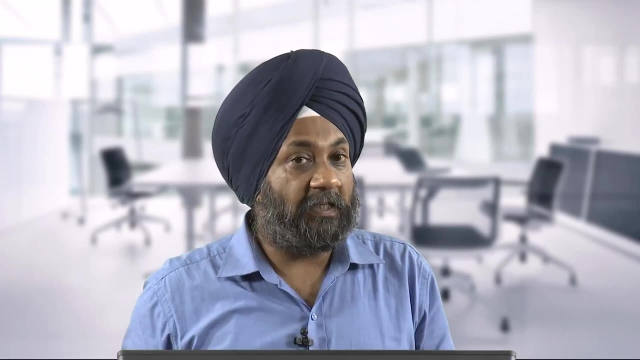 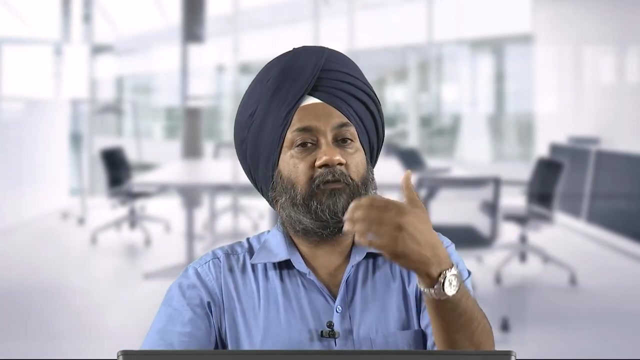 process this type of a design very easily. we will choose the process, We will modify our design, we will tweak our design, we will fine tune our design, keeping in mind the guidelines that we know for a specific process And therefore the iterative thing that, once we have finalized, we are not able to manufacture. 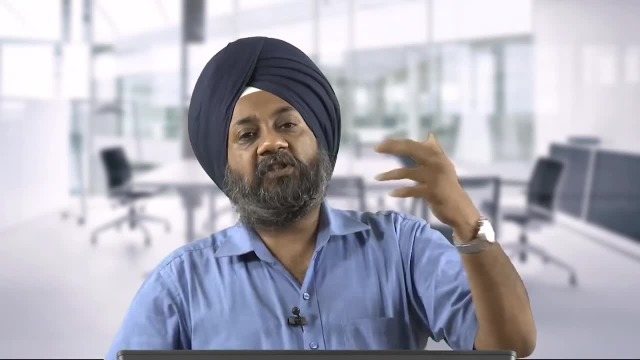 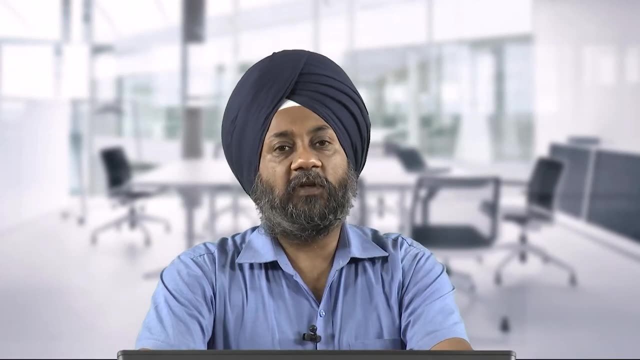 it. We are not even able to prototype it again. we change the design, we make some modification, again we are not able to prototype it, So then these problems will be there. So these type of problems can easily be overcome if we follow the manufacturing guidelines. 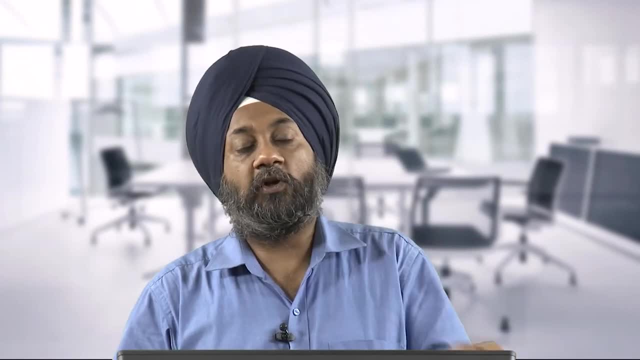 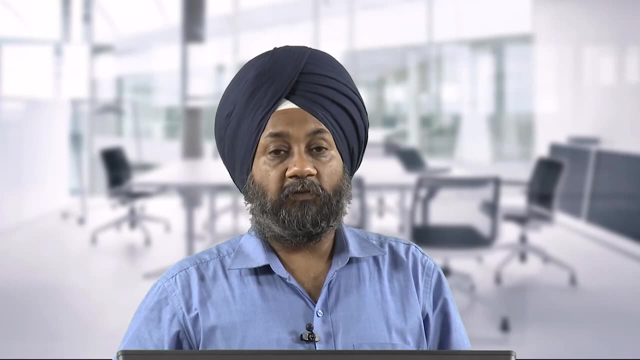 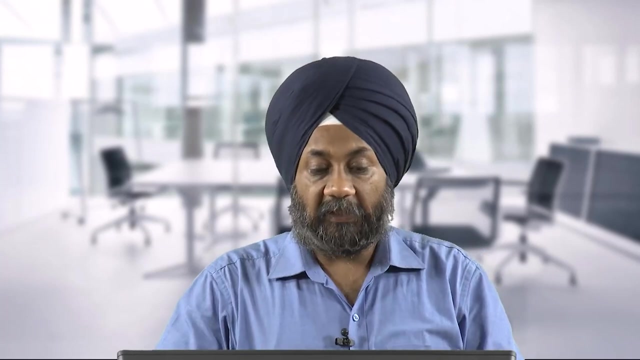 for the specific process by which the product is going to be converted into a final form or into a fully commercial product. So these are some of the, we can say- summary of the manufacturing process, Okay, Of the manufacturing processes vis-a-vis the engineering materials. that for which type? 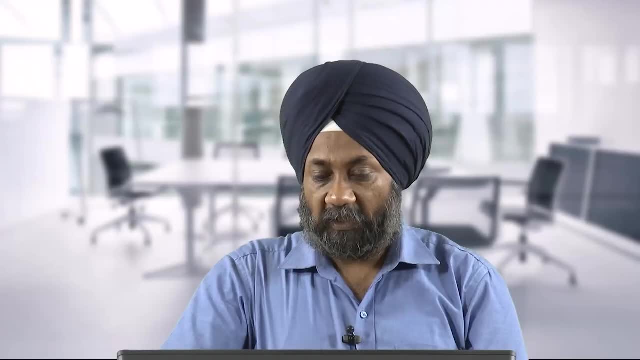 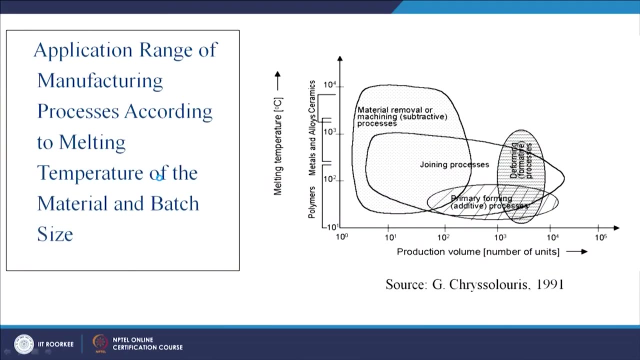 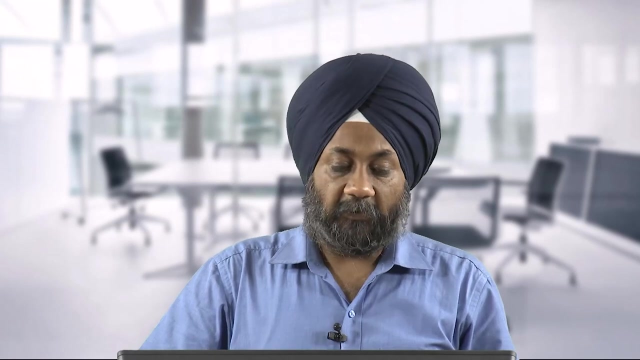 of material, which type of process is well developed? This is another- we can say- guideline or another criteria which can help us to decide that which process can be used under certain circumstances or under certain specific circumstances. So this is based on 2 important parameters. 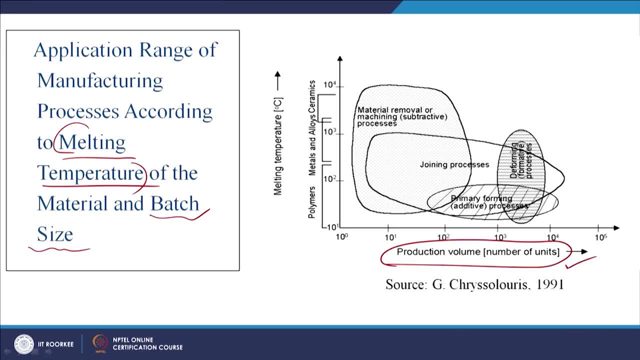 First one is the melting temperature And the another one is the melting temperature. Okay, The other one is the production volume, or the number of products that have to be produced, which can also be called as the batch size. So on y axis we have the melting temperature. on x axis we have the production volume. 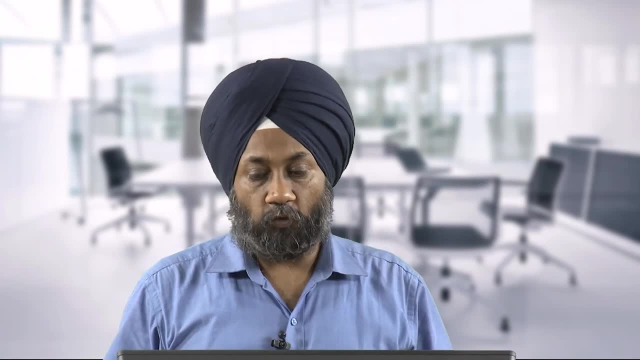 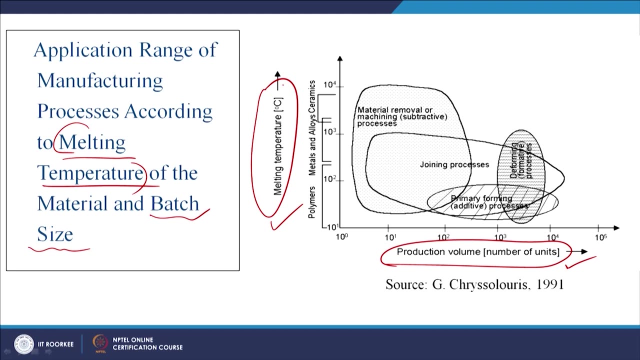 So when, once we have to select a manufacturing process, we must focus on these 2 parameters So we can see if the melting temperature is very, very high. So we cannot use a casting process, because in casting we need to melt the metal. So we can see here. 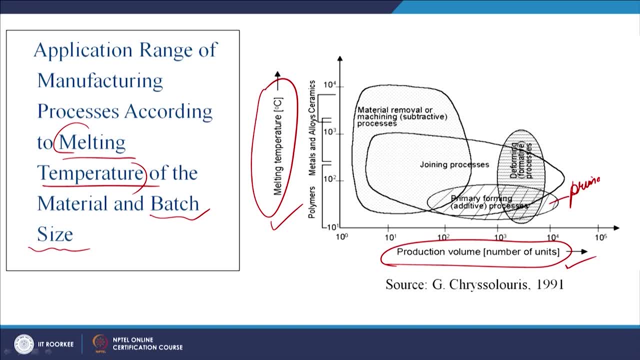 This is our primary forming processes. We can see it is written here: primary forming. So casting falls here. So it can only be used up to a melting temperature of a specific range only. So in that case, if the melting temperature of the material is less, we can use the primary. 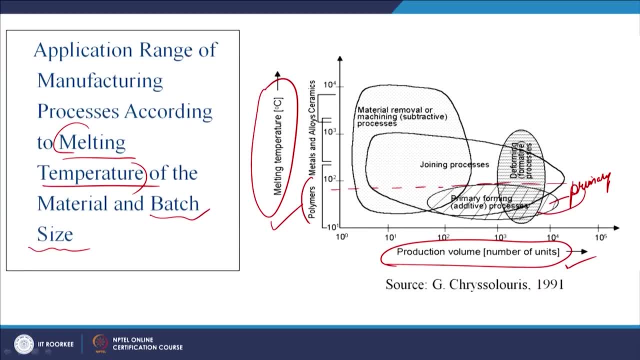 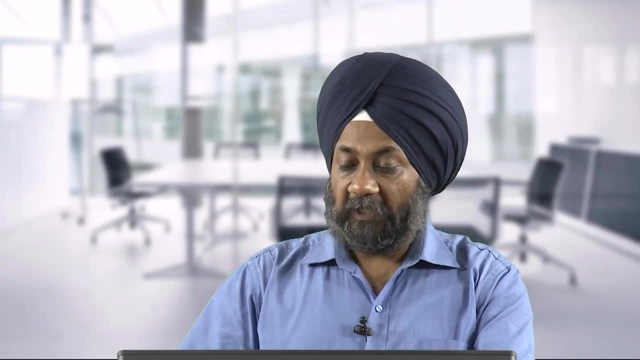 forming processes And from materials point of view you can see. for polymers we do not have too high melting points And therefore the primary forming processes, such as injection molding, compression molding, these can easily be used for processing of polymers. Then we can see if the ceramics have very high melting point. 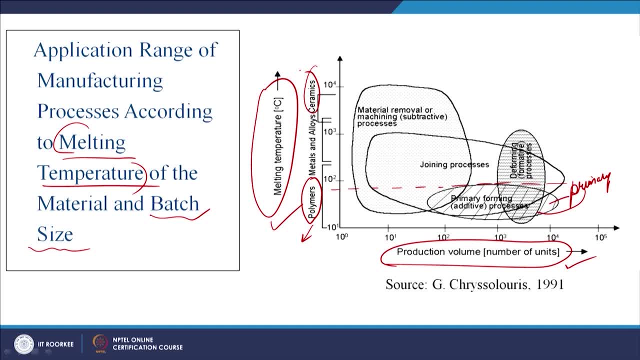 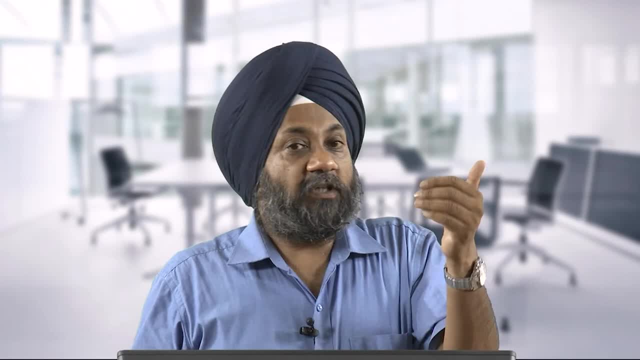 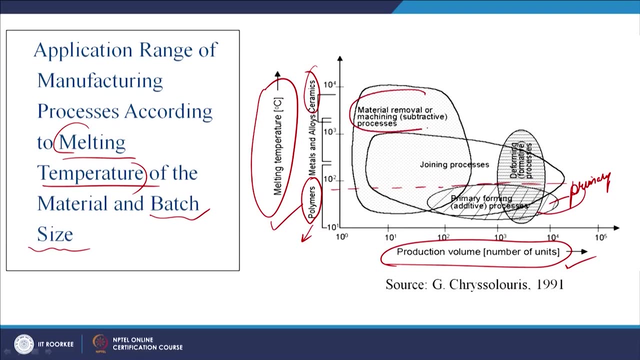 So for them, it is difficult to form them using primary forming processes because we cannot melt them easily. So we need to look for certain other processes which can be used, and similarly for metals. if you see, If the temperature is very high, we can go for material removal processes. 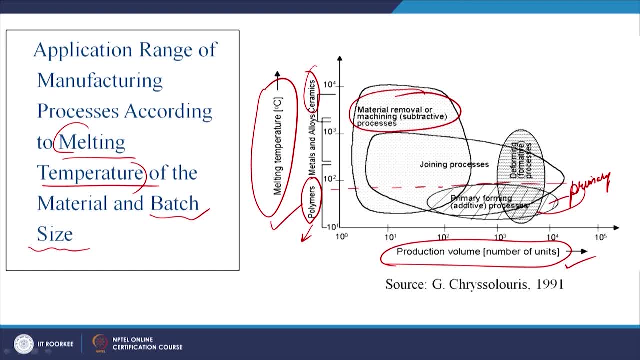 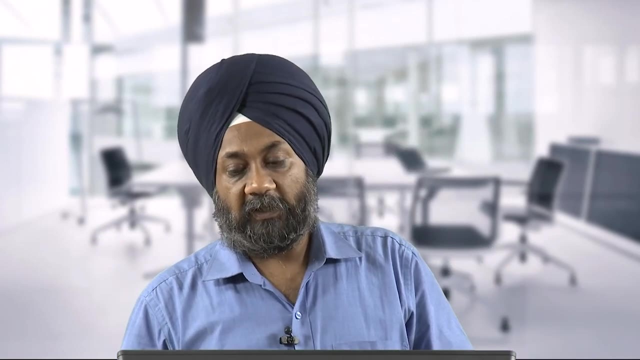 We can machine the part into a given shape. Similarly, if the production volume is very large, we can go for deformative processes. It is written here deformative processes. it is already written here. So if the production volume or base size is large, then only we must go for the deformative. 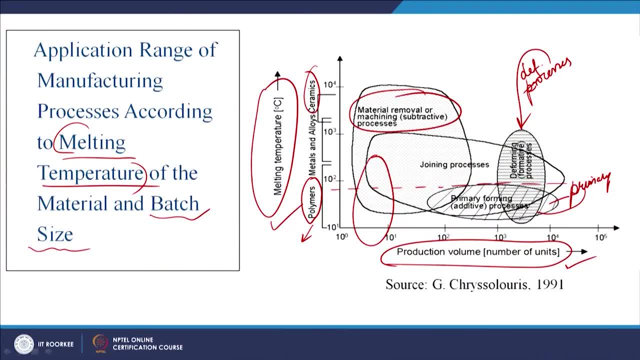 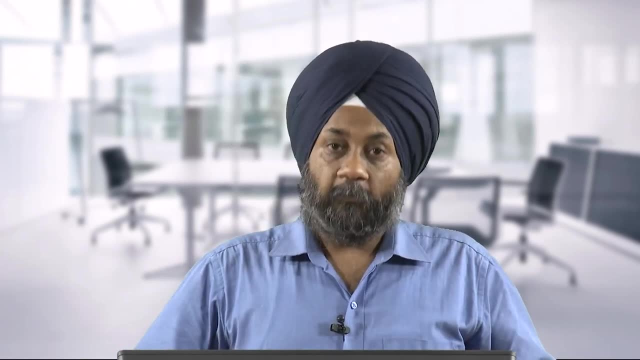 processes If the production volume is small. somewhere here we must not go for deformative processes, because the cost of the die, the cost of the equipment, the cost of the machines may not be justified if we have to deform only a small batch size or only a small quantity of products. 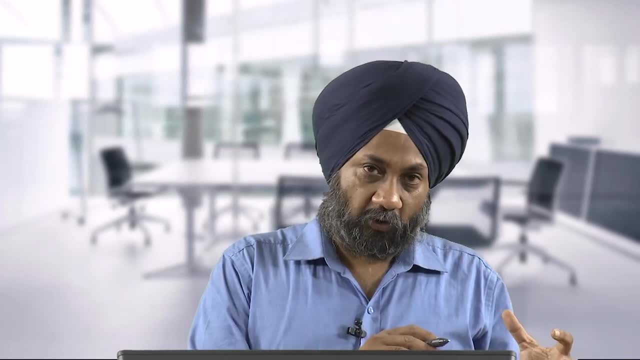 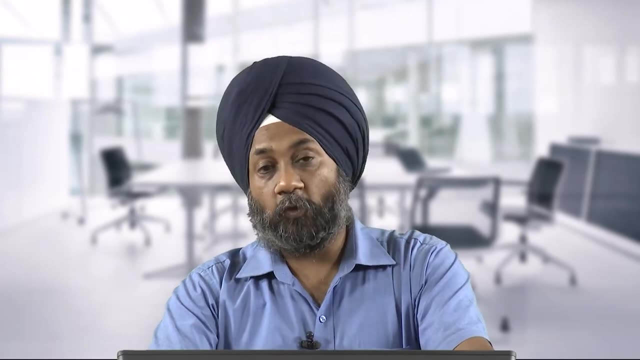 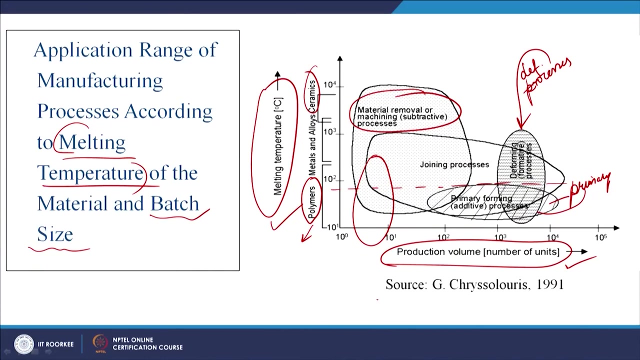 So, based on the production volume, based on the melting temperature of the materials, based upon the type of materials that are going to be used for the product design, we can appropriately, judiciously, select a manufacturing process. So here, this diagram has been taken from this book, the source is given and, if you can follow, 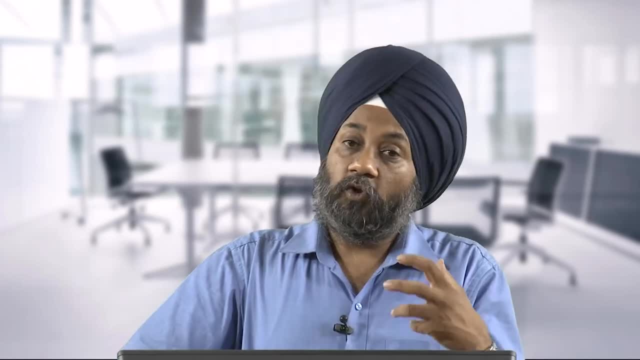 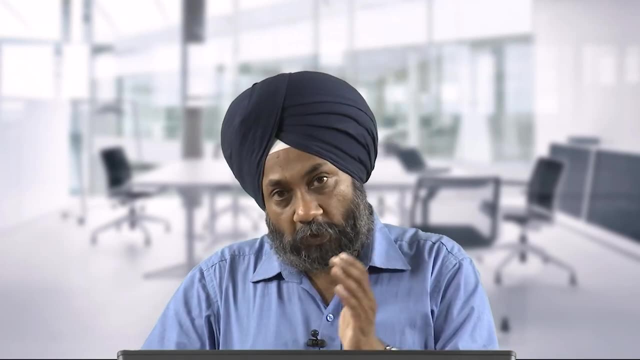 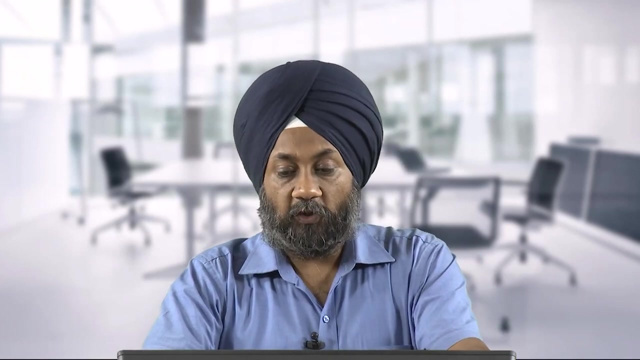 this book. from specifically this important diagram, you can get the further insights into the selection of the manufacturing process depending upon these 2 important criteria of melting temperature as well as the production volume, So you can see for yourself which processes are used. So this diagram has been taken from this book. 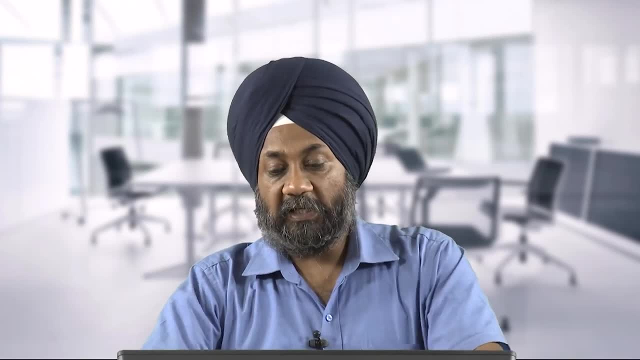 The source is given and, if you can follow this book from specifically this important diagram, which processes are used for the production volume of the materials. So these are the 3 criteria I have already taken: The primary forming, where the melting temperature is less. 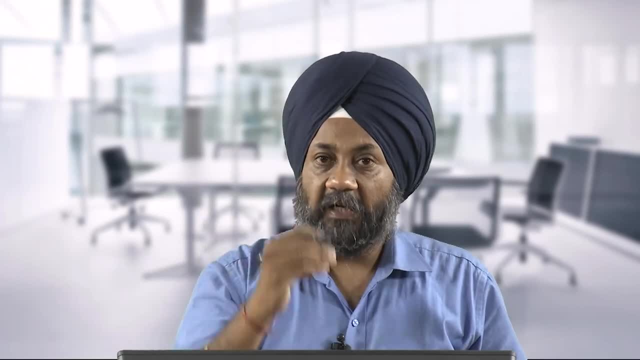 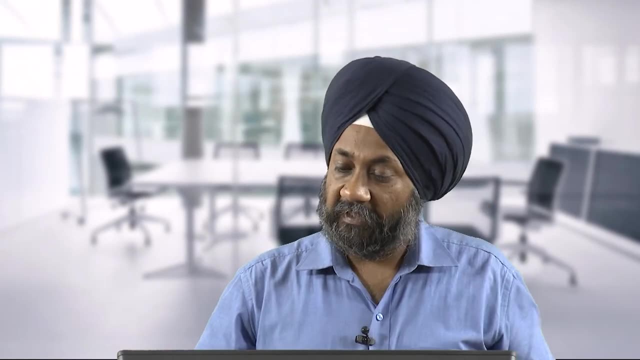 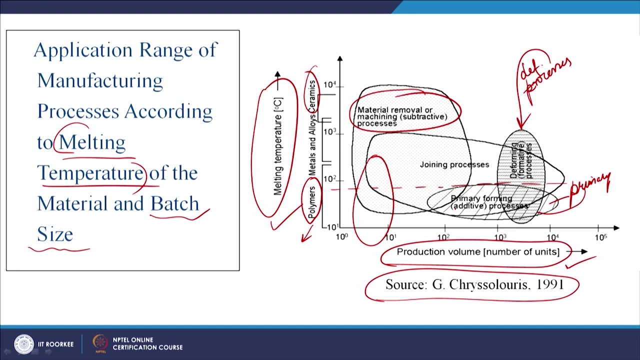 Material removal processes where the melting temperature of the material is high as well as the production volume is low. Similarly, the primary forming process is where the melting temperature is less. Deformative processes where we have a large quantity or the batch size is very, very large. 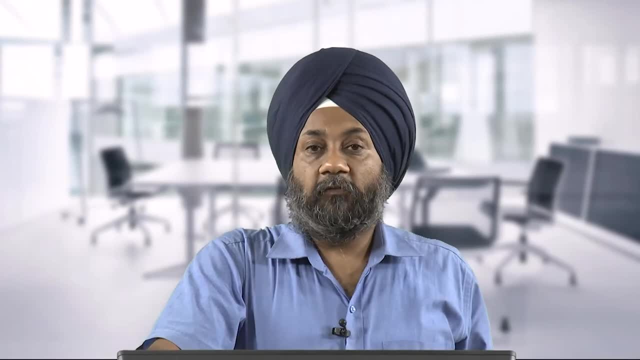 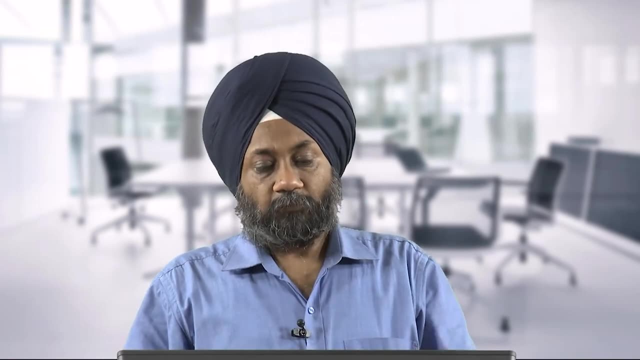 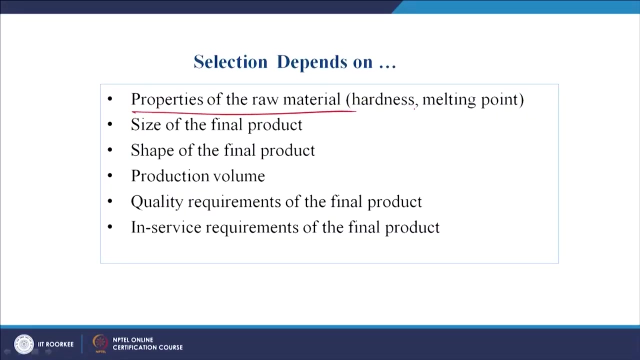 So these guidelines are handy tools for us in order to decide that which process we must use for which particular application. Now the selection depends upon- we can see the properties of the raw material. if you see in the previous slide we can see different types of raw materials are there. we can have 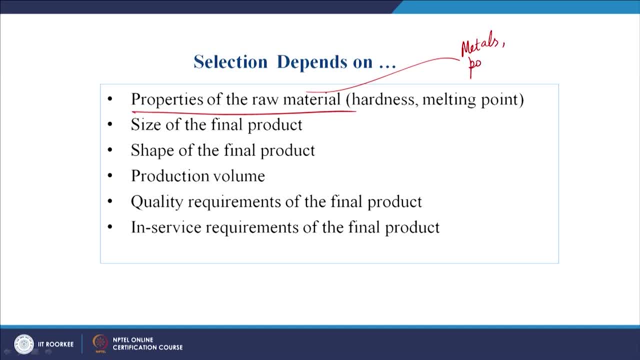 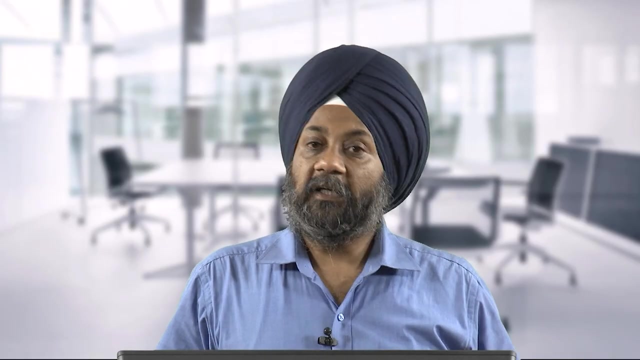 metals. we have taken an example of polymers. we have taken an example of ceramics. So different types of materials will ask for different types of manufacturing processes. so for ceramics there will be different processes. for metals there will be different processes. for polymers, there will be different processes. 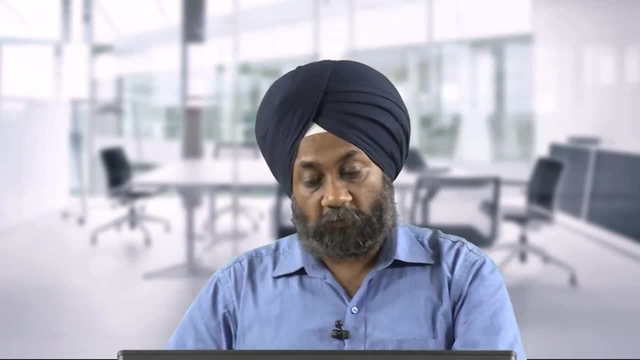 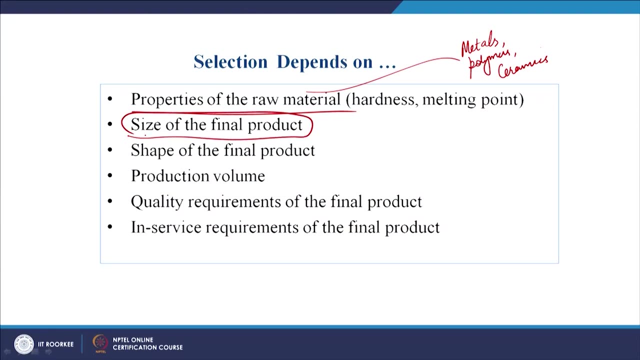 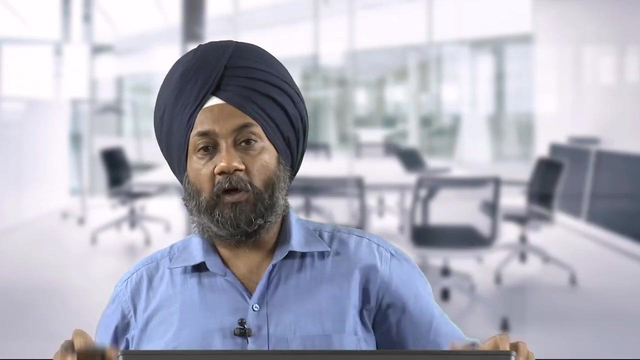 So the selection of the process will depend upon the properties of the raw material for the size of the final product very, very important. If it is a small product, a different manufacturing process will give you economic production. if it is a very large size product, a specific manufacturing process will give you a desired 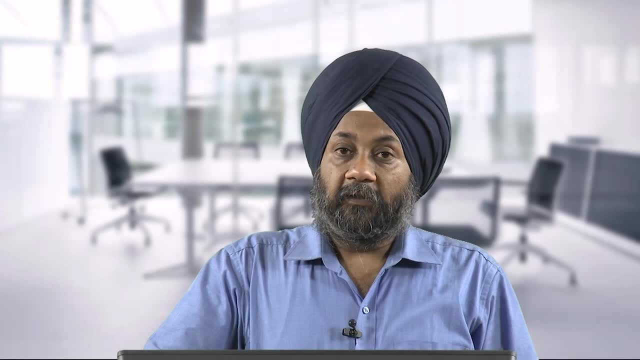 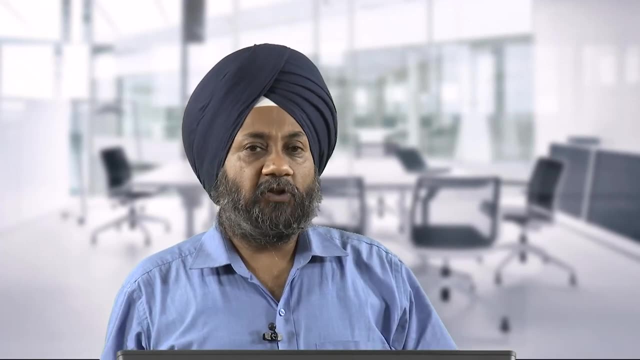 output. So we can see simple thumb rule: if the size is very, very, very, very big, you will not be able to make it by machining process Because you have to hold the job on the machine and then only you have to machine it. but 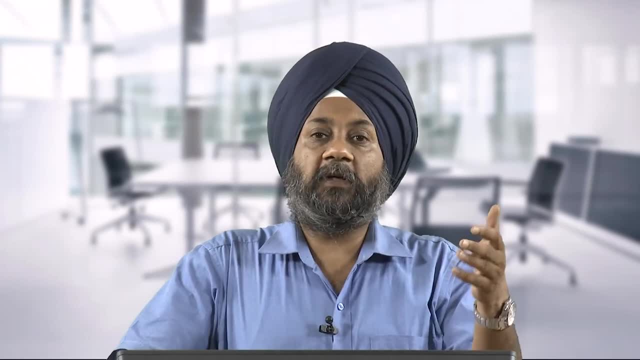 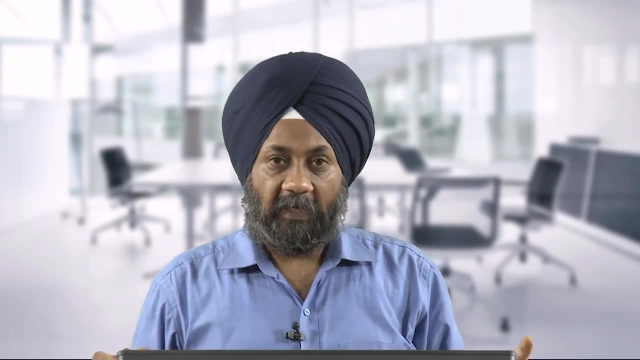 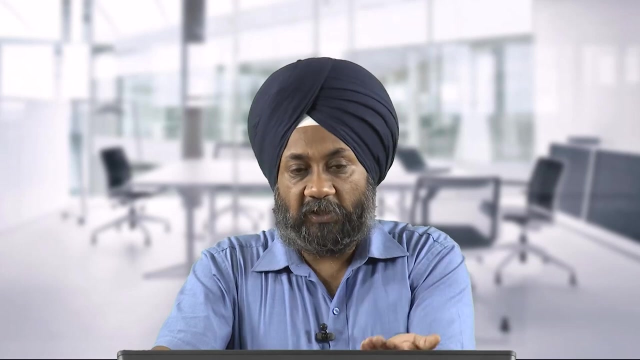 you can easily make it by the casting process. So simple, maybe. rule of thumb. that is, the size of the product is very, very large and it has to be made by metal as the raw material. it is always advisable to follow the casting process. Simple rule, simple guideline. it is written nowhere, but as my own experience of maybe 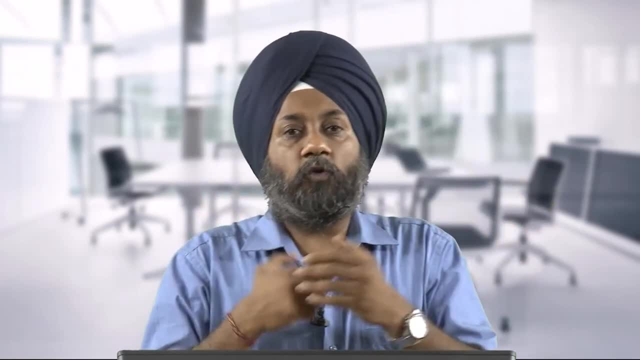 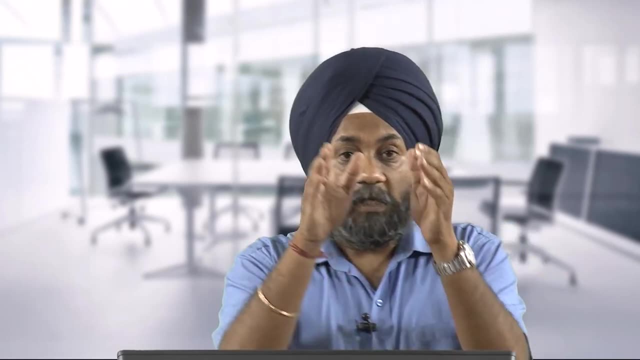 dealing with this type of courses for so many years, it has just come to my mind. So: large size product, mostly you will go for casting. there may be certain exceptions and if you see the syllabus for this course, we have already highlighted the exceptions. the 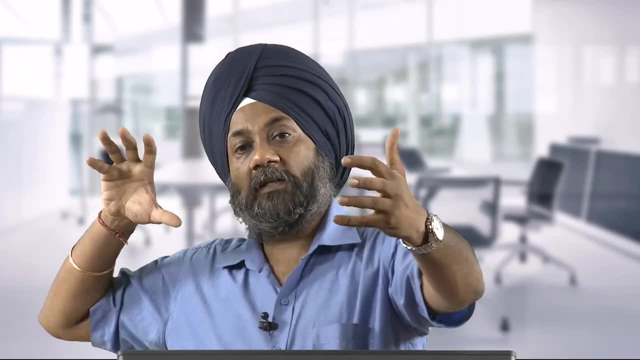 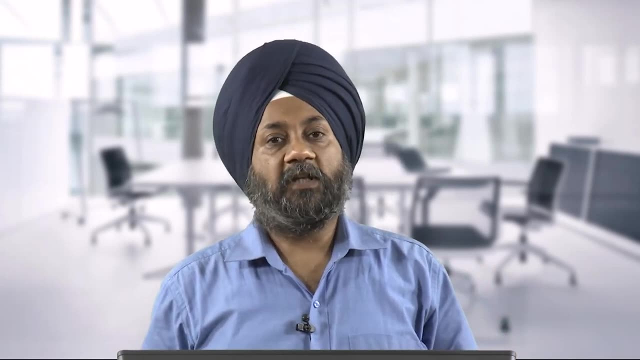 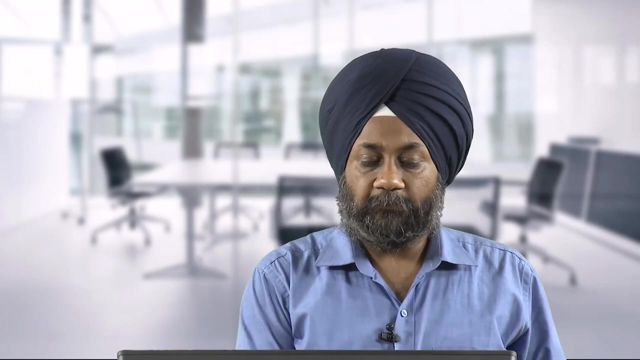 applications. So maybe there may be exception, that there is a large size product, but it can only be made by machining process. But in general, if the size of the product will be large, it will be made by the casting process. So the size of the product is important, the shape of the final product is important. 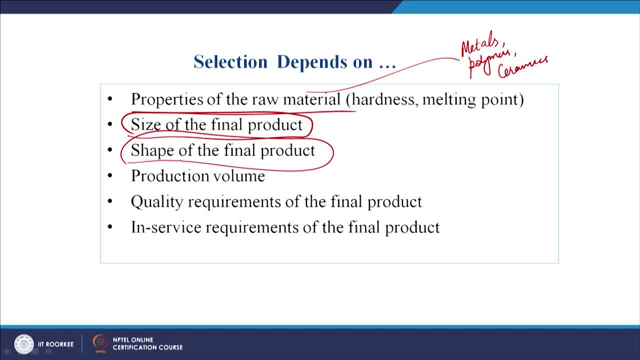 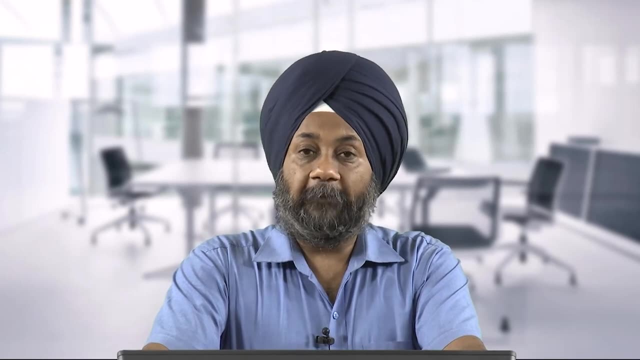 If it is very, very intricate, very, very complex geometry you have to make, it will certainly affect your choice of the manufacturing process, Sometimes your process with that you are using for making a product like this, that can be, we can say, very, very easy to make a product with this shape, not very complicated. 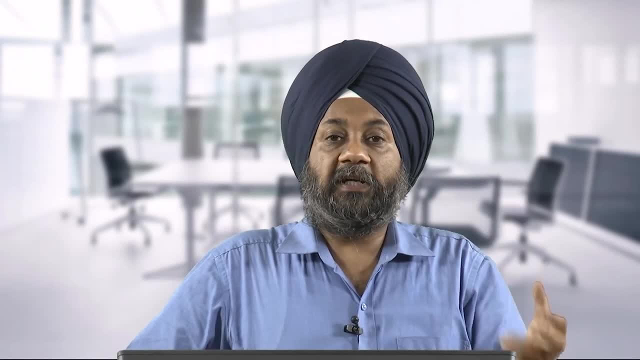 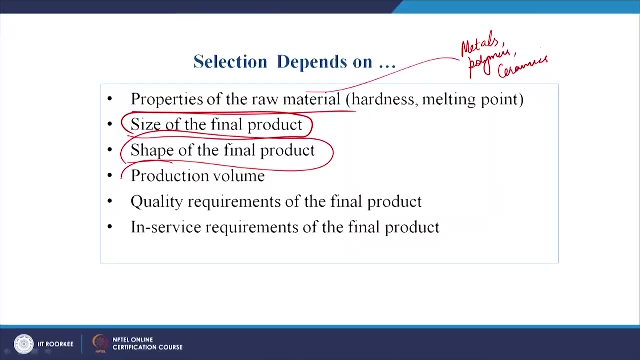 But, on the contrary, you may have a other, fairly Fairly complicated products which may not be made by a process which you can use for making this product. Similarly, in the previous slide we have seen production volume, the number of products that we are going to produce. 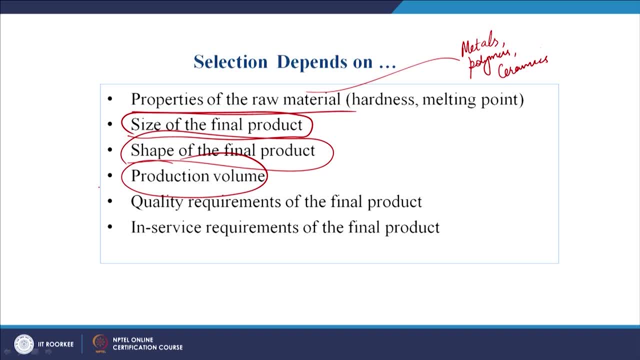 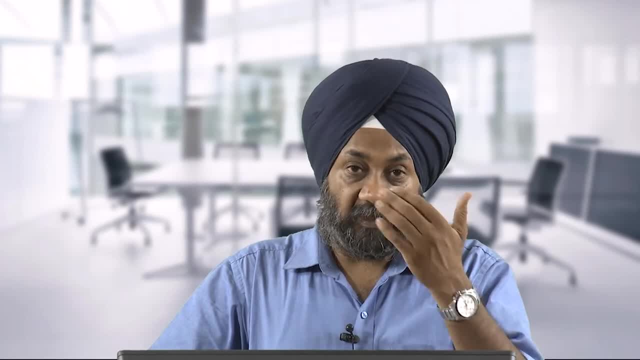 In the previous slide. you can refer back. you can see the number of products or batch size is large. deformative processes are advisable quality requirements of the final product. we will see with examples and case studies that if you do not use a particular process or a specific process, 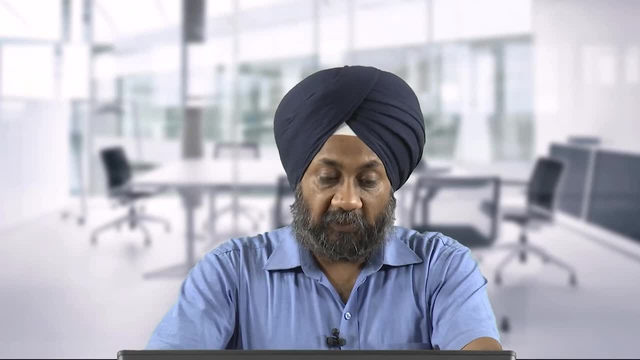 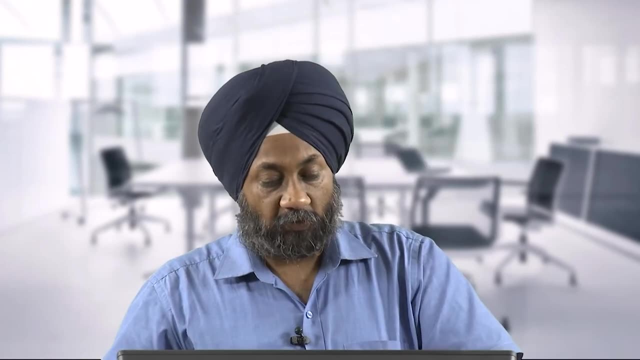 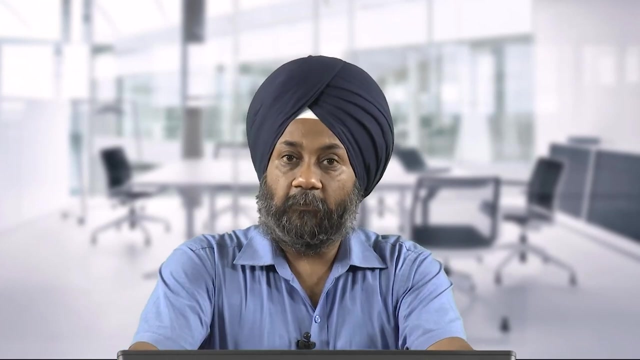 The quality of the product will not be as desired, So it will certainly affect our choice of the manufacturing process, or our selection of the manufacturing process, as well as in service requirements of the final product. sometimes also will help us. One example that is coming to my mind is of self lubricating bearings. 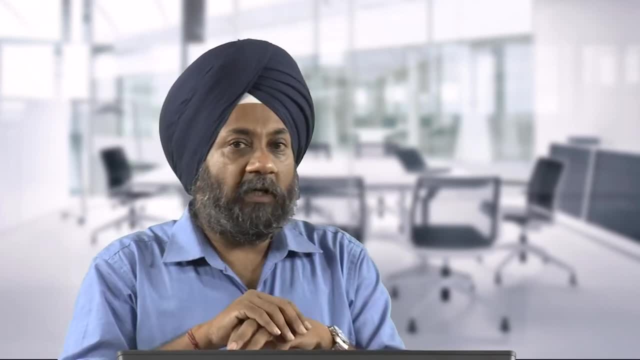 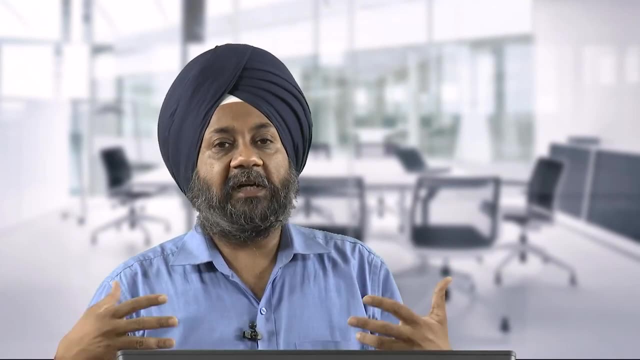 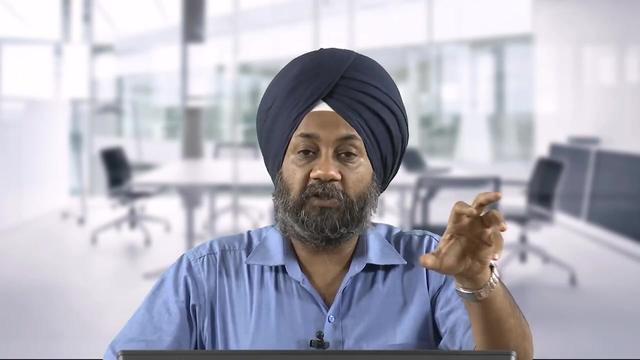 Now in self lubricating bearings. you must impregnate the oil during the manufacturing process itself So that when you put it in service It automatically lubricates the moving element. So during the manufacturing process only we have to select the manufacturing process in such a way that you manufacture the self lubricating bearing. 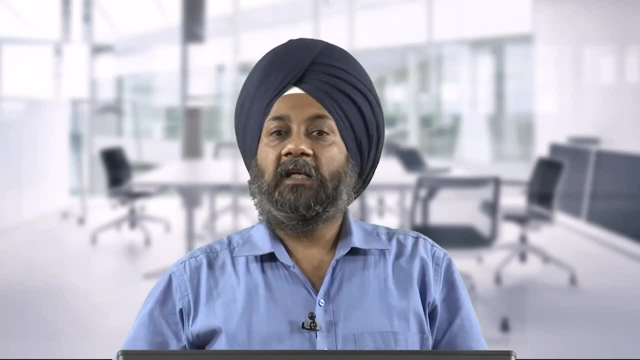 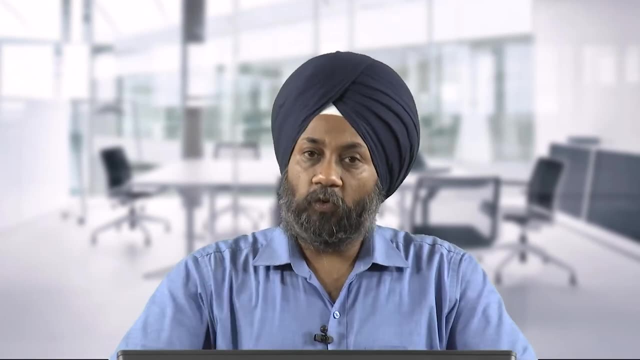 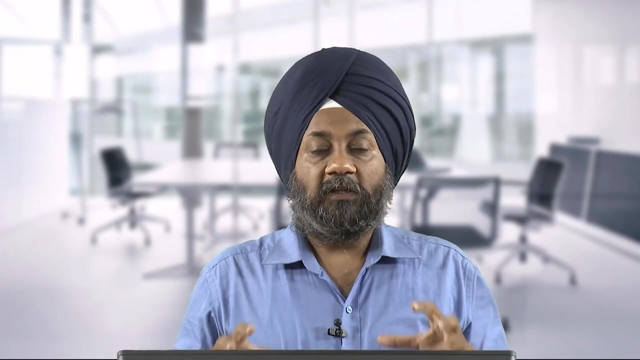 So that in service, when it is used, it is performing its intended function as per the design requirement. So with this we conclude the today's session. I think the session was more in general discussion And we have tried to see that how the processes can be classified.